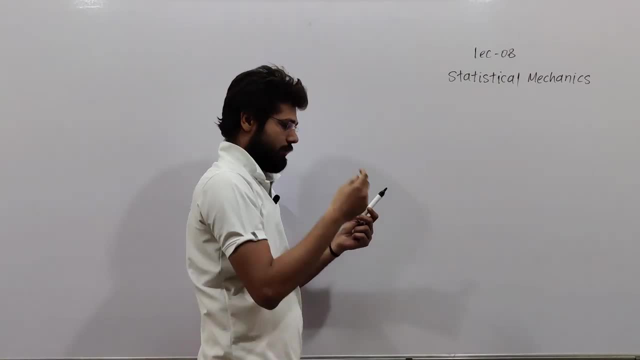 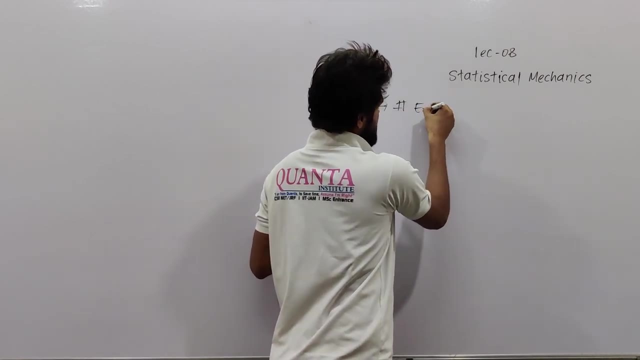 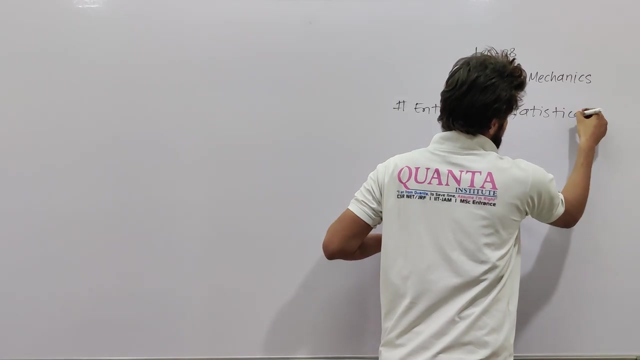 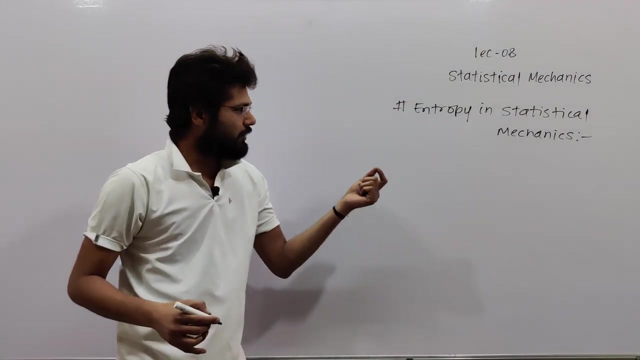 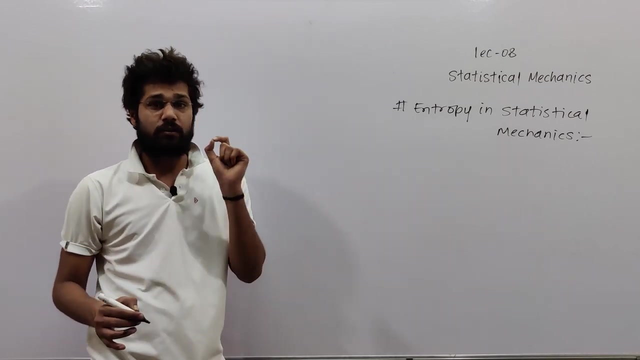 mechanics. Okay, So right. Entropy in statistical mechanics: The relation of entropy, the format in which it is written. that relation is also called etch theorem- Etch theorem- This relation is also called etch theorem, And this relation is also called 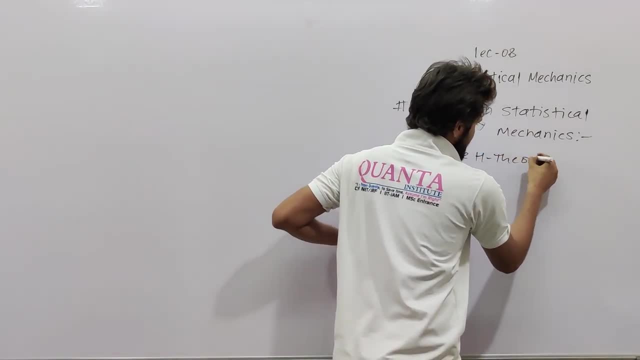 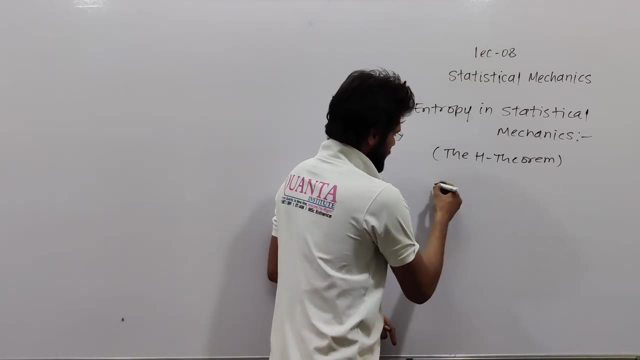 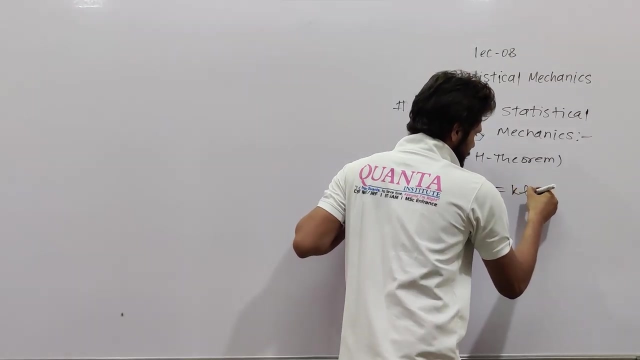 etch theorem, So you can also write the name of the topic: etch theorem in entropy or stats. he can also be called etch theorem. What happens? What happens in entropy? in this statics s equal to k, ln of omega. 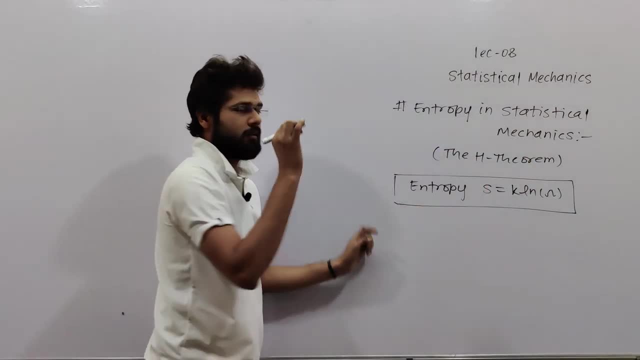 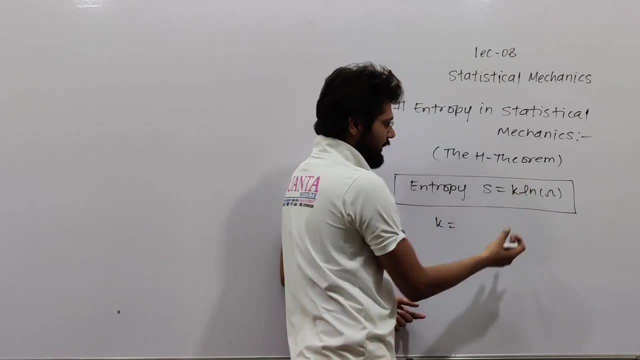 This is the entropy in the statistic, This is etch theorem. What is here? what is k? gaming? well, What is K? What is omega? What is S? S is entropy. Look at K and omega. K is Boltzmann constant. 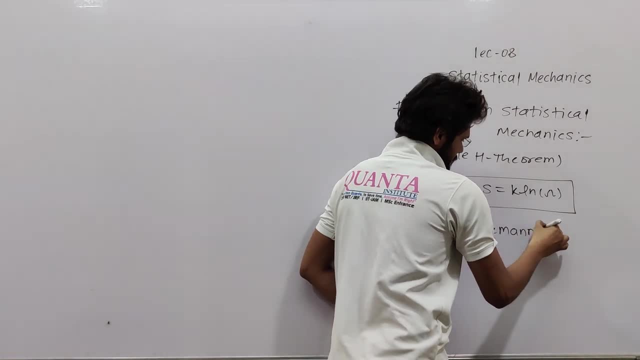 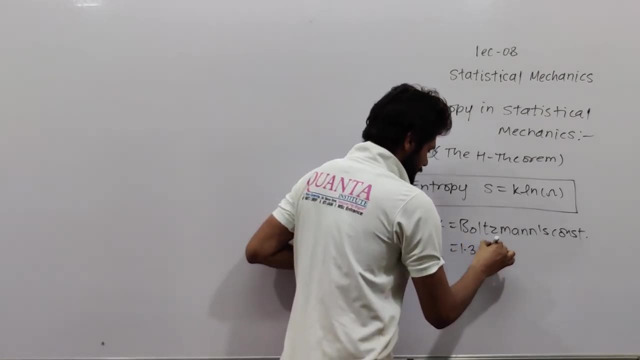 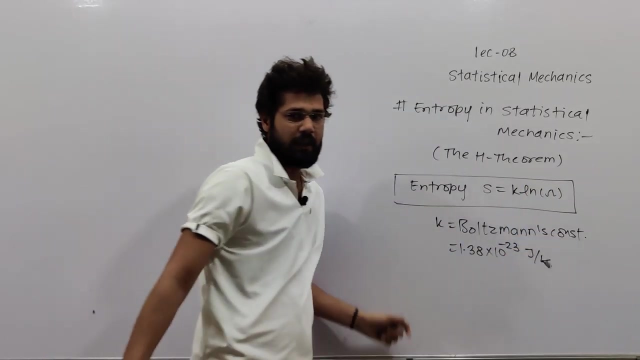 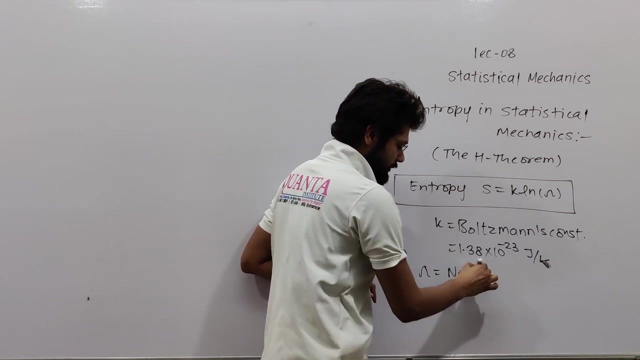 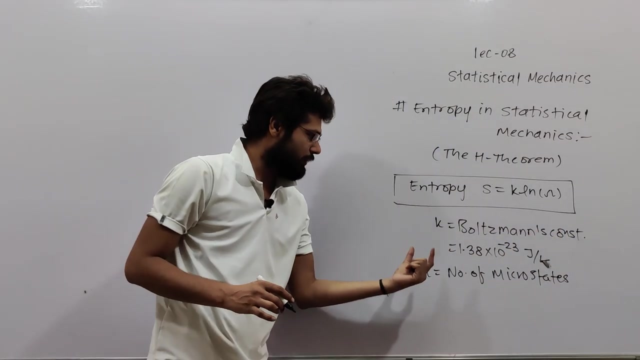 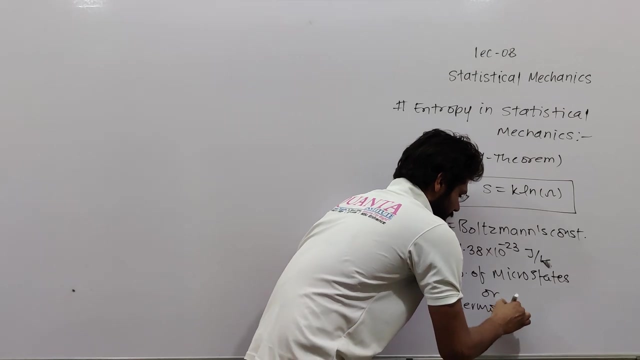 Boltzmann constant. Boltzmann constant is 1.38 into 10 to the power minus 23 joules per Kelvin. And what is omega here? Omega is number of microstates, And number of microstates is also called thermodynamical probability. 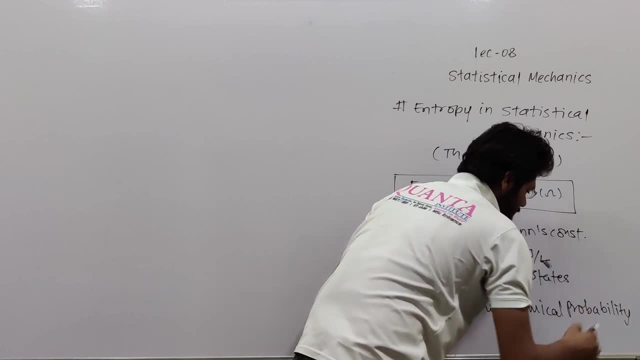 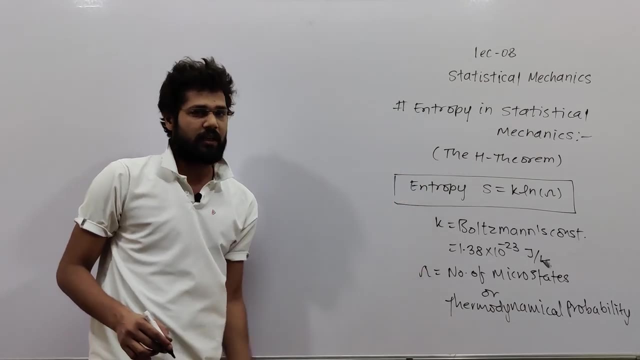 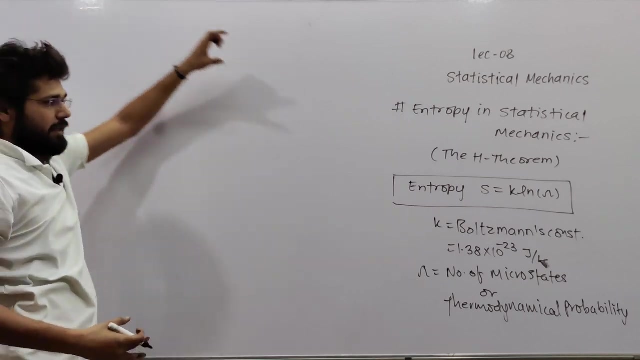 This was discussed yesterday in the lecture. Thermodynamical probability is called microstates. So this is the H-Thorum and this is the Entropian Statement. Now let's discuss this a little bit. See, what is this actually. 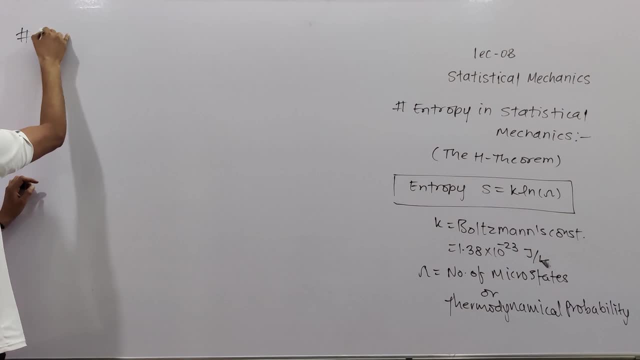 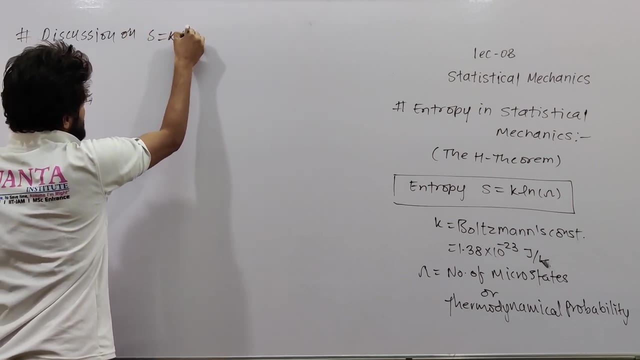 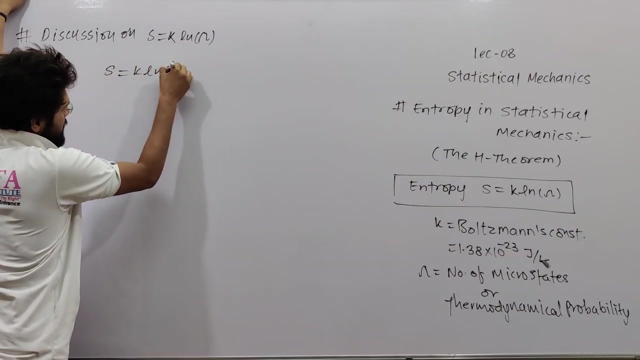 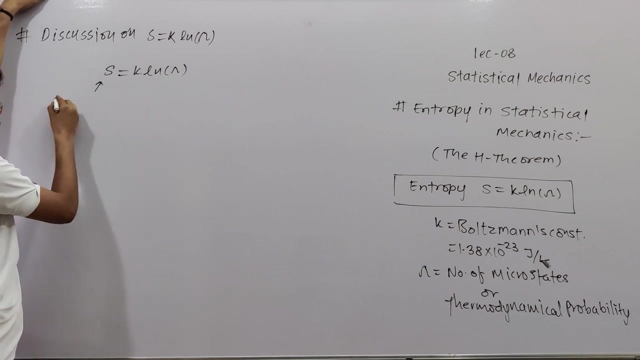 Next topic is Discussion on S equal to K, ln, omega. Discussion on H-Thorum. First of all, you have to discuss this relation, Okay, Okay. Now what is S here? Entropy? Entropy is a thermodynamical variable. 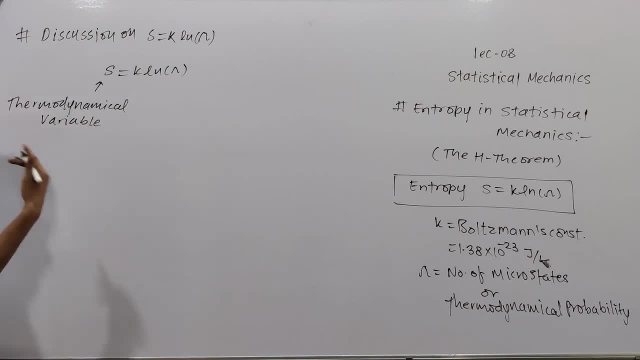 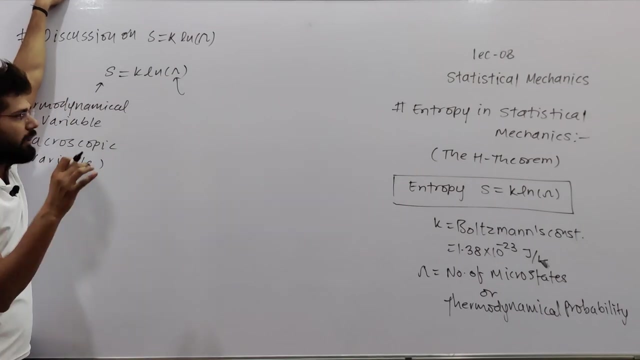 And I can say entropy is a macroscopic variable. Thermodynamic means macroscopic variable, Is it correct? Okay, And what is this omega? Number of microstates. Number of microstates is what? Microscopic property of system, A macroscopic parameter. 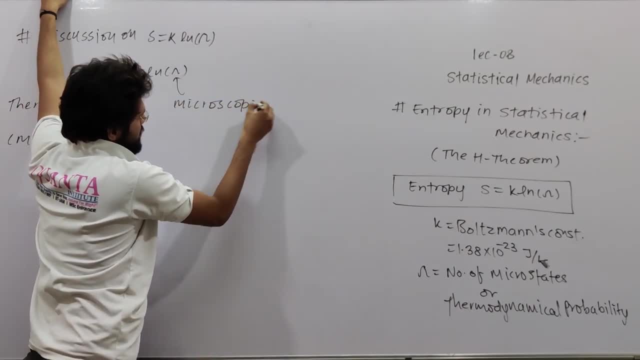 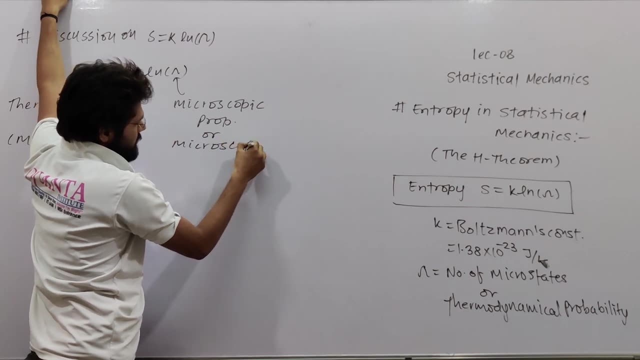 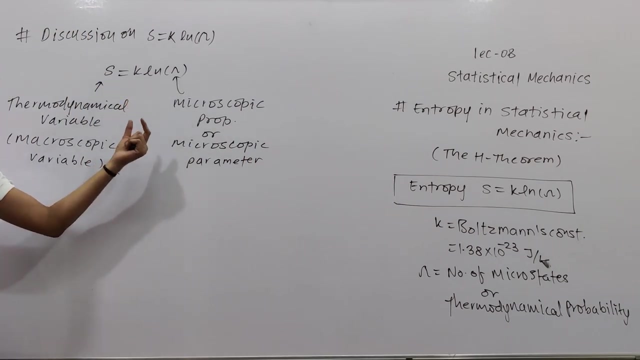 Microscopic property of system or macroscopic parameter of system. Microscopic parameter of system. Okay, Now notice one thing: If you know the omega, if you know about microstates, then you can obtain entropy. And I can also say that if you know the microscopic properties of the system, then you can obtain macroscopic variables. 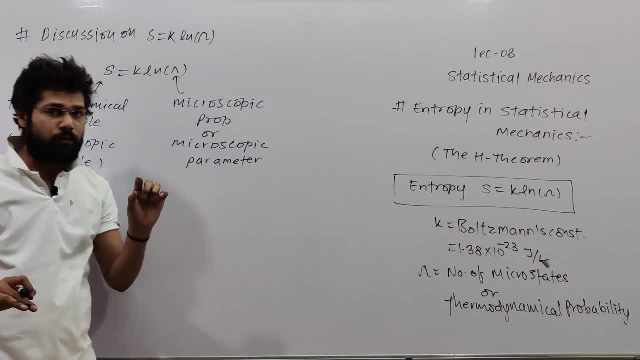 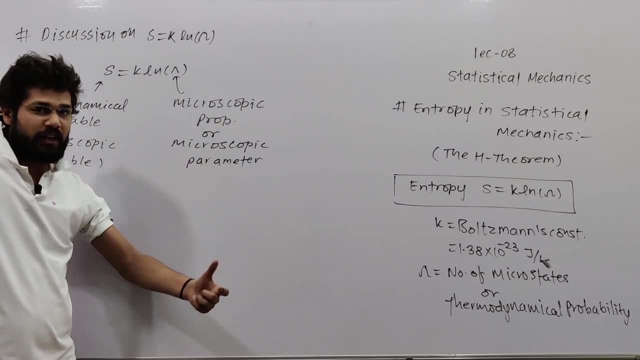 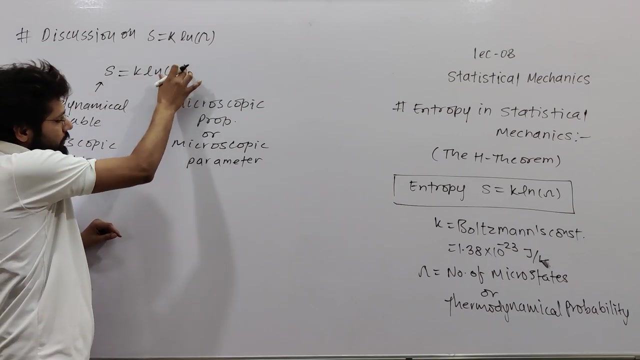 Okay, So what is this relation saying? This relation is a very strict relation. When the S-Thorum was developed, there was a Diwali celebration in the scientist community. Why did this happen? See? See, This is what. 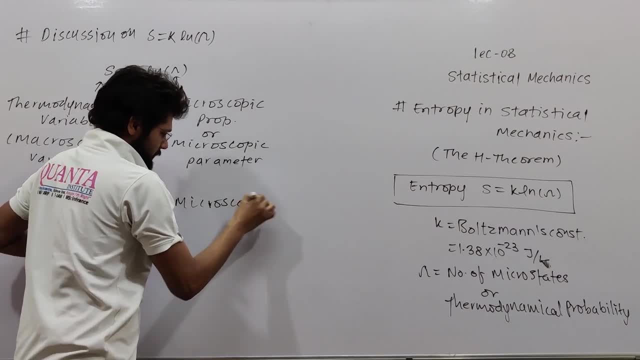 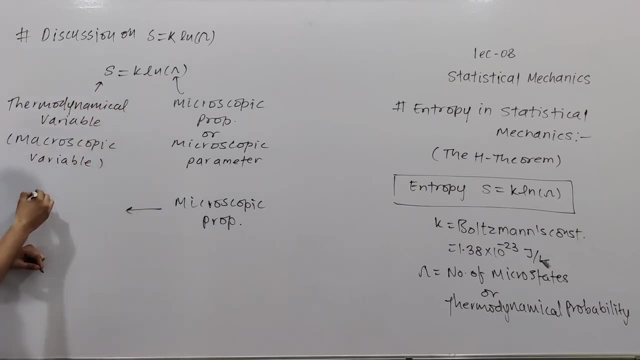 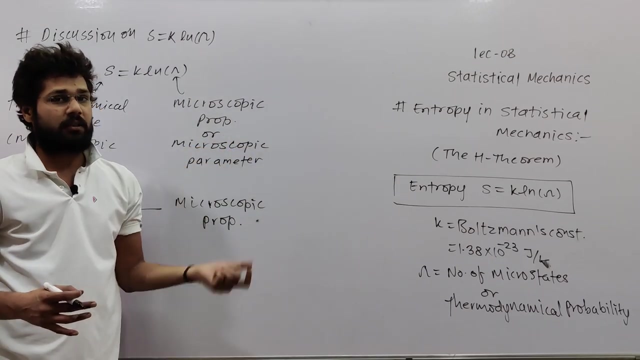 Microscopic property And by microscopic properties of system you are getting, you are obtaining macroscopic variables or macroscopic parameters. Actually, why was the STATMAC designed? Why was the STATMAC developed when there was thermodynamics? See, what did you do in the STATMAC. 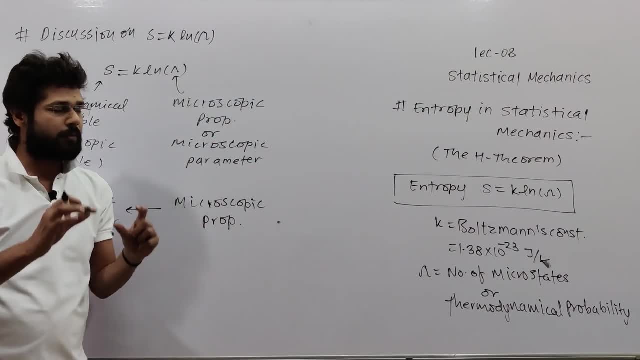 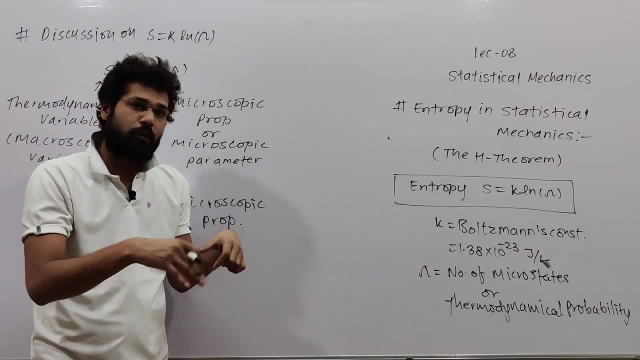 What did you do? Why did you develop? What was the thought? The thought was that you want to study the system at the micro level. And what did you want to obtain by studying at the micro level? That you get thermodynamic results from the microscopic study. 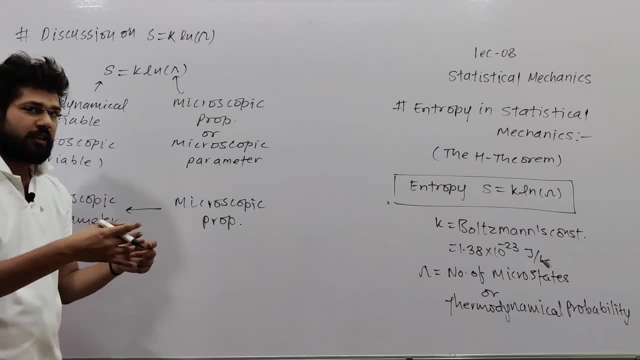 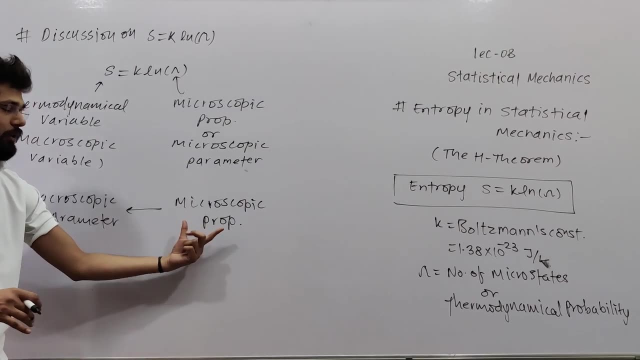 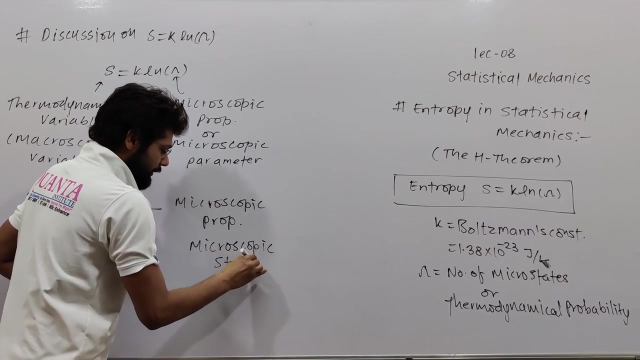 You obtained the results of the thermodynamic macroscopic study. So see what is this relation giving you. This is a type of microscopic study, And what is the microscopic study giving you? Thermodynamic results. You can see what are the macroscopic parameters. 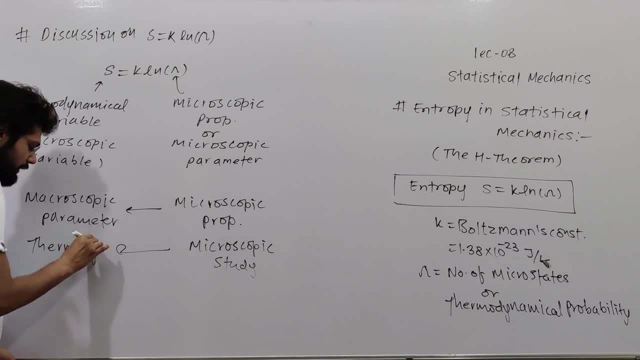 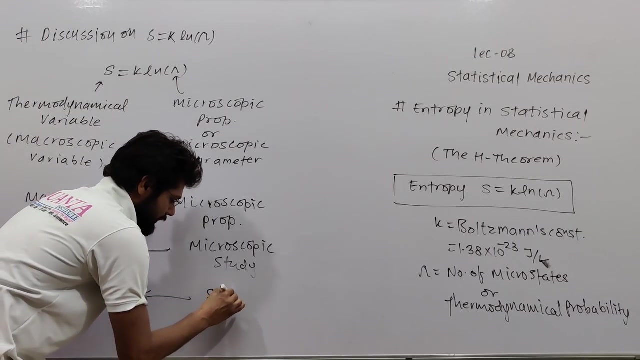 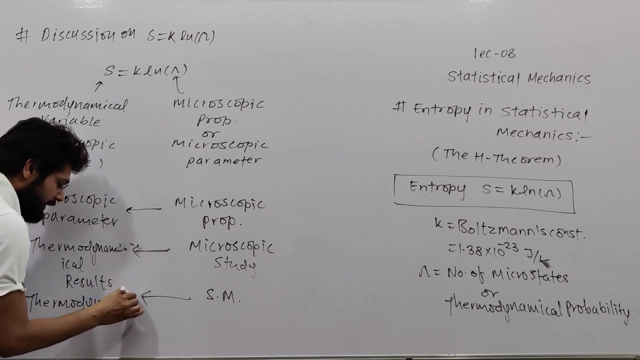 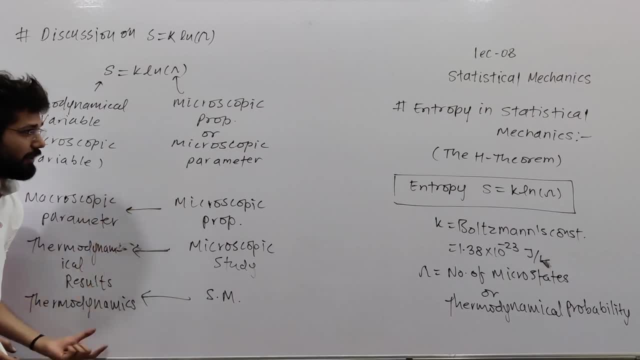 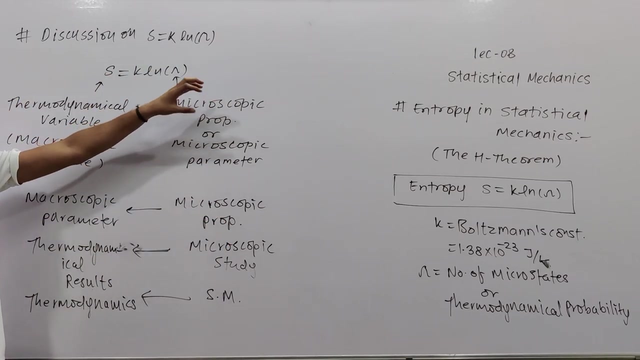 That you can obtain thermodynamics from microscopic study, And that's why this relation is so important. This relation is a trickle Means. it is very special When it was developed. it was a very special day Because you are obtaining thermodynamic variables from microscopic properties of the system. 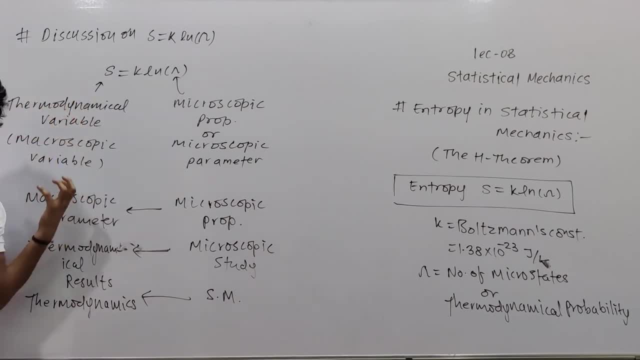 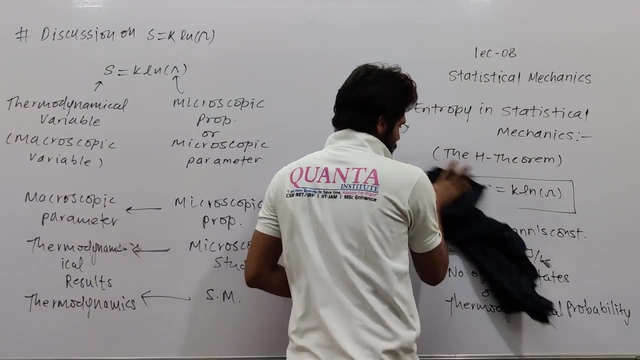 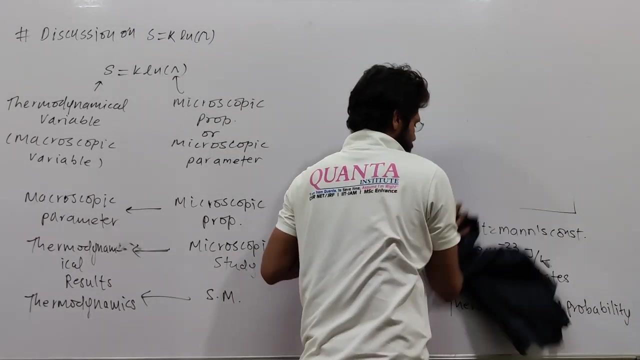 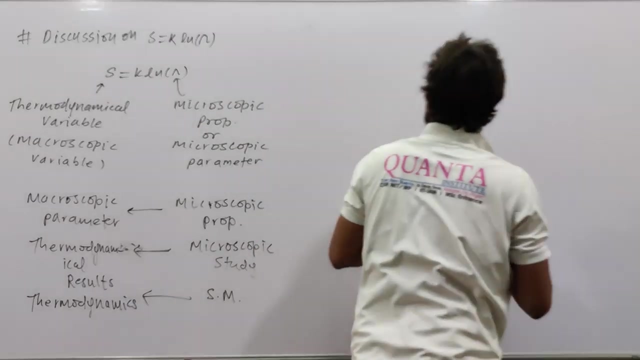 By microscopic study. you are able to obtain them from the macroscopic parameters. And there is some other point regarding this: See. This was the first point. Why is this so important? Next one is: See. S is equal to K, ln, omega. 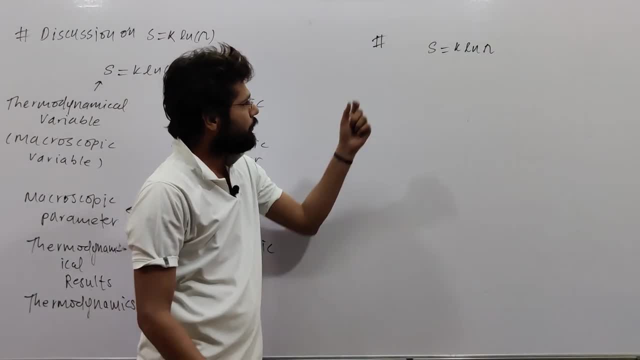 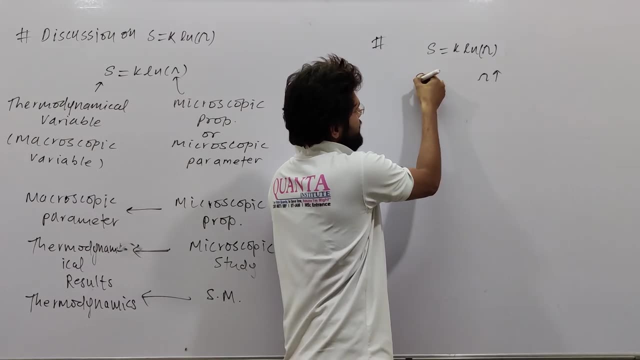 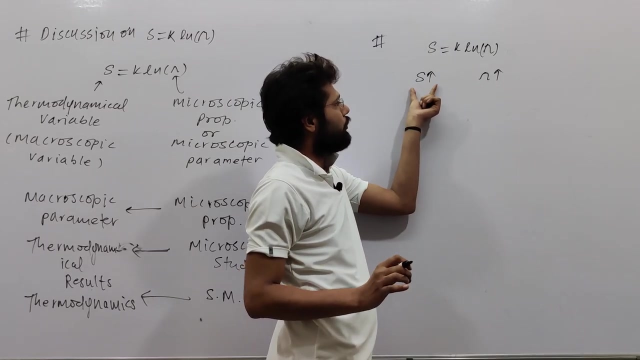 Okay, This is your relation And from this relation you can say that If omega is large, Means it is very large, Then S will also be large. If number of microstates is more in a macrostate, Then its entropy will also be more. 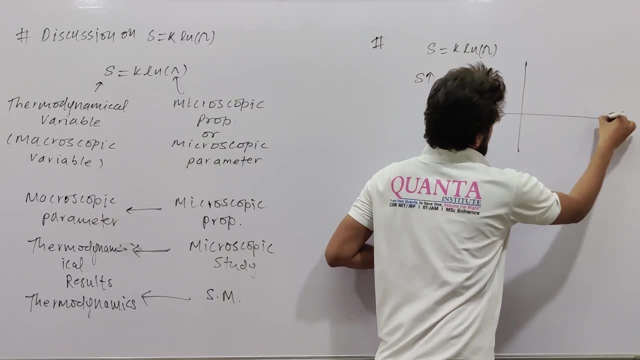 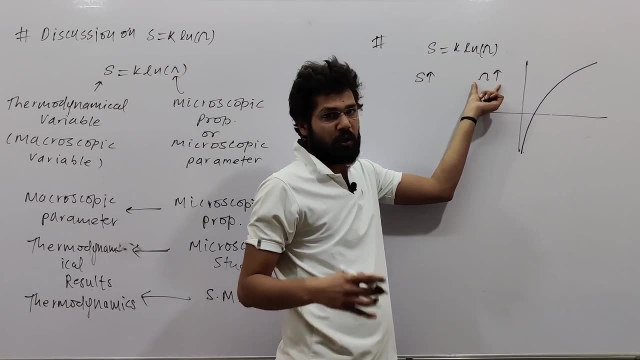 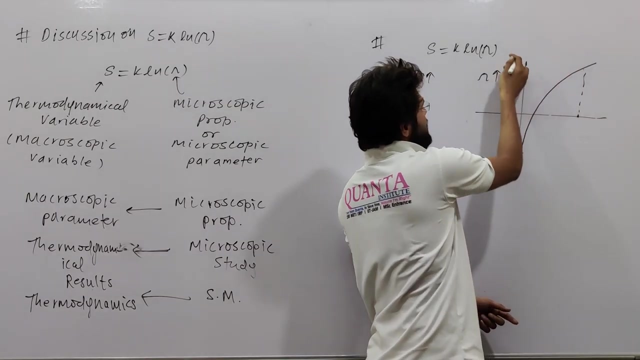 Okay, Because what is the curve of ln omega? The curve of ln omega is like this: And you know that number of microstates is a positive parameter, So it is a positive parameter And if it is very large, Then also nl omega is a large number. 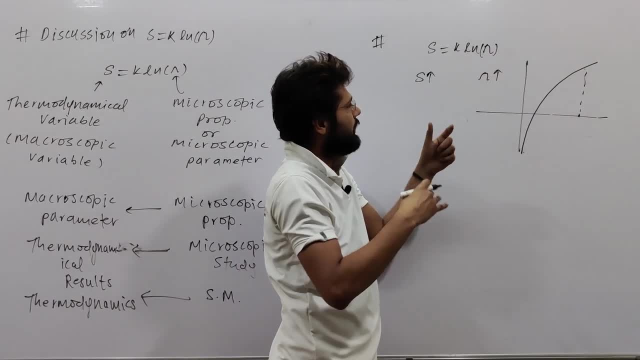 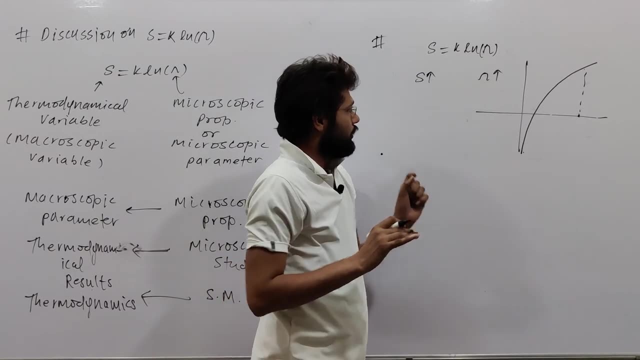 And if it is very large, Then also s will also be large. This is absolutely correct. Now let's talk about one thing from here. See The most probable macrostate, The largest number of microstates is there in it. 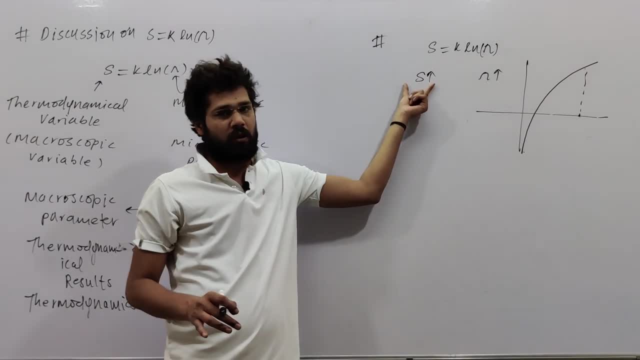 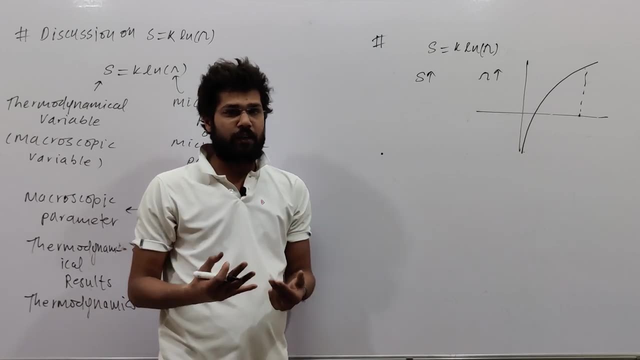 Then what will be its entropy? It will be largest. So I will pass a statement That most probable macrostate has largest entropy. This will be absolutely correct, Although this discussion was done yesterday also. Okay, Still, you see once. 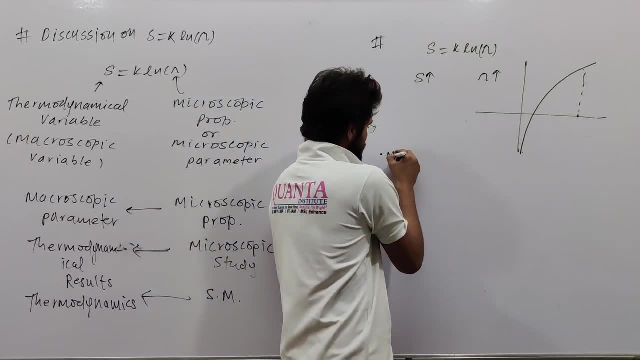 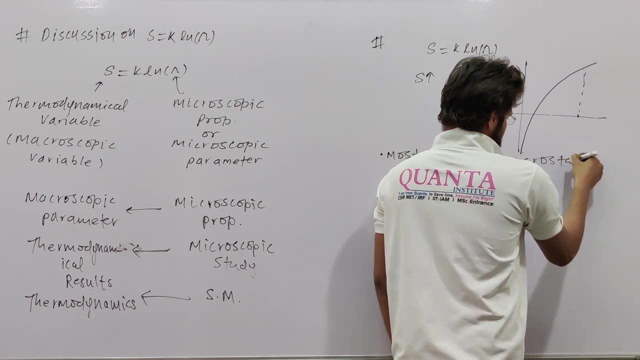 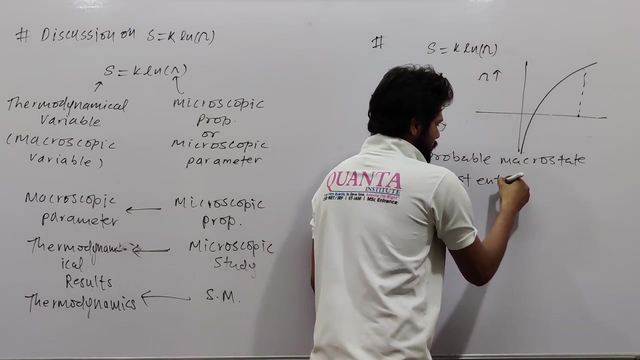 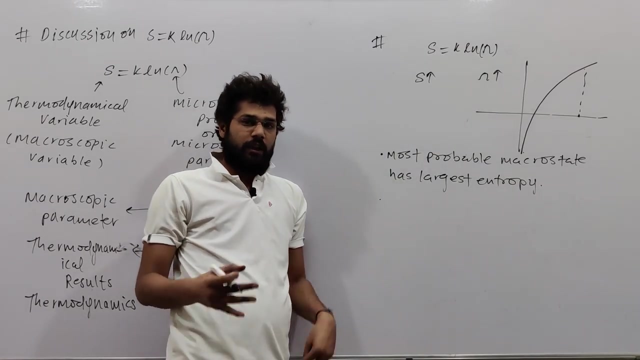 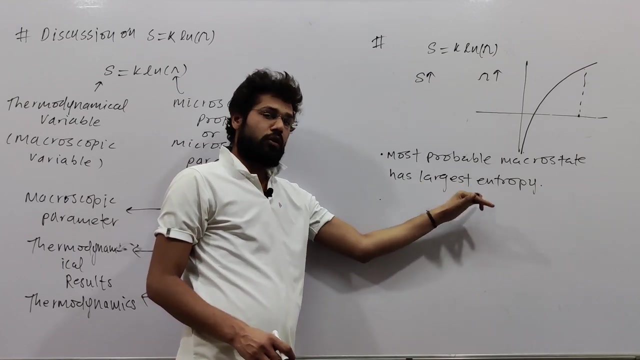 See: Most probable macrostate has largest entropy. It is absolutely clear from this discussion. And most probable macrostate is also equilibrium state of the system. So I can say The equilibrium state has largest entropy. I can say this Since: 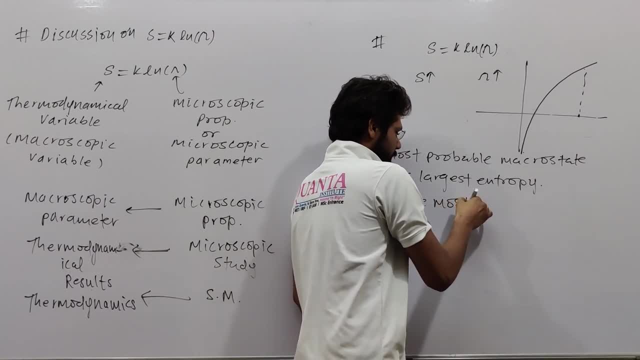 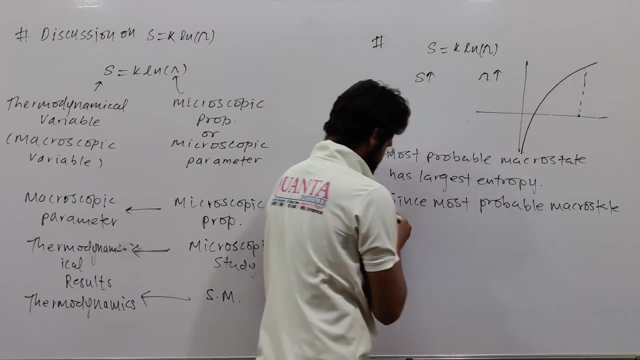 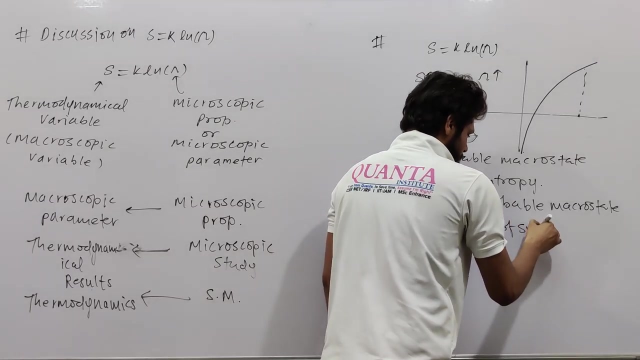 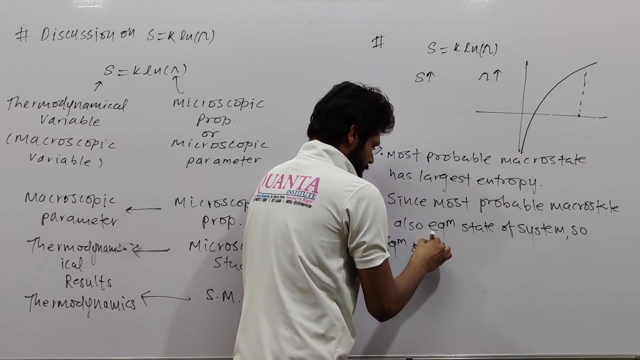 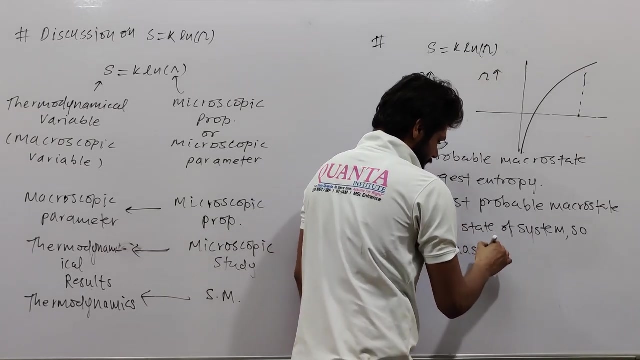 Most probable macrostate. Most probable macrostate Is also Equilibrium state Of system. So Equilibrium state Is also Entropy of the system. Okay, Okay, So is also, or has, the equilibrium state has largest entropy. 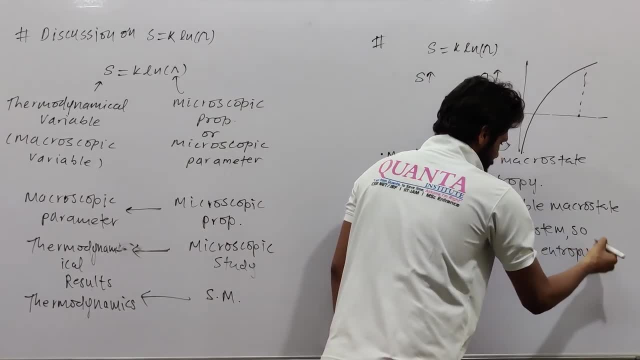 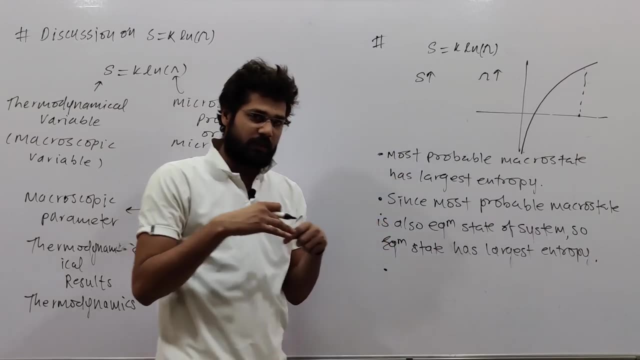 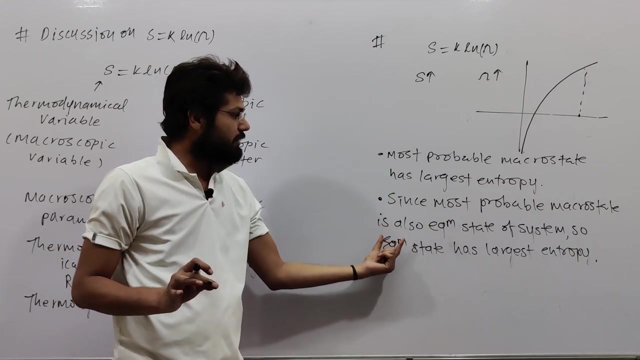 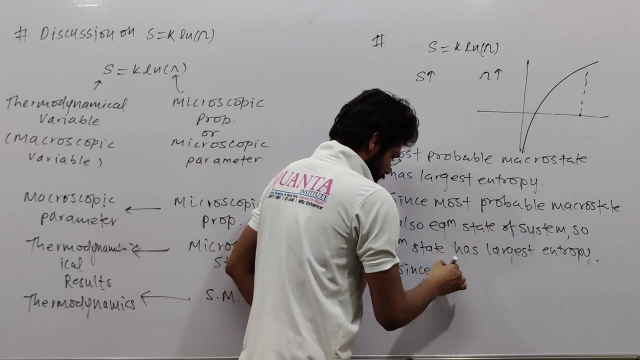 absolutely correct. largest entropy. in the equilibrium state, entropy will be largest, absolutely correct. and one more thing we can write: since entropy is measurement of disorderedness in the system, so the equilibrium state will be most disordered, since entropy is a measure of disorderedness. 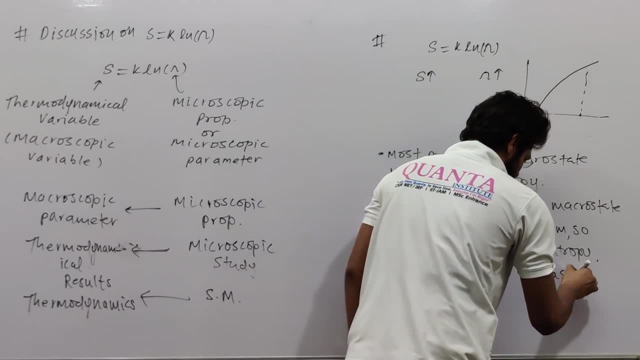 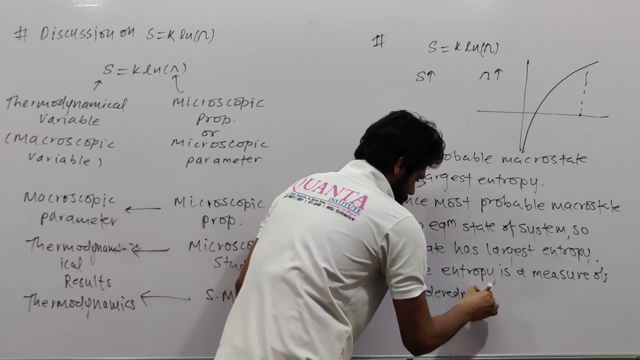 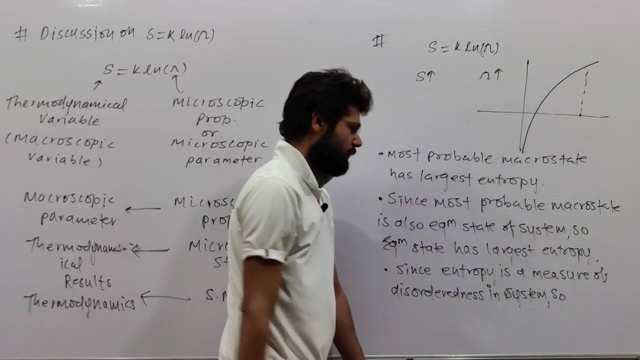 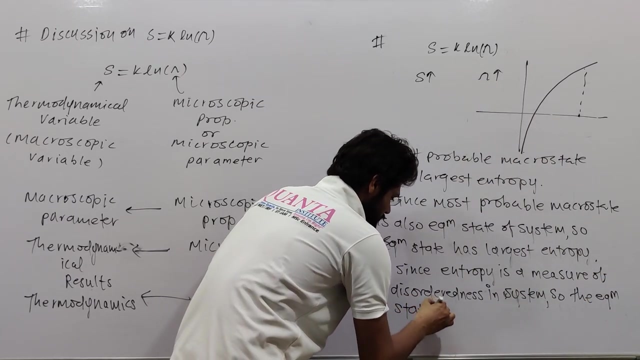 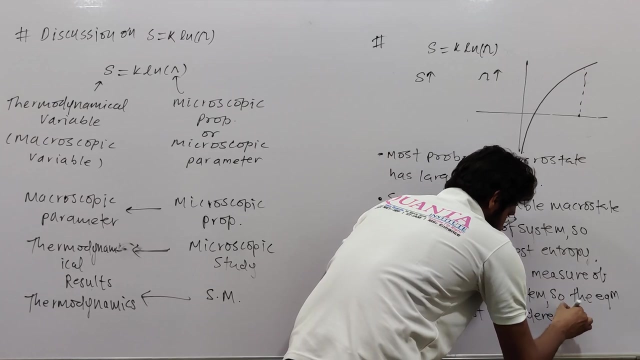 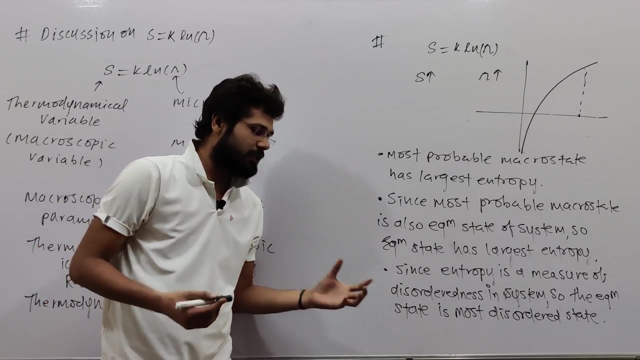 disorderedness in the system. so the equilibrium state will be most disordered, since entropy is a measure of disorderedness in the system, so the equilibrium state is most disordered state. ok, the realization of this is, as mentioned in yesterday's lecture, why it is most disordered. 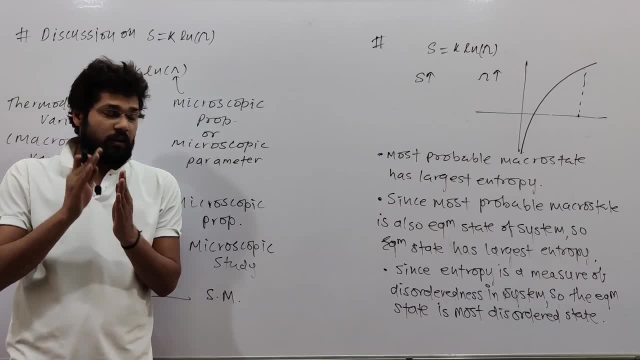 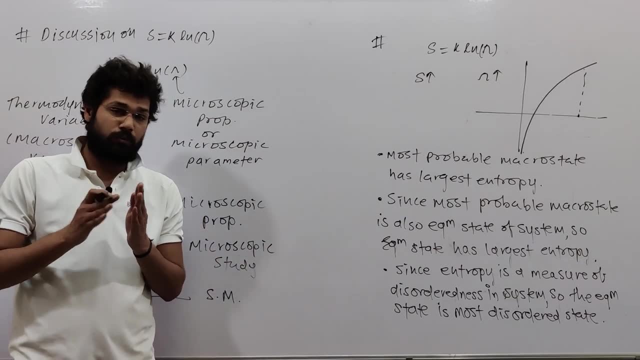 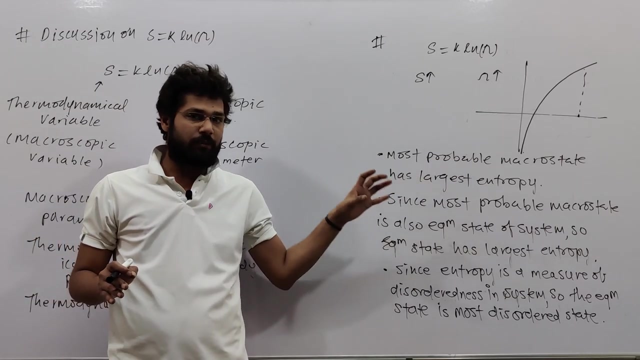 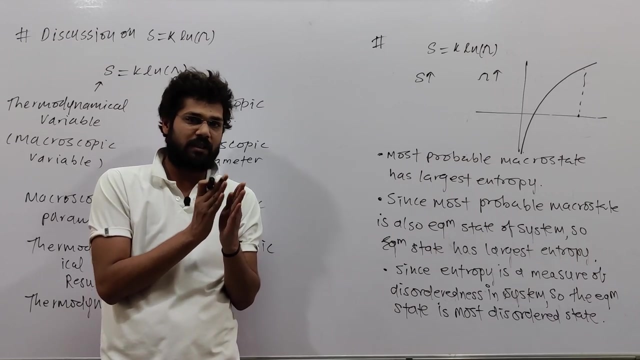 let me tell you again: because in equilibrium state the system passes through large number of disorderedness. there is most disorderedness, most disorderedness, in the equilibrium state because in the equilibrium state there is most microstate. what is microstate? a distinct internal arrangement. 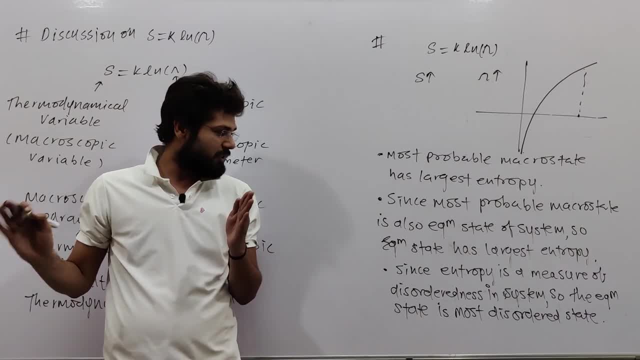 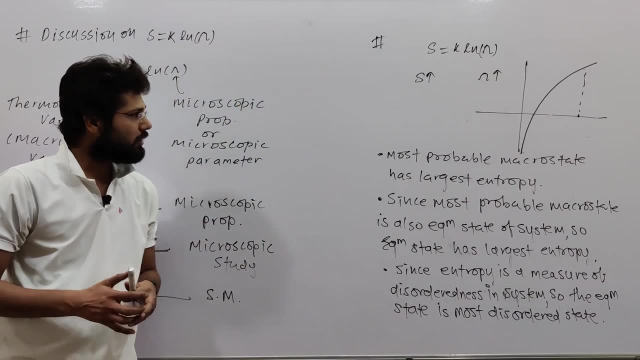 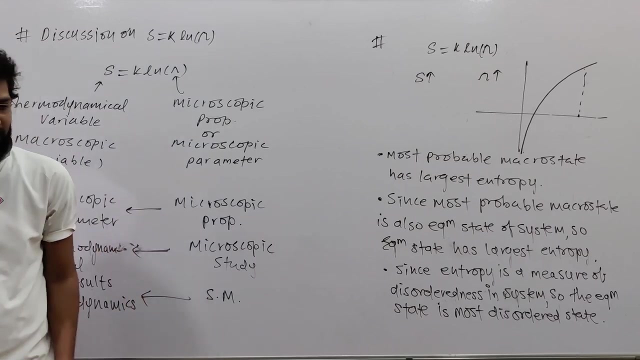 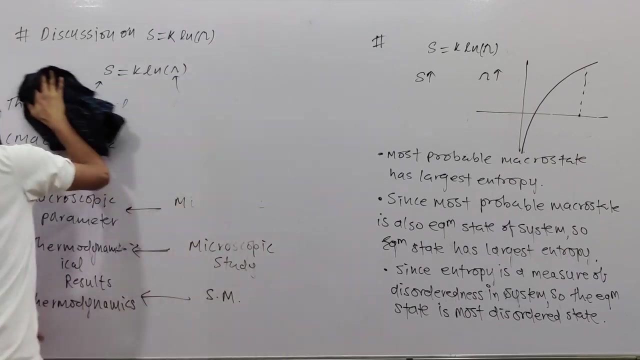 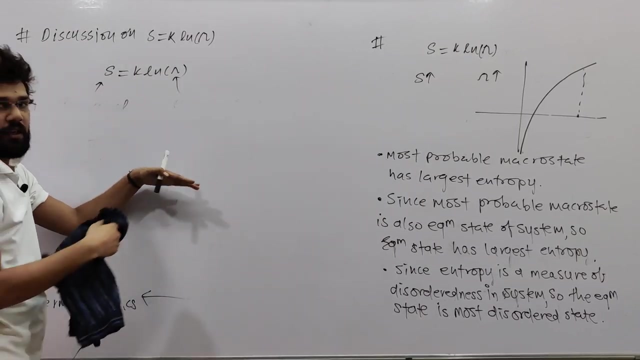 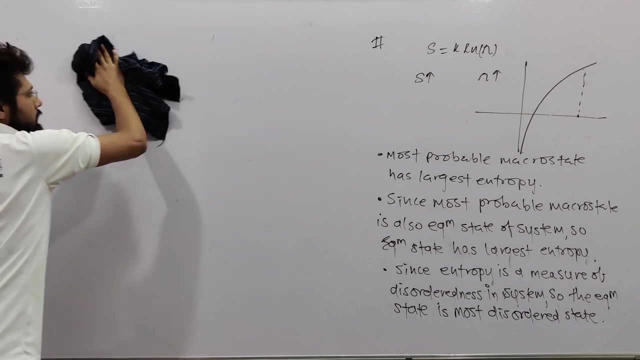 and what is the system? with time, various internal arrangements go through, so most disorderedness are there one more thing: that the equilibrium state is most unpredictable is also clear. next let's talk about. next in this discussion, there is third point. third point is what you can obtain. 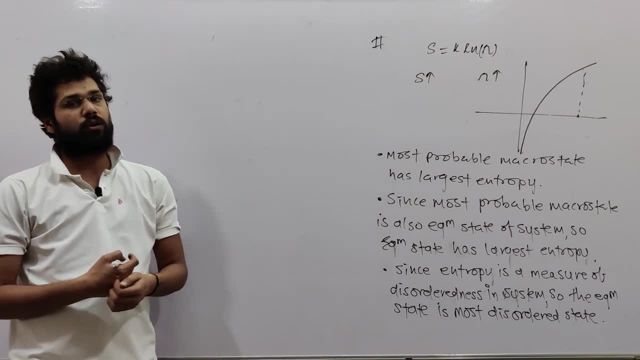 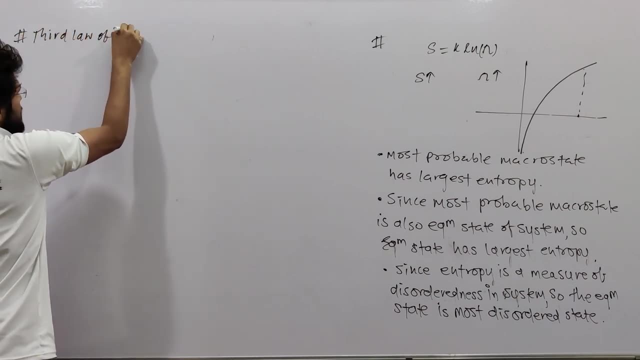 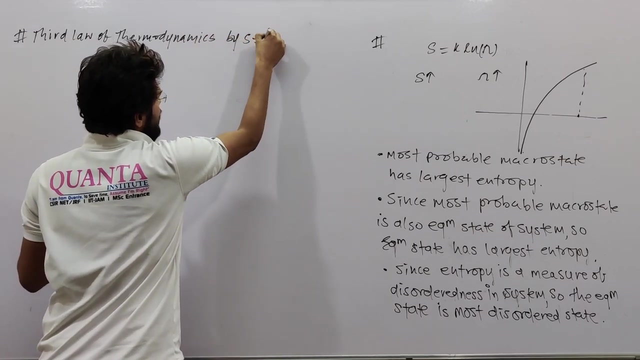 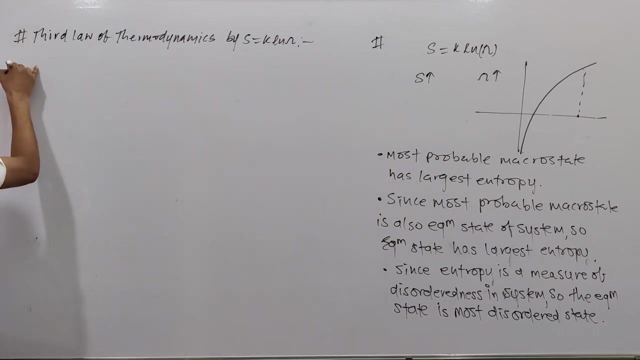 third law of thermodynamics by this relation by H-Thorum, let's see third law of thermodynamics. third law of thermodynamics, third law of thermodynamics by S equal to K, ln, omega by H-Thorum. how to obtain third law in thermodynamics, let's see: 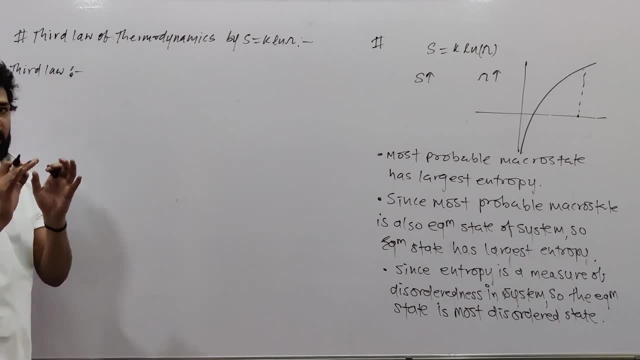 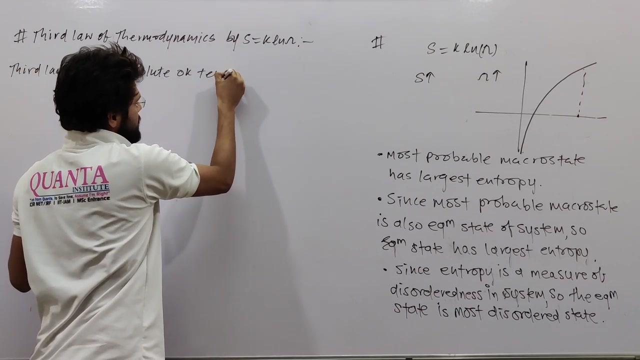 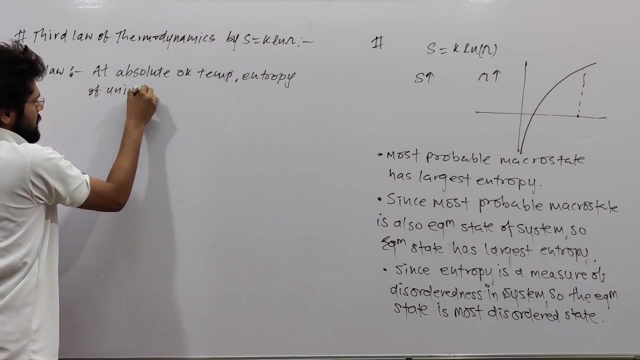 what is third law? according to third law, at absolute zero temperature, the entropy of the universe is zero. at absolute zero kelvin temperature- zero kelvin temperature- entropy of universe universe is zero. this is third law of thermodynamics. so let's see how to obtain this. 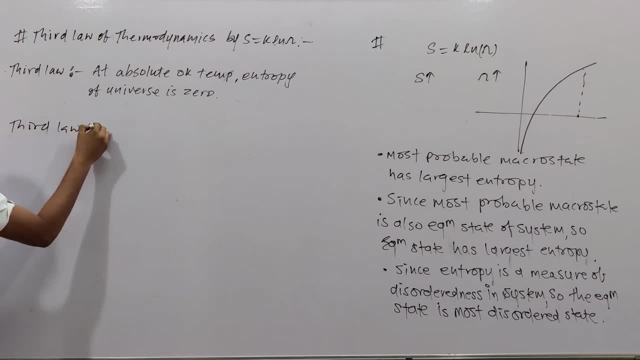 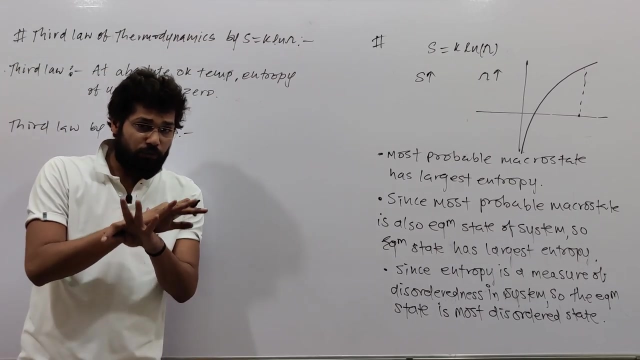 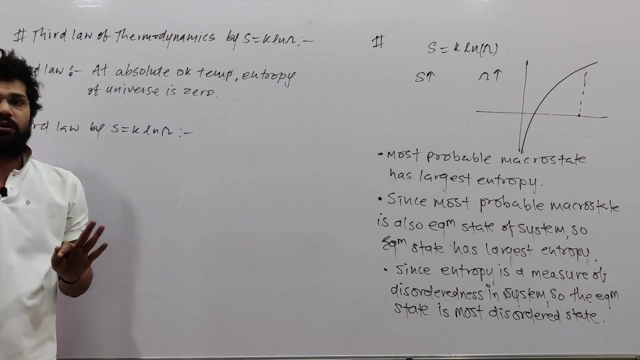 third law by s, s, s, l and omega. let's focus on what is the actual temperature of zero. at zero kelvin, all movements will be seized. nothing will move because kinetic energy will be zero, because kinetic energy depends on temperature. as you know what is vrms? 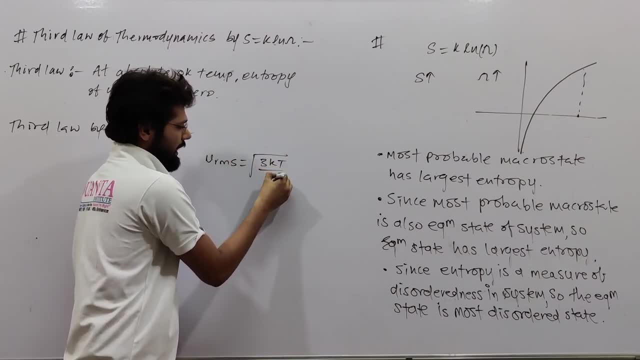 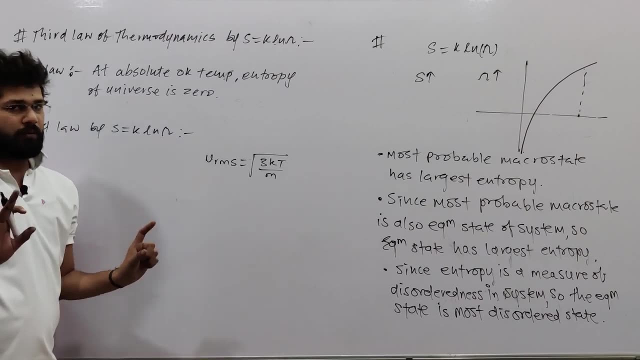 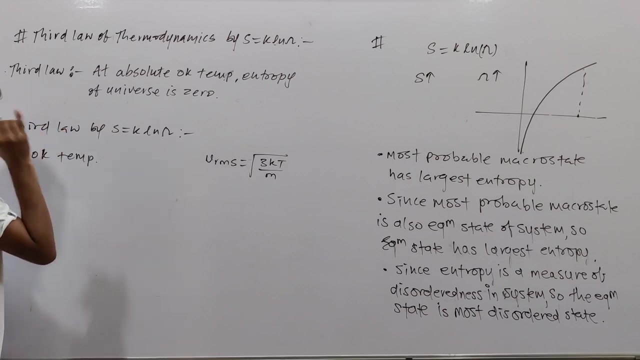 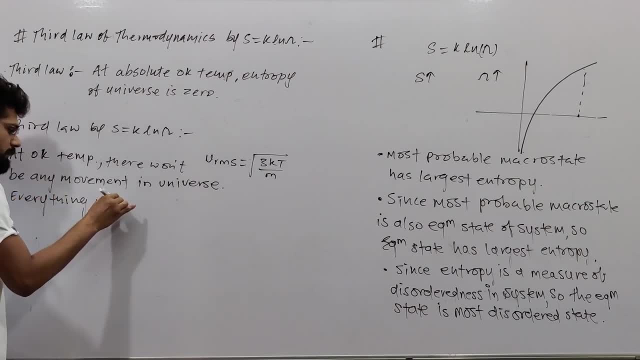 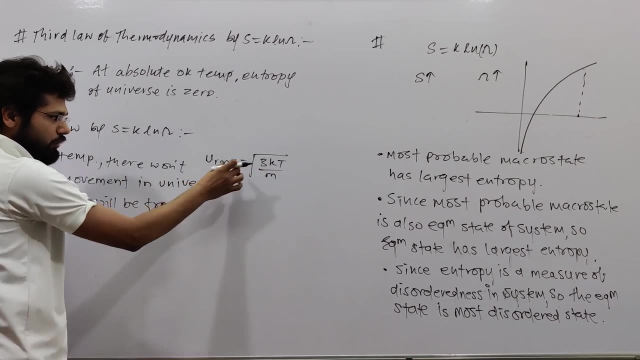 everything will be freezed. reason i have cleared here, because vrms is this: t is equal to zero, so vrms is zero, kinetic energy is zero. everything will be freezed, freezed. now. everything is freezed. you can say that universe is in a single state. 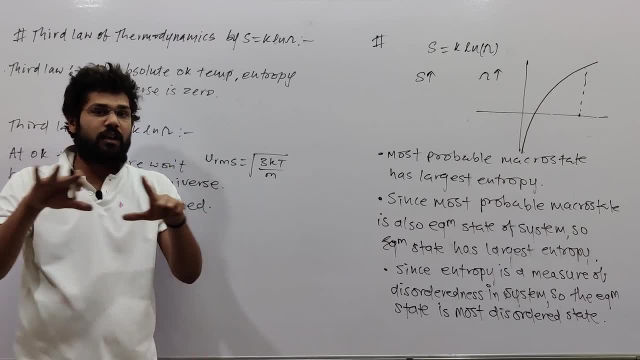 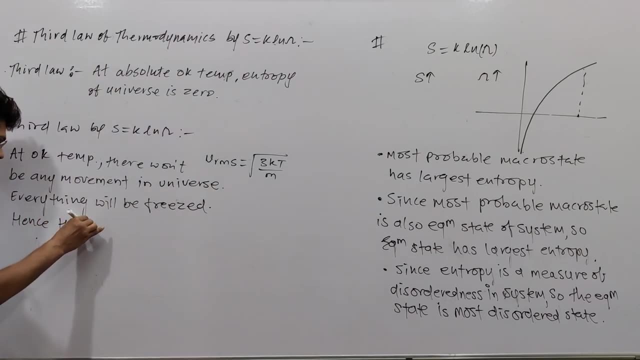 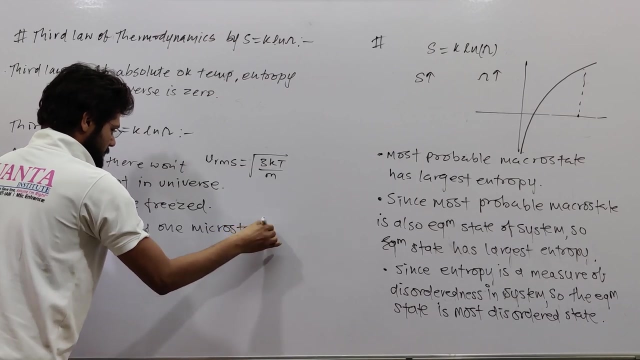 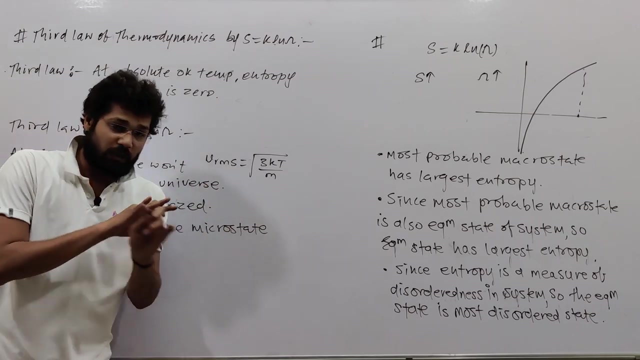 in a single micro state. universe has a single micro state at that time, is it right or not? and hence, there is only one microstate of universe, of universe, there is only one microstate. there is no internal arrangement because everything is freezed, is it right or not? 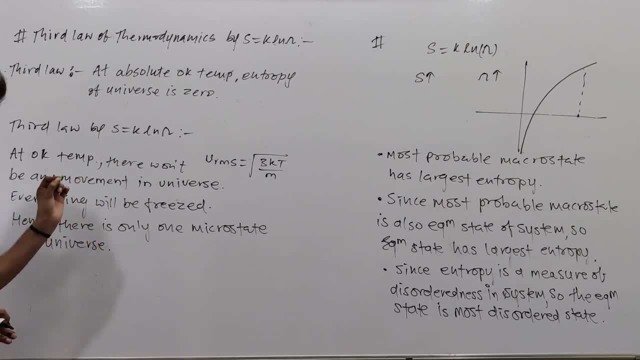 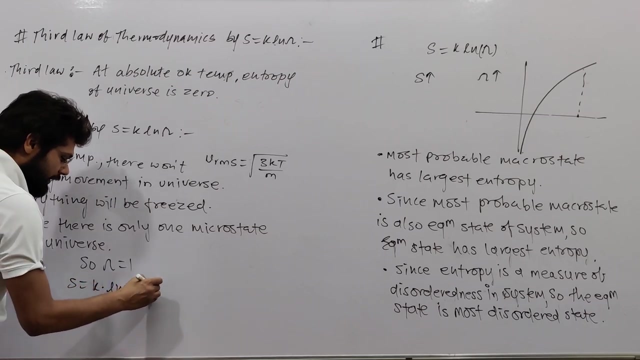 there is no internal arrangement. there is only one state in which your universe exists, there is one microstate. so omega equal to one and if omega equal to one, then by this relation, what will be the entropy? k? ln omega and k? ln omega is one. what is ln one? 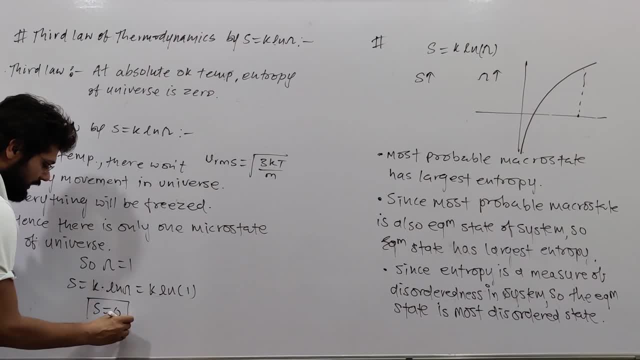 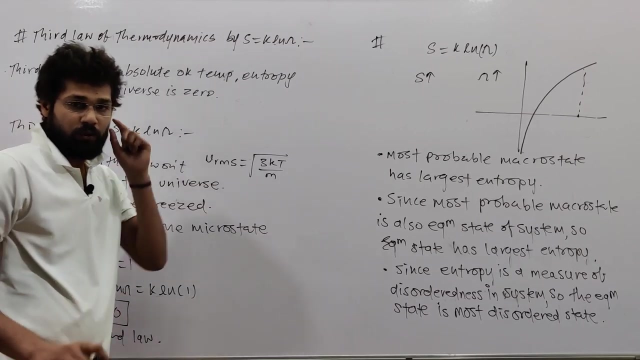 zero. so s equal to what zero and this is what third law, and it is third law of thermodynamics. so at zero kelvin, third law, third law: at zero kelvin, entropy will be zero of the universe, and this is third law. by s k ln omega. 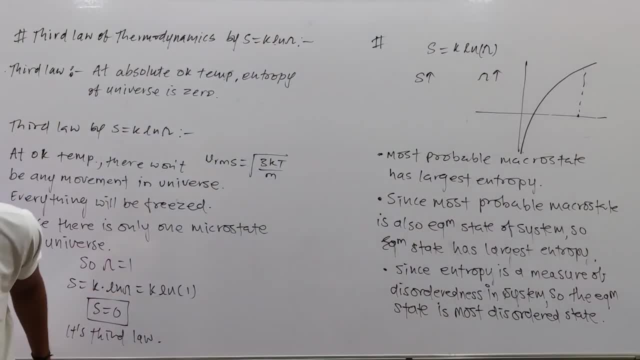 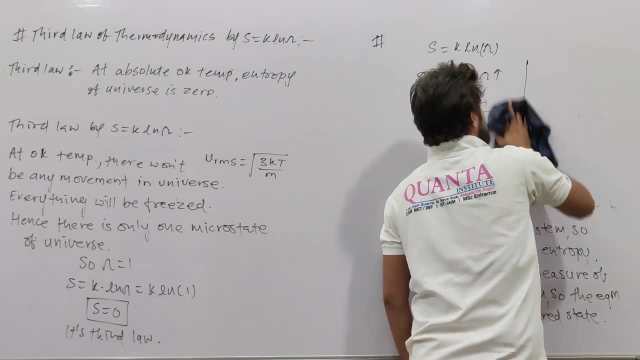 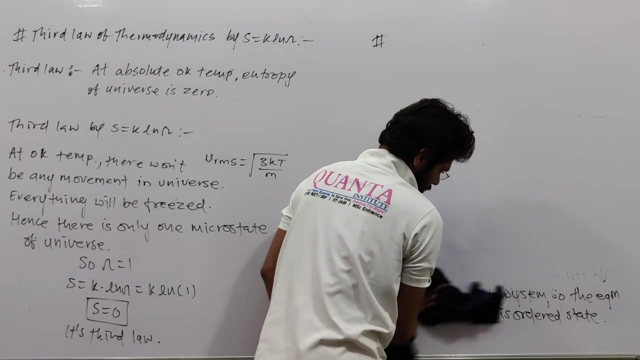 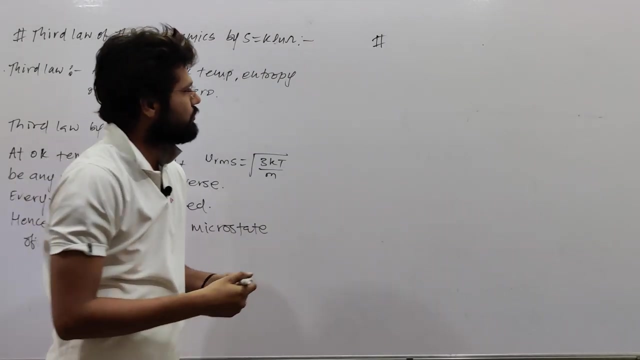 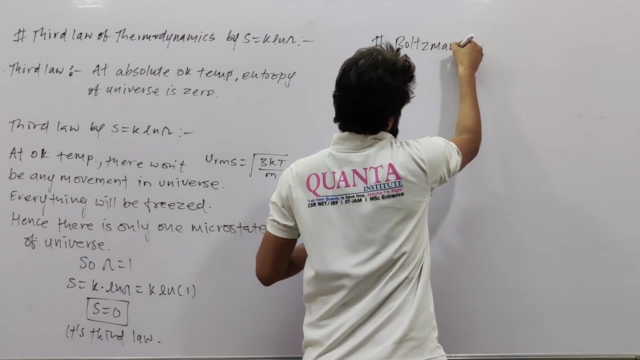 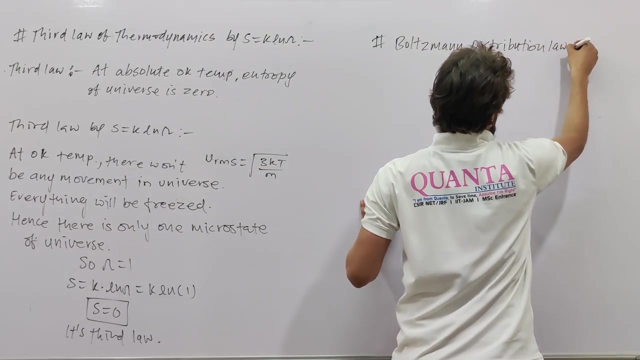 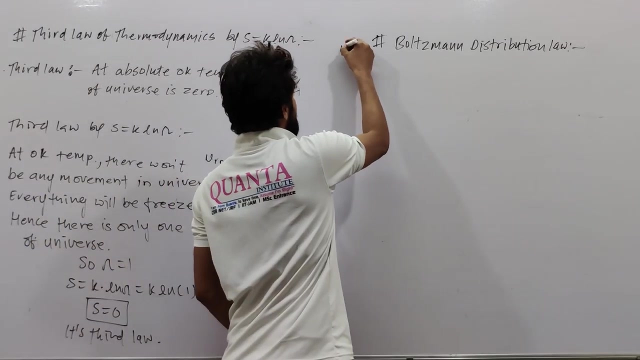 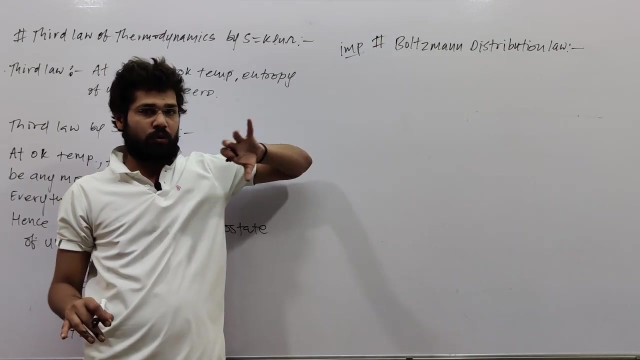 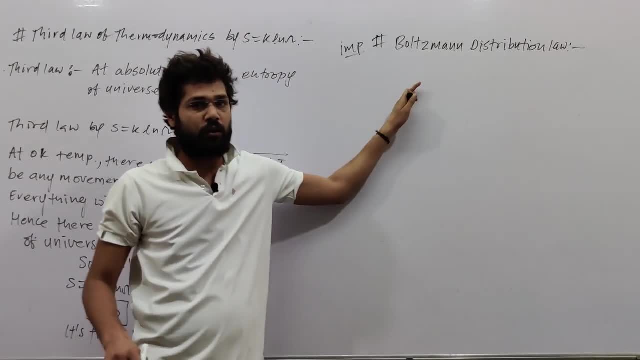 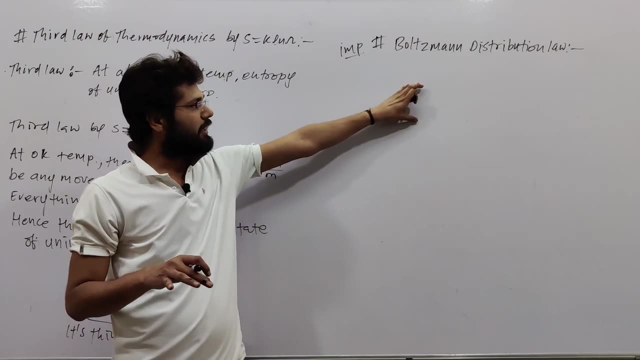 it many times. so the main problem in this question is that you do not know that the we don't know that we have to apply Boltzmann distribution. So here we will learn this thing also. First of all, we will learn that what is Boltzmann distribution law actually? 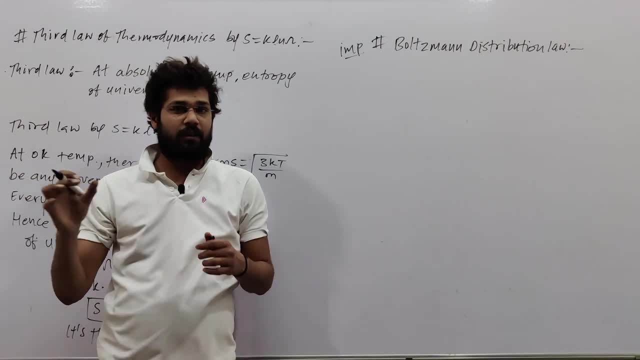 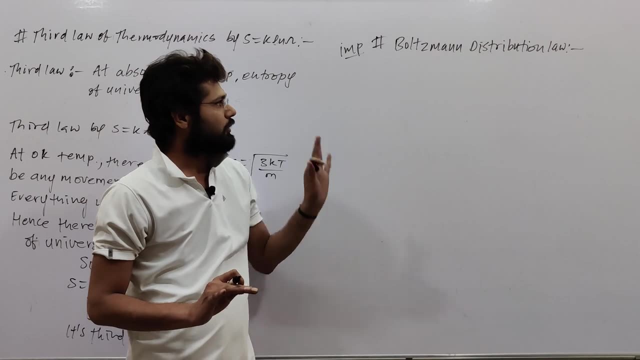 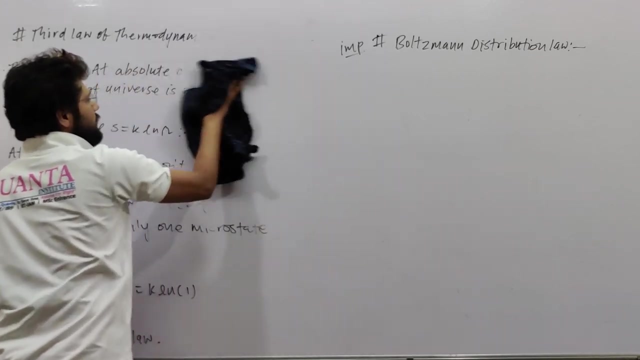 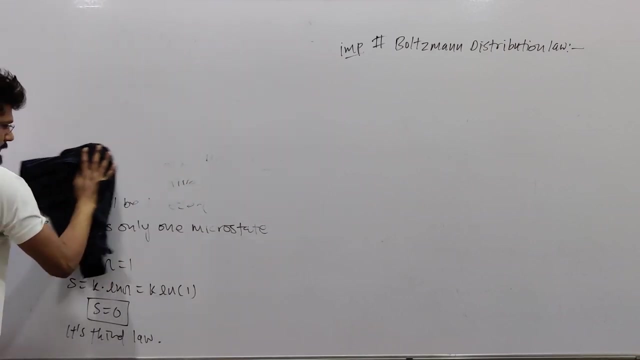 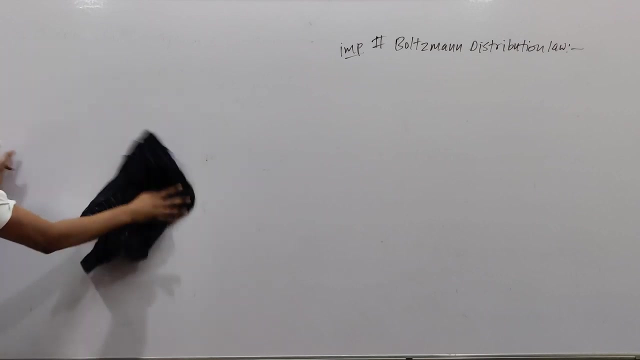 After that, how to identify from the language of the question that we have to apply it. So, first of all, what is it See? what is it Actually? what does it say? Actually, it tells you that, in an energy level, what is the average number of particles? 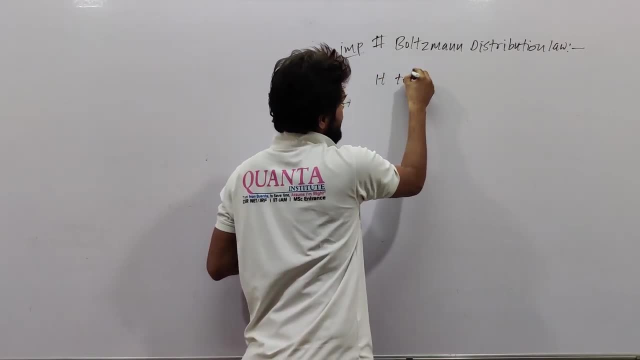 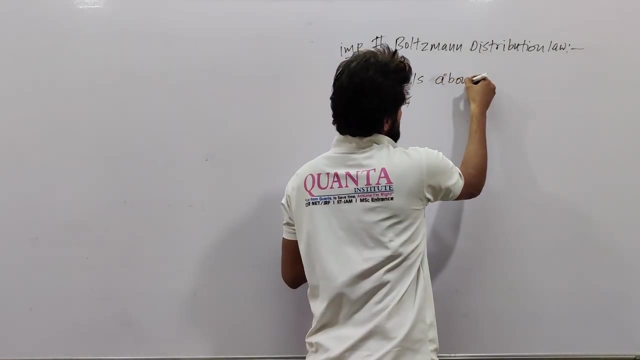 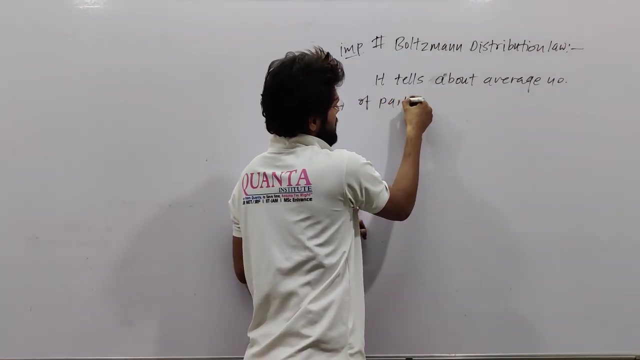 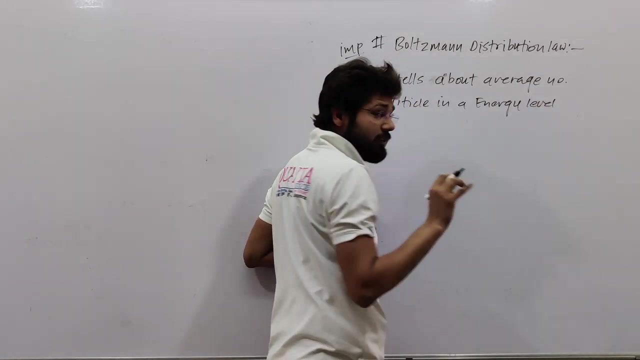 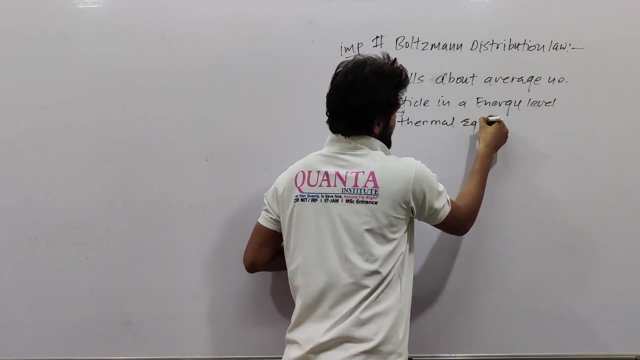 It tells about that. It tells about average number of particles. It tells about average number of particles. It tells about average number of particles in an energy level, at thermal equilibrium, At thermal equilibrium. This is more important If there is a system at thermal equilibrium. 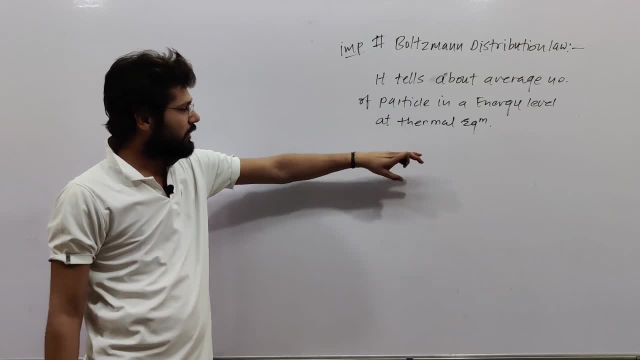 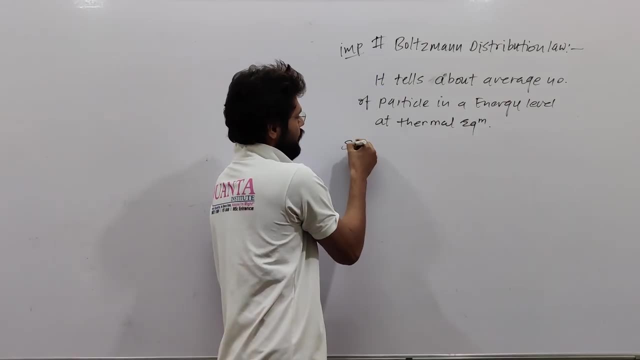 at that time, its energy levels or various energy levels, the average number of particles at this level. how much does it tell? Okay, Let's write what is its statement, What is the statement of the law. See what is the statement. 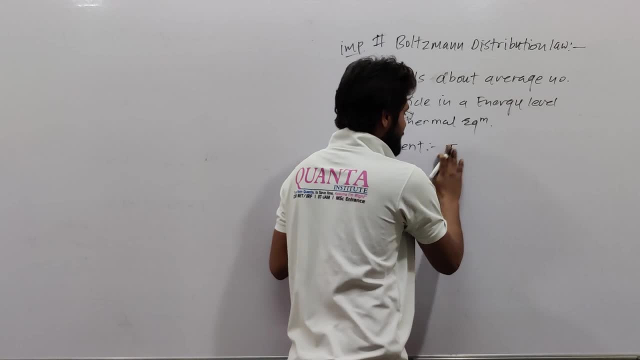 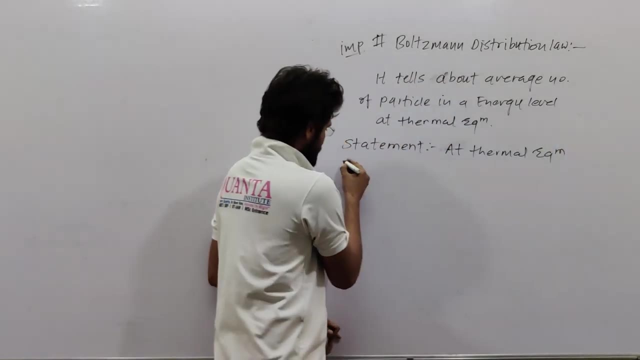 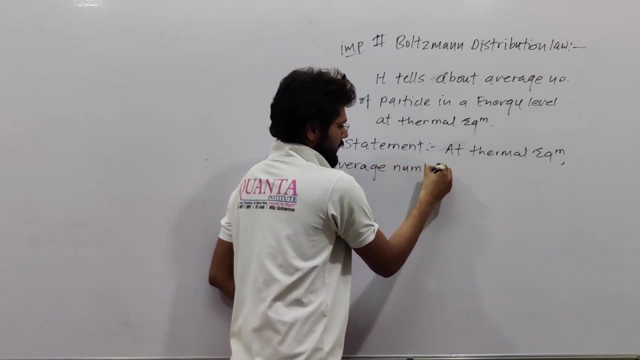 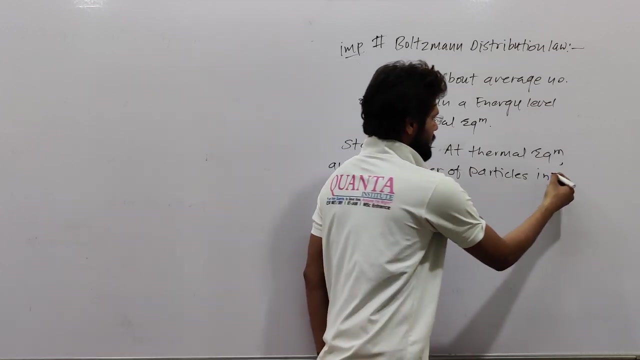 The average number of particles at thermal equilibrium. First of all, let's write at thermal equilibrium: At thermal equilibrium: Average number of particles. At thermal equilibrium: Average number of particles. Number of particles In an energy level. In an energy level. 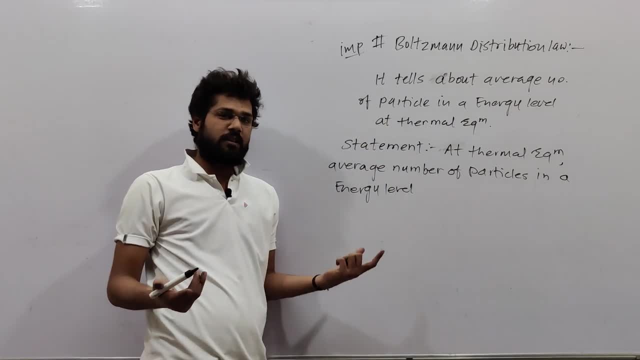 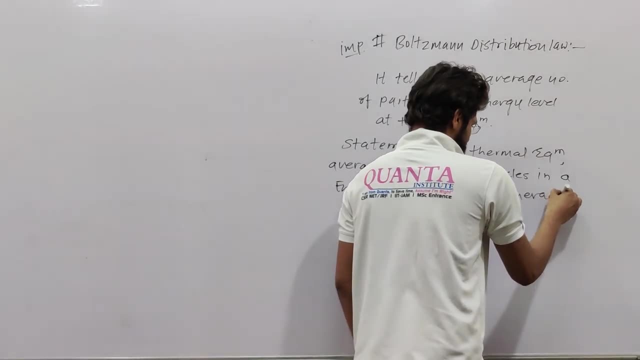 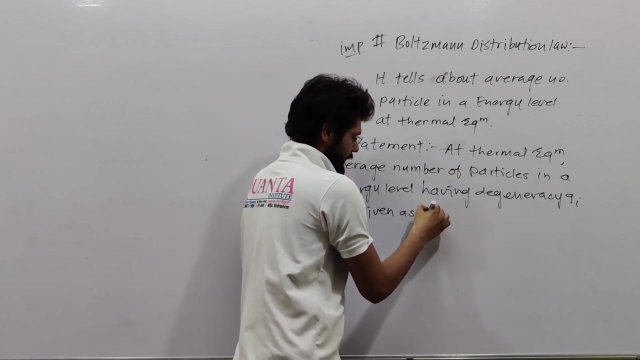 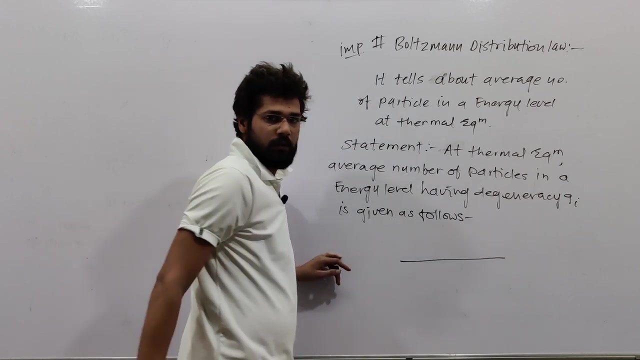 Energy level Having degeneracy GI. Energy level can be degeneracy, Having degeneracy. degeneracy GI is given as follows: Is given as follows: What happens? There will be a level. Okay, This is EI level. 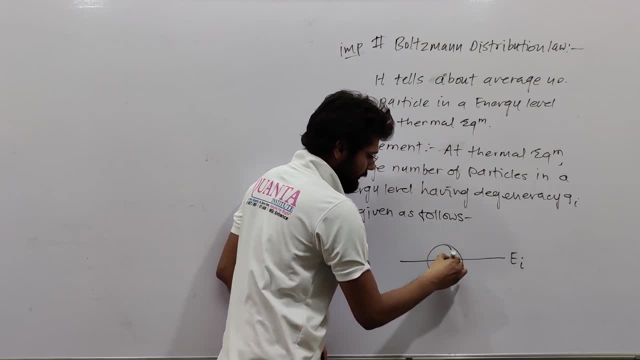 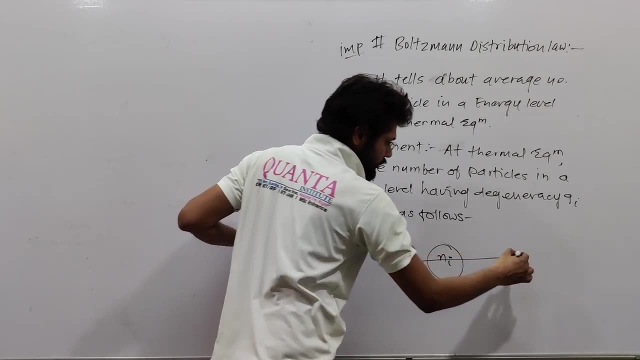 Okay, In this the average number of particles. I will say that the average number of particles is NI. So what will be NI? It is talking about that, And the degeneracy of this level is GI. Okay Then, average number of particles. 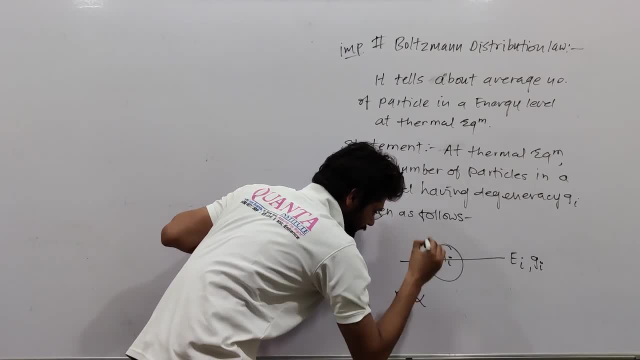 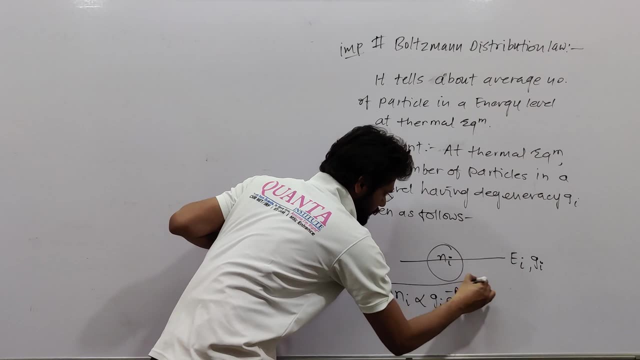 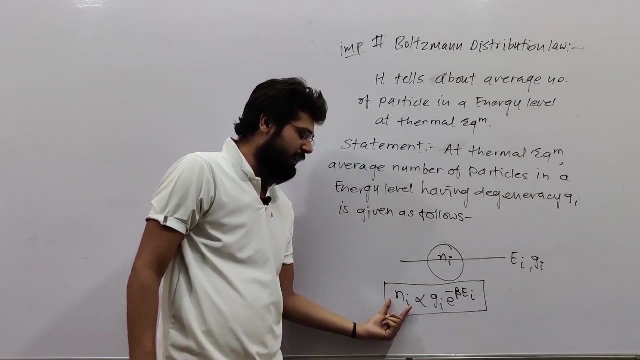 by Boltzmann distribution law is given as this way: Beta EI, This is your Boltzmann distribution law. The special thing is that there is a sign of proportionality here. This does not give the average number of particles exactly. It tells that the factors will be proportional. 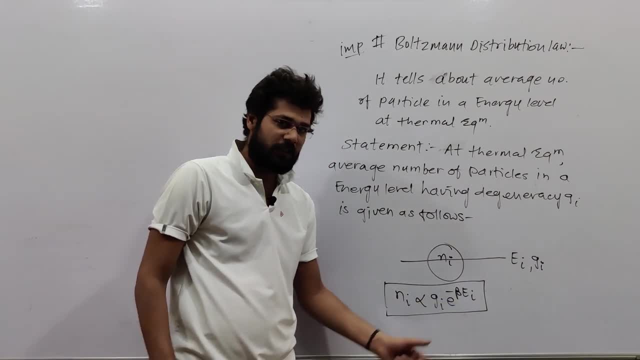 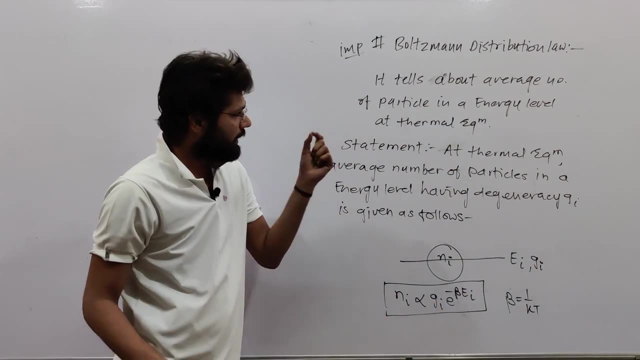 Okay, The unknown factor here is beta. What is beta here? So beta is 1 by kT. 1 by kT. What is T? The temperature at which your system is on the thermal equilibrium. Okay, T is temperature and thermal equilibrium. 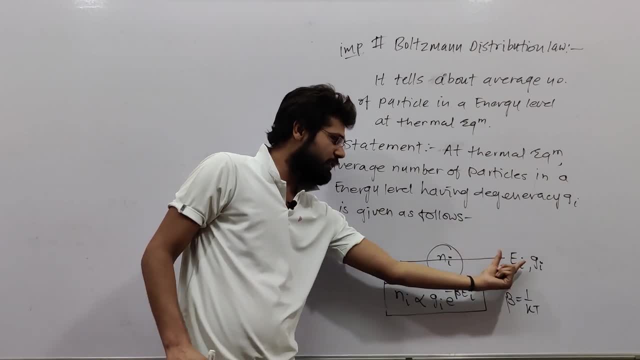 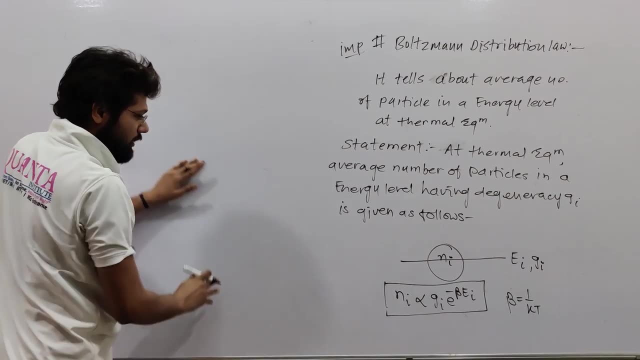 Okay, And the level of EI is being talked about. GI is the level of degeneracy, NI, obviously, is the number of particles, Average number of particles. Okay, Now, first of all, let us learn some other things. There will not be one level in the system. 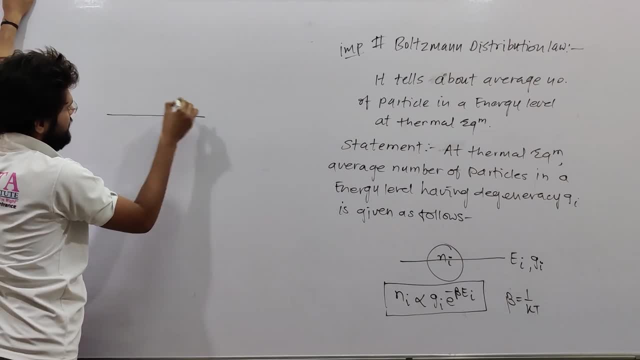 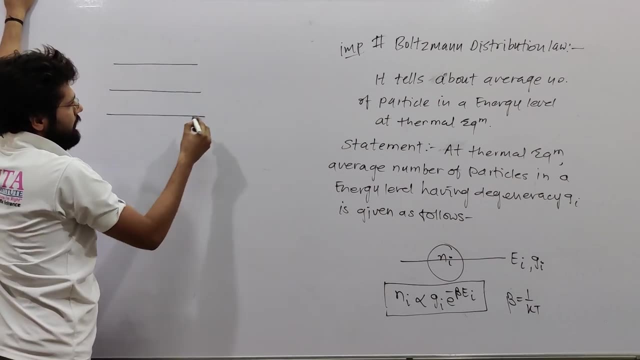 There can be many levels. So let's say you have three levels in the system And the system is always on the thermal equilibrium. Okay, From this type you have three levels. Let. this one is E1 level, This one is E2 level. 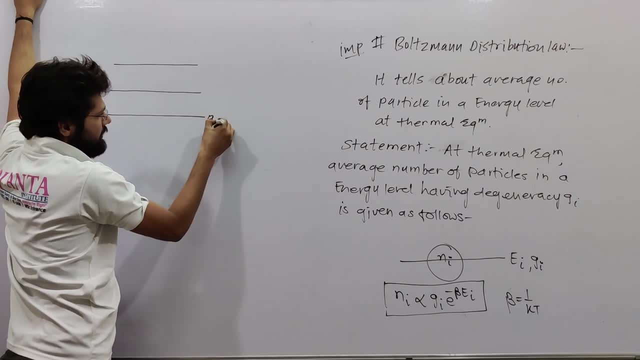 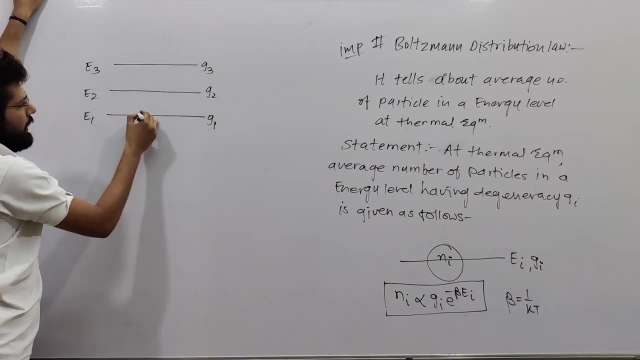 This one is E3 level And its degeneracy is G1.. This one is G2.. This one is G3.. Let the average number of particles are here: N1.. Here is N2.. Here is N3.. Okay. 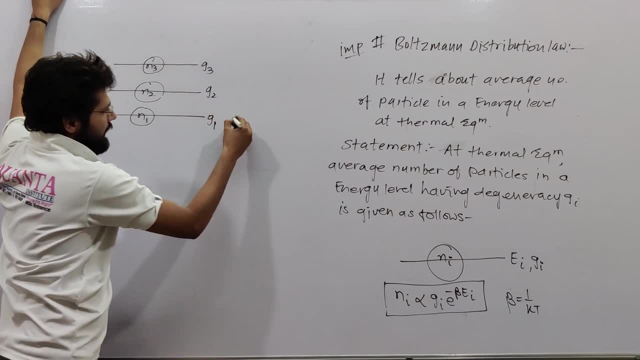 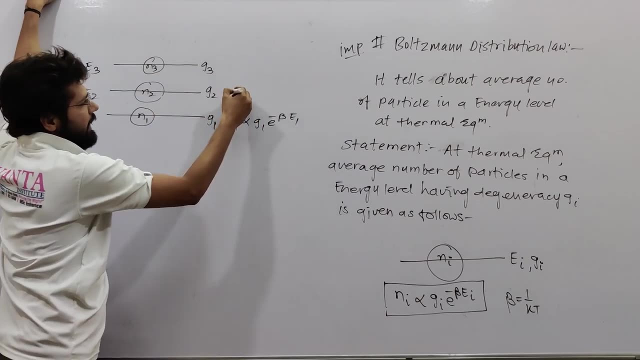 And there are only three levels. So you know one thing: What will be N1? Proportional to G1.. E power minus beta- E1.. What will be N2? Proportional to G2.. E power minus beta- E2.. 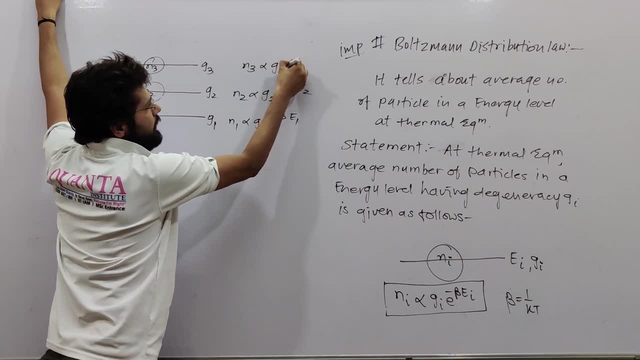 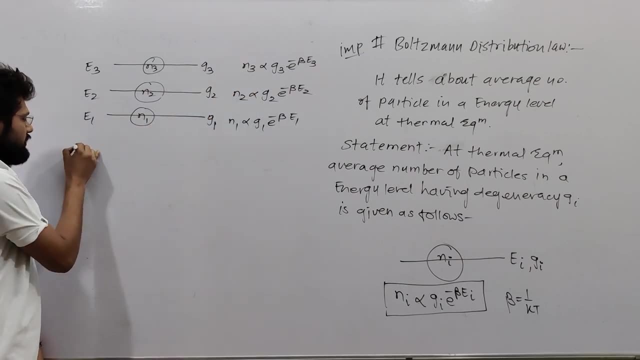 And what will be N3?? Proportional to G3. E power minus beta E3. By distribution law. And one thing you should be clear: The total number of particles. Write it in the system. How many will be there? 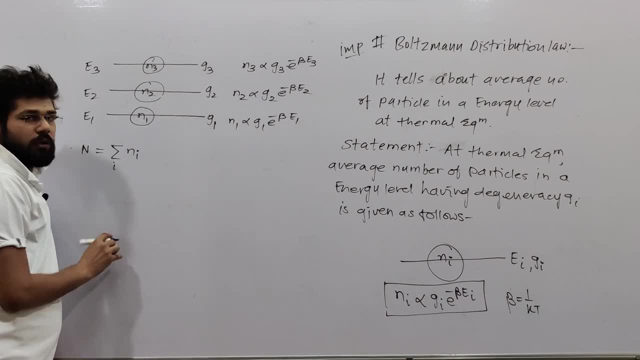 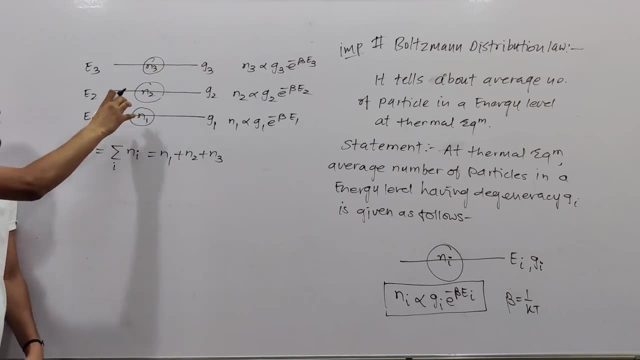 Obviously, summation Ni Will there be or not. That means N1 plus N2 plus N3.. These are three levels. Here is N1 particle, Here is N2 particle, Here is N3 particle. So what will be the total number of particles? 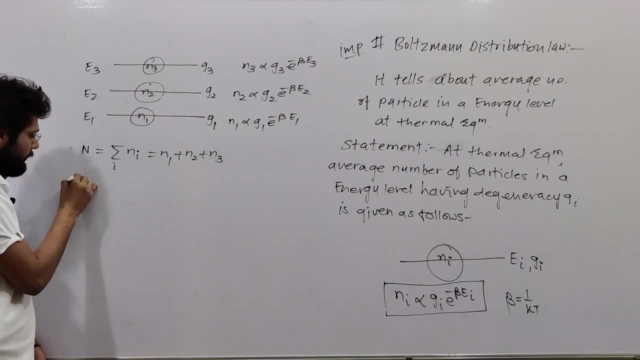 It will be this thing. Okay, So you can write the total number of particles like this: How is it? N1.. Now there is a proportionality sign in N1.. What should I write in N1?? Take some constant here. 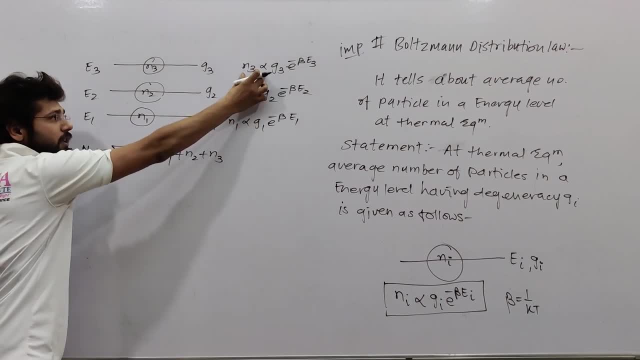 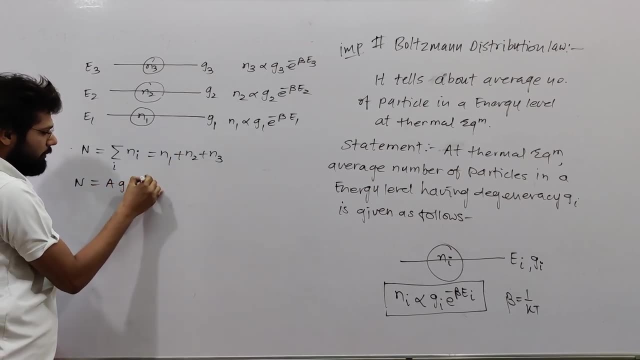 Take some constant A. Take the same constant here. Take the same constant here. Remove that proportionality sign. So A: G1. E power minus beta: E1. Plus A. G2. E power minus beta: E2. Plus A. 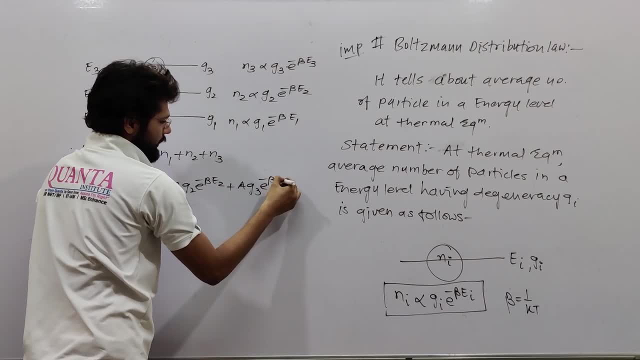 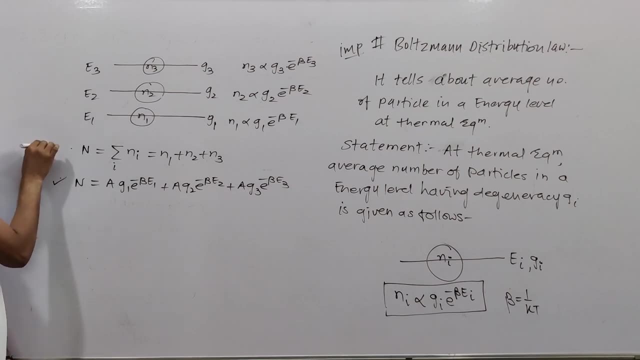 G3.. E power minus beta E3. Will N be given by this type or not Absolutely. Similarly, you can obtain one more thing here: What will be the total energy of this system? What will be the total energy See? 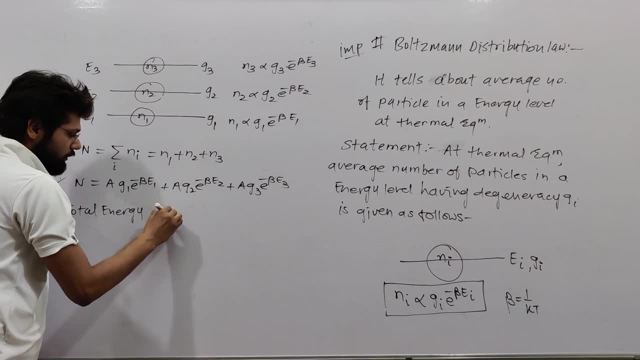 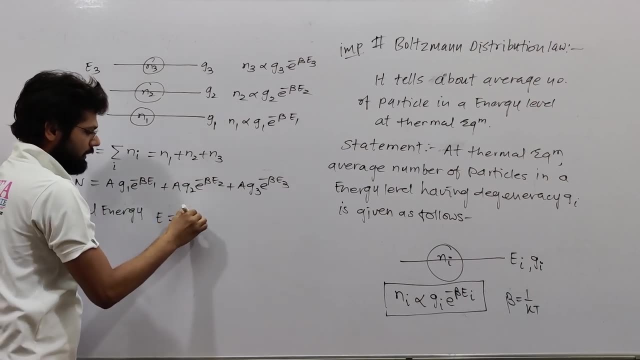 What is E? equal to Brother. there is N1 particle in E1 level, So N1 particle, E1.. Do it like this: E1 is the energy of one particle And there is N1 particle. The total energy of the whole system is E1.. 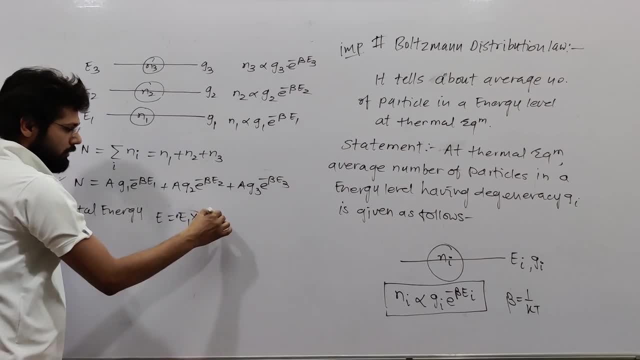 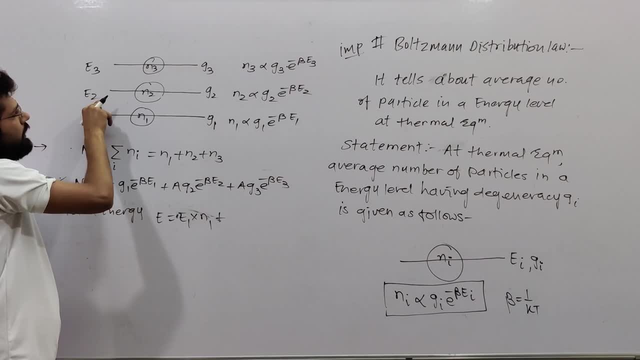 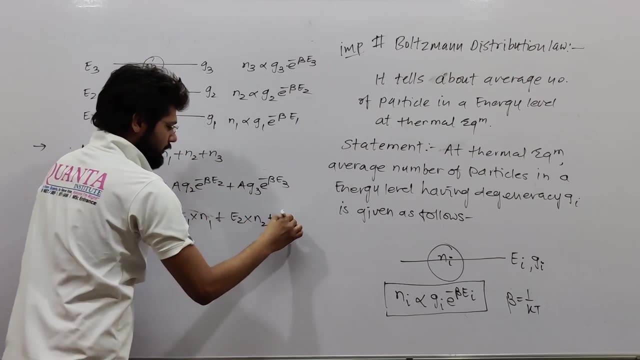 Then the energy of every particle will be counted Here here in the E2 energy level there are N2 particles. So what is the total energy? This Here? here are N3 particles. So this happened here. Okay. 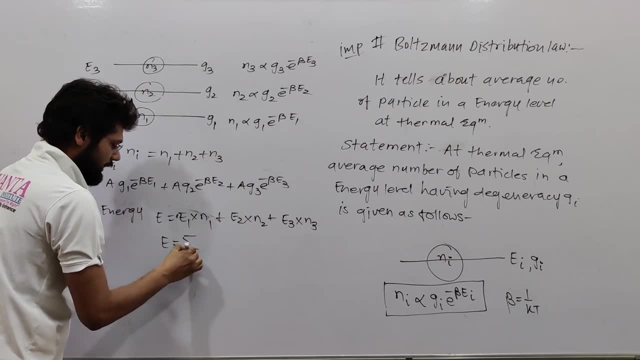 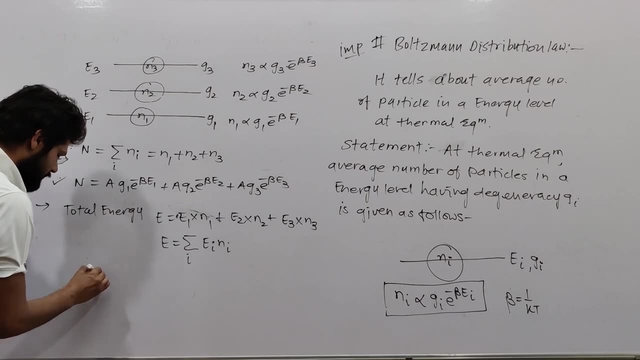 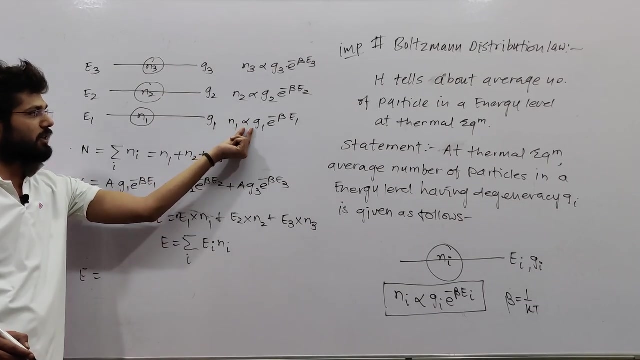 If I want to write this in general, Then summation i EI NI. You can write it like this: Now again, where will this relation give you? How are you able to write this further: e1, introduce n1 and add proportionality sign and use some constant a. 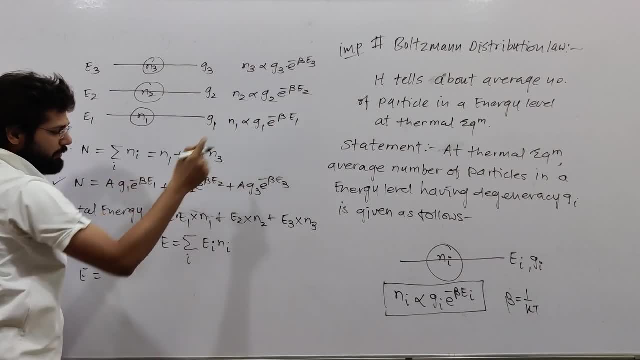 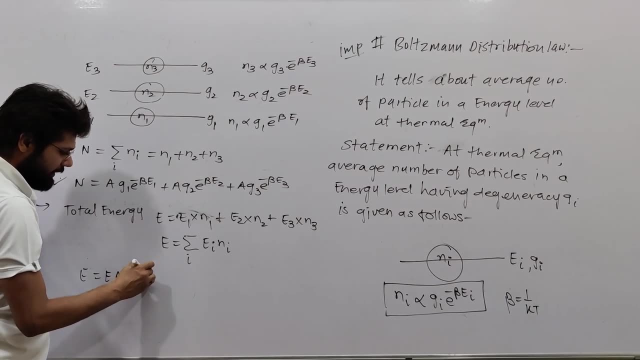 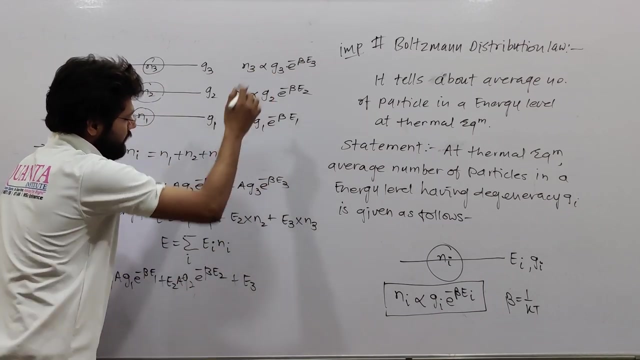 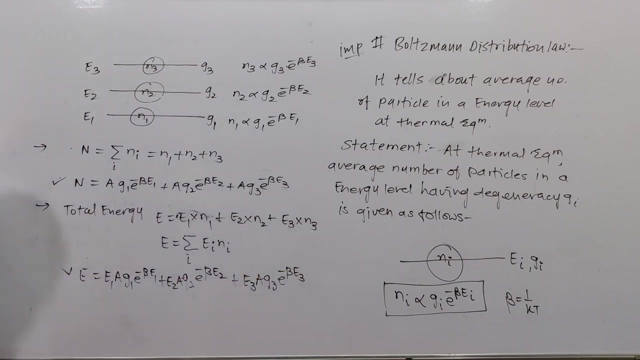 so instead of n1 I will write ag1- e-beta e1, so it will be e1- ag1- e-beta e1 plus ag2- e-beta e2 and e2a plus e3 and n3. ag3- e-beta e3. this is your second relation. 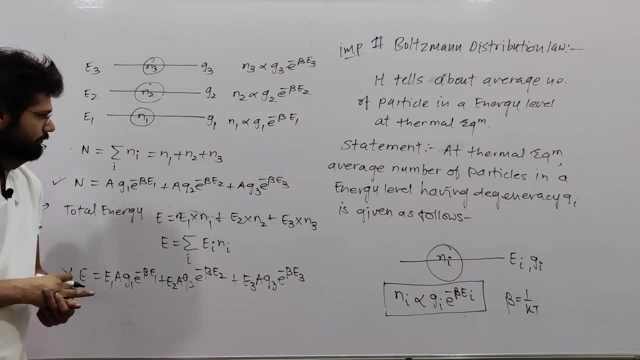 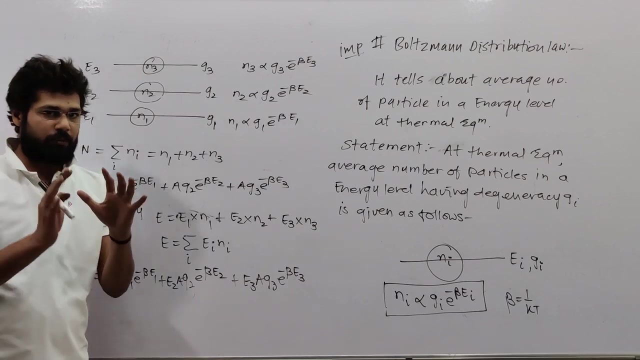 why am I doing this? actually, when you face a problem in the Boltzmann distribution law, sometimes you have to do this, so I have given you an idea that this will happen there. you should be clear about this. now let's talk about how you will identify the question. 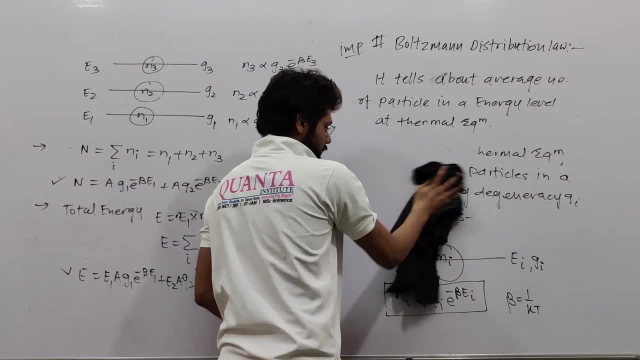 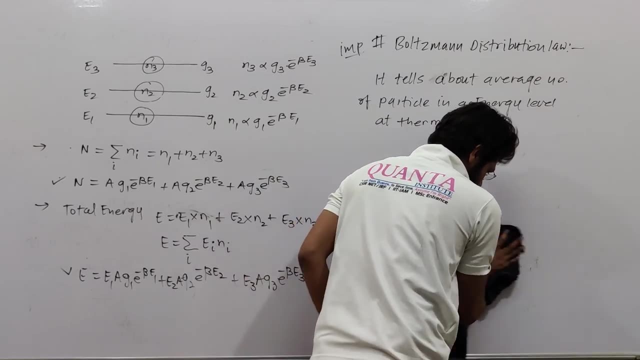 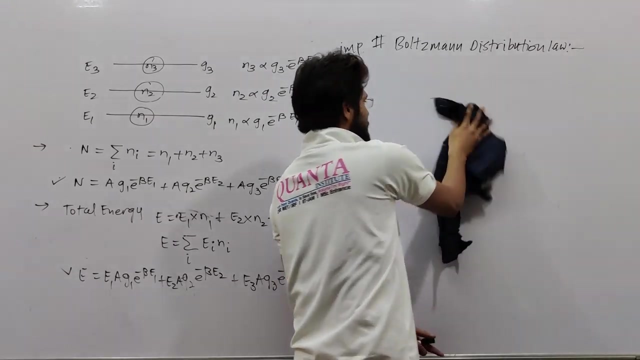 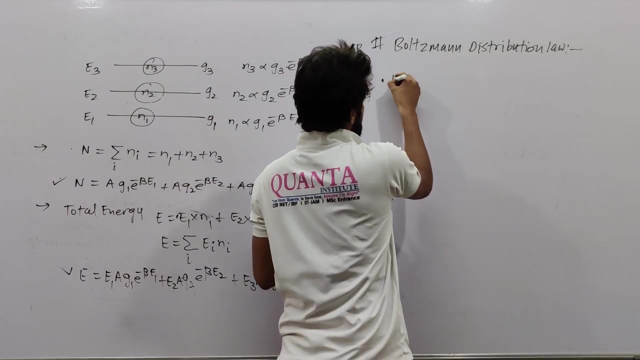 let's move on. how you will identify the problem of Boltzmann distribution law: see, I am telling you this because generally you can't get to the answer. I will also clear the reason why you can't get to the answer. see how to identify the problem. 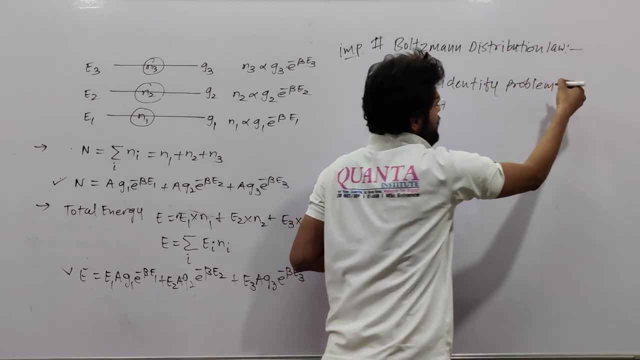 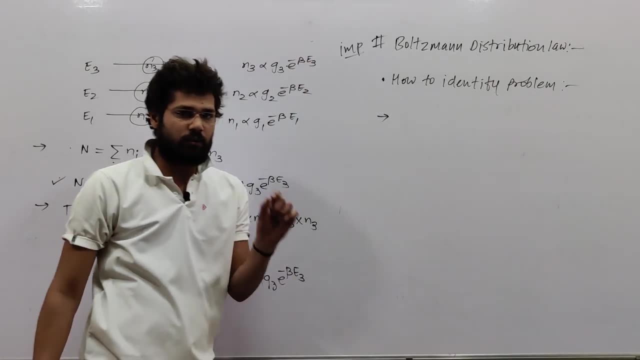 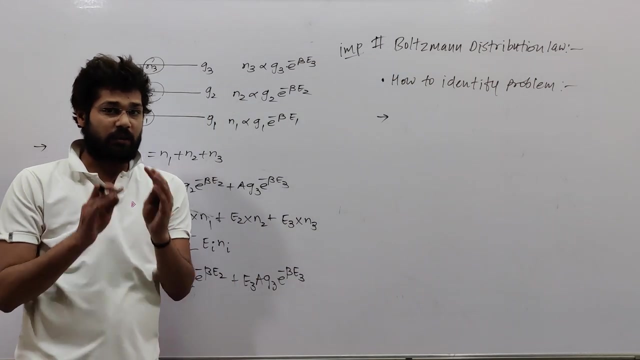 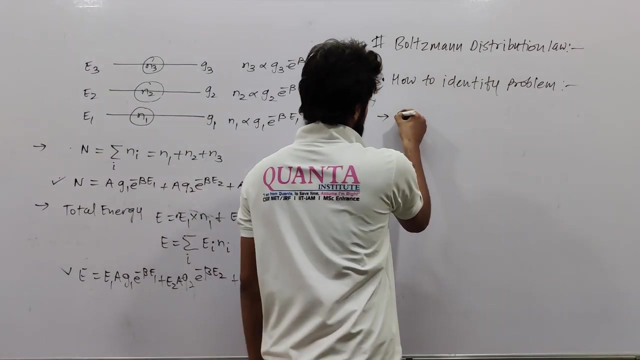 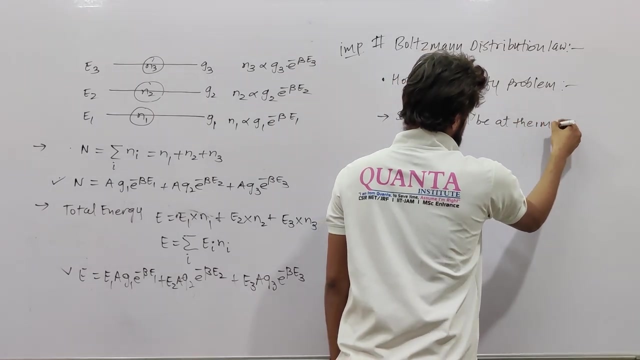 on Boltzmann distribution law. ok, write it all. first of all. there are two points through which you can identify the problem. first, you read the Boltzmann distribution. it talks about thermal equilibrium. so system will be at thermal equilibrium. you can identify from here: system will be at thermal equilibrium. 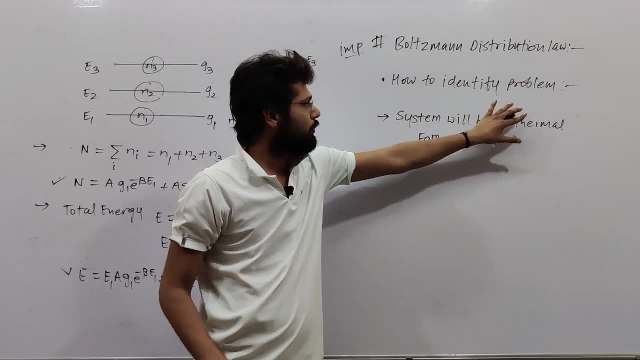 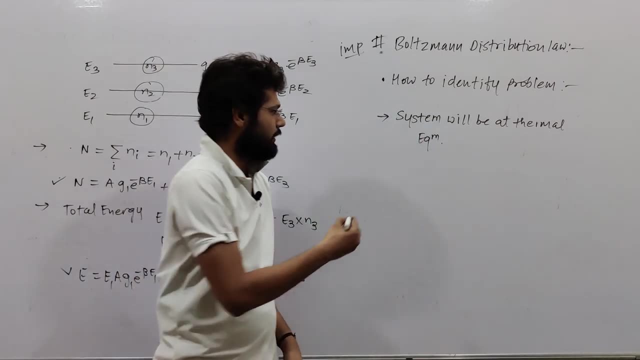 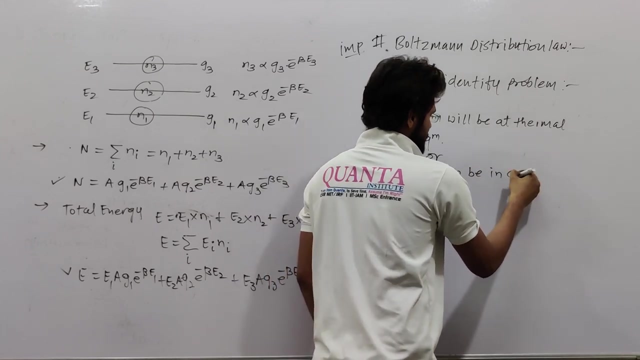 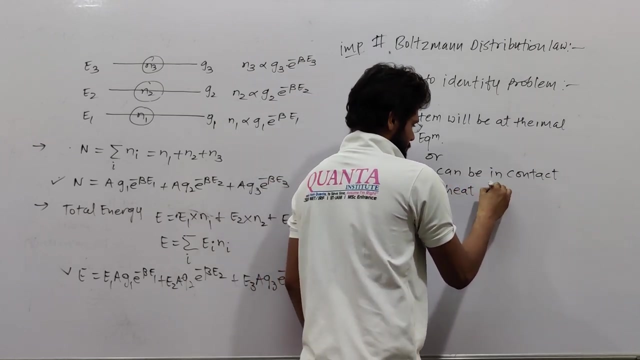 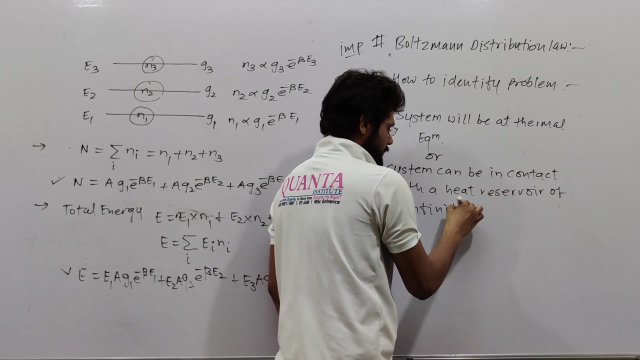 ok, now one thing is happening. this thing is also said in a different way, means in a different way. it can keep the same thing in front of you: how and system can be in contact with a heat reservoir of infinite heat capacity, of infinite heat capacity. it can also be like this: 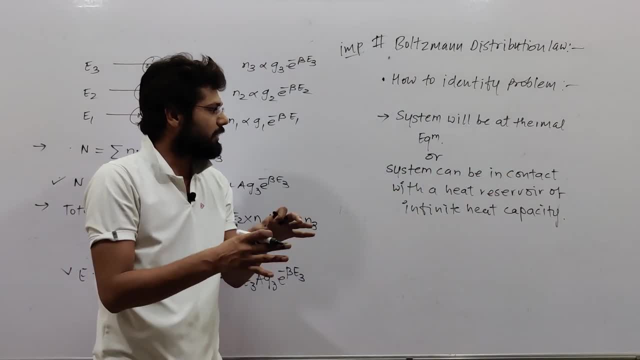 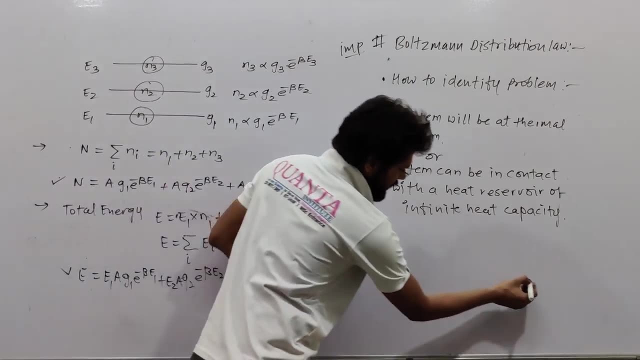 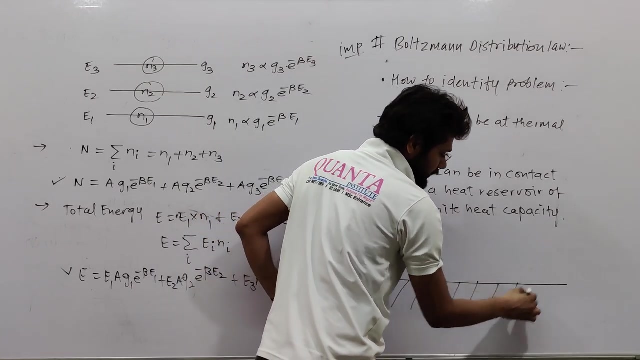 now you explain it properly. if it is in contact with an infinite heat reservoir, then how it became the equivalent of a thermal equilibrium. see what is the situation here: there is an infinite heat reservoir. ok, I will make it like this. what is infinite heat reservoir? let me tell you now. 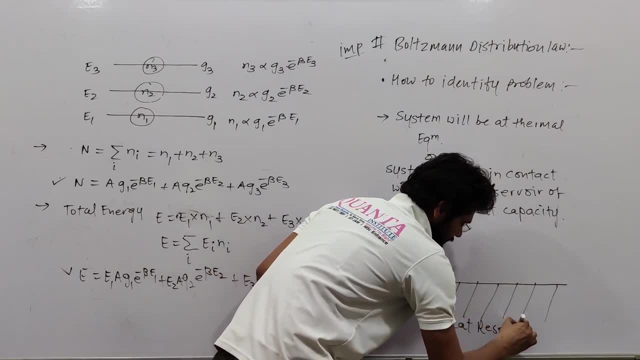 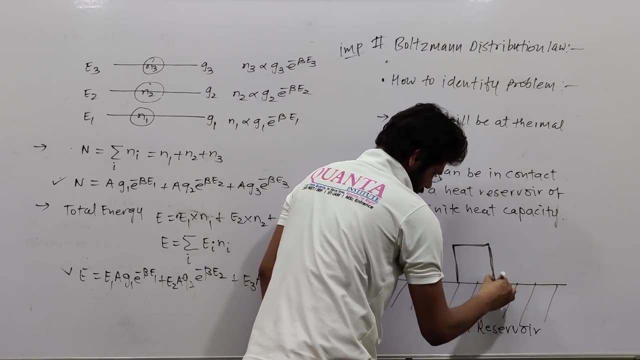 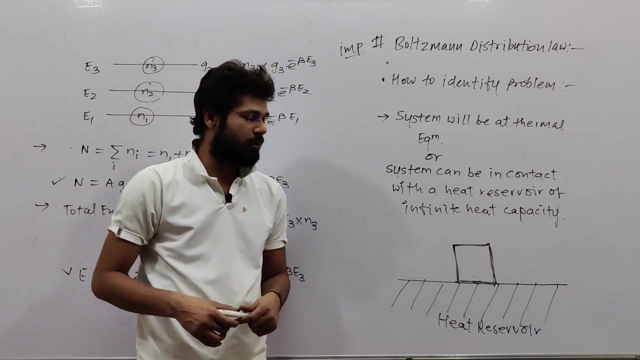 this is a heat reservoir and it is of infinite capacity and your system is in contact with it permanent. you are in contact with it like this: ok, see what is a heat reservoir of infinite capacity? it is like it is a heat sea. what is a heat sea? 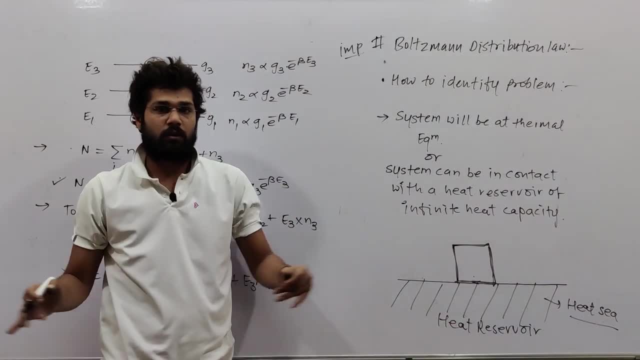 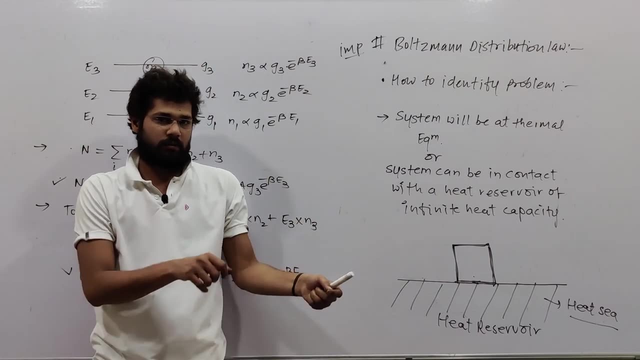 like your water, sea, sea. it is like that. and now in the sea, as I say, if I put some water, one or two buckets, one or two glasses, so does it make any difference on the sea level, on the water level, does it make any difference on the sea level. 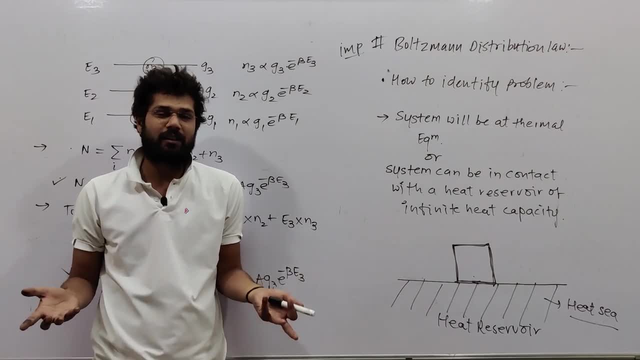 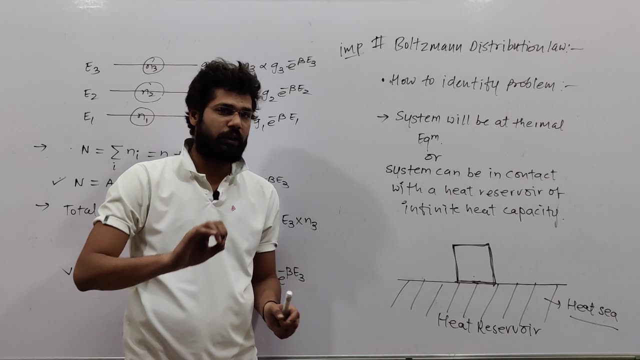 I think no. I think no, what will I do? it does not make any difference, it is a reality. so infinite heat reservoir is also the same. if you put some heat in it, then its temperature level it is at a particular temperature. ok, at its temperature level. 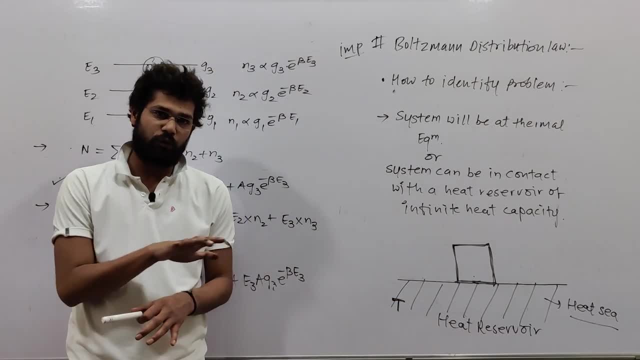 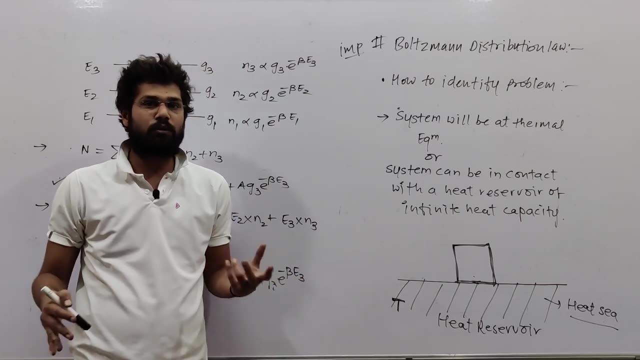 means the water level. here is the temperature level. there will be no effect on it. if there will be some heat in it, then there will be no difference. there will be a little or a lot, like in the sea if you empty 10,, 12,, 20,, 25 tankers. 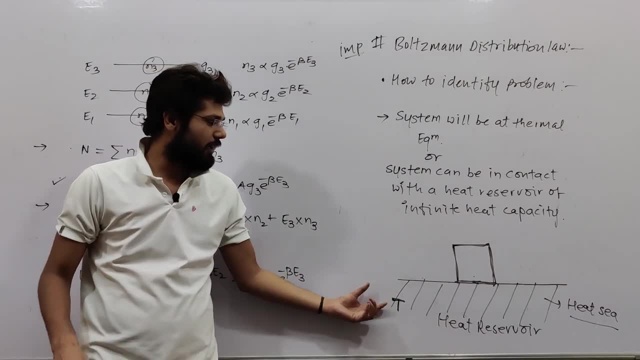 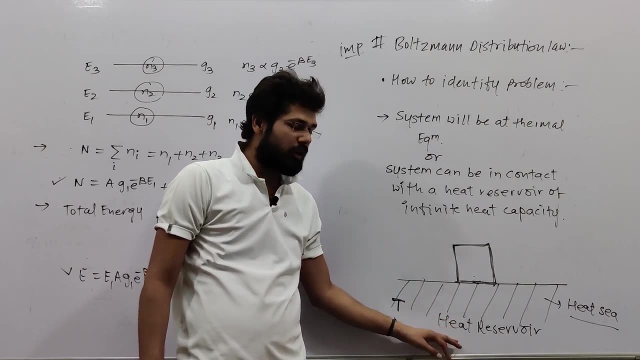 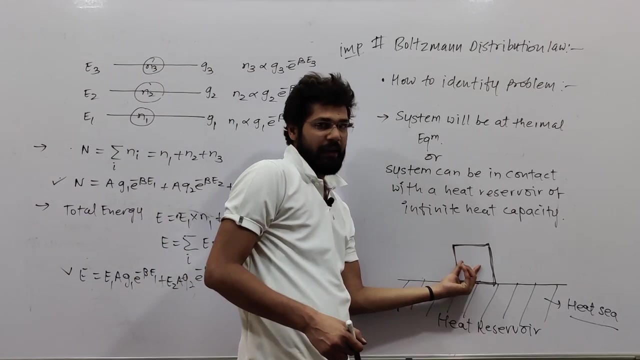 then will the level increase? no, similarly, even if there are many systems here and they are also in contact with it, then there is no impact on its temperature level. ok, how does it stay like this? there is no effect on it. ok, now the system is in contact with it. 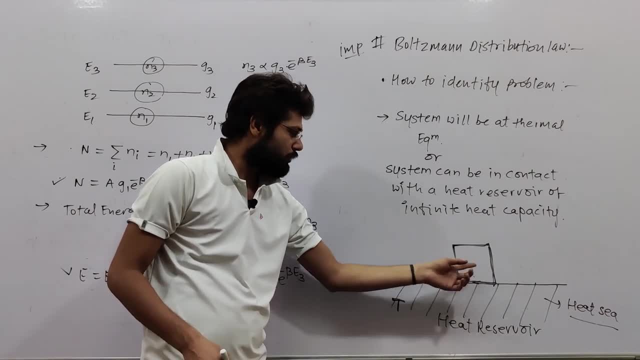 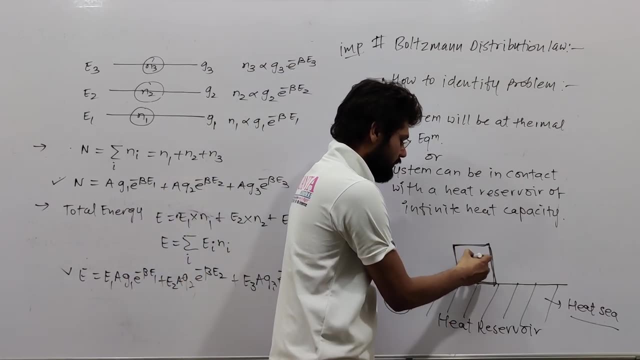 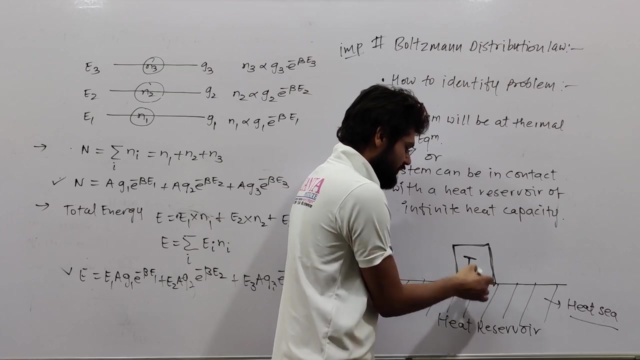 if two systems are in contact like this- this is also a system- then what will happen? it is at T temperature. so what will it do? it will bring it at T temperature. will it set or not? it will do for that. the system will exchange its energy. 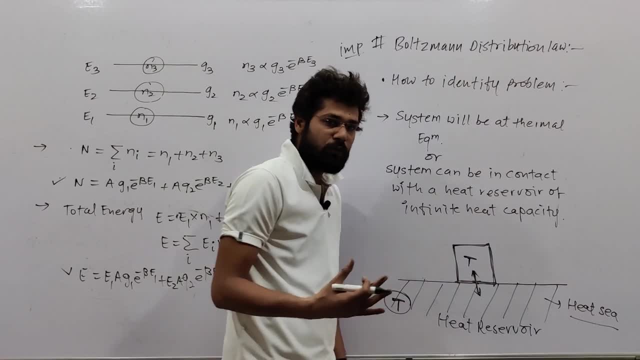 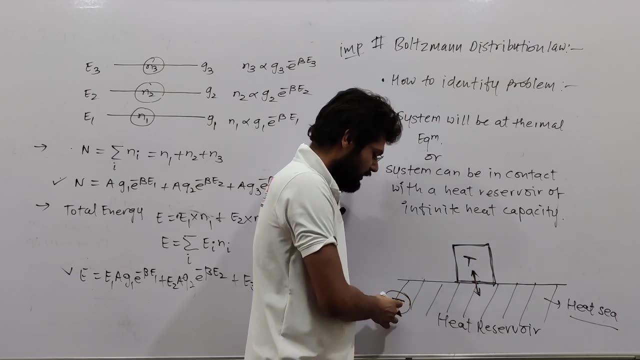 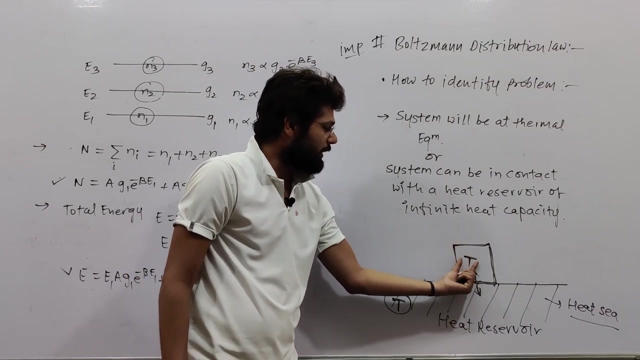 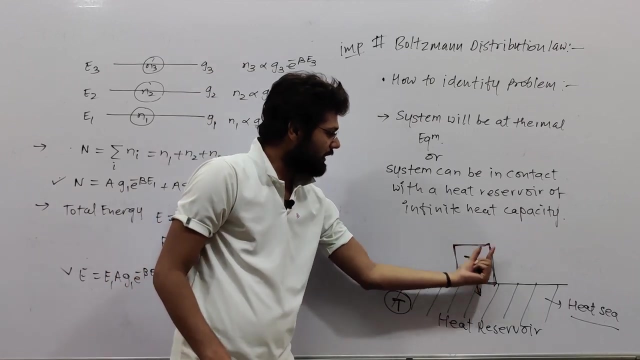 with the reservoir. I will say heat once the extra heat it will share with the reservoir and the temperature will be equal to the temperature of the reservoir. ok, ultimately, I can say that here: T after some time the temperature will be T permanently. ok, and now the temperature of the system. 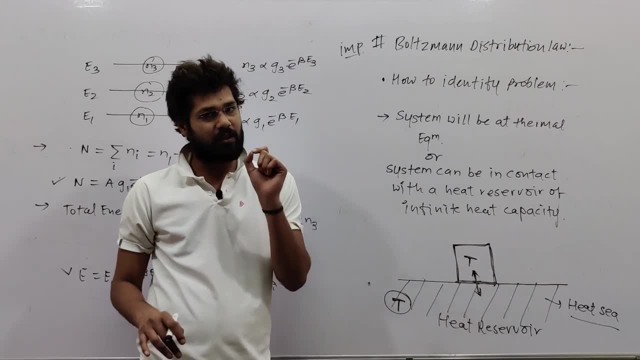 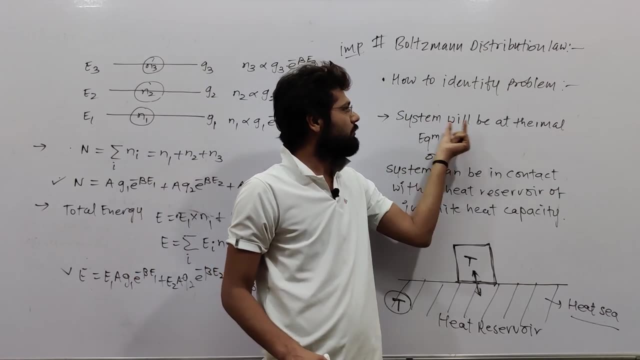 is permanently T. it means the system is at thermal equilibrium, ok or not? so this situation, it is also equivalent to this thing: the system will be at thermal equilibrium. you can also say this: the system may be in contact with the heat reservoir of infinite heat capacity. 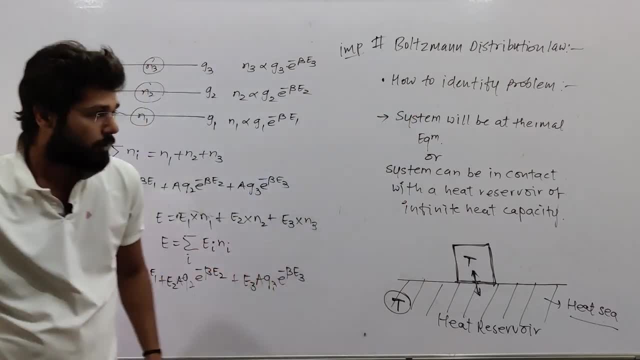 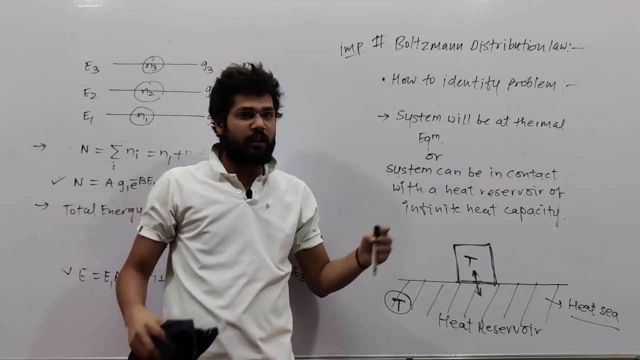 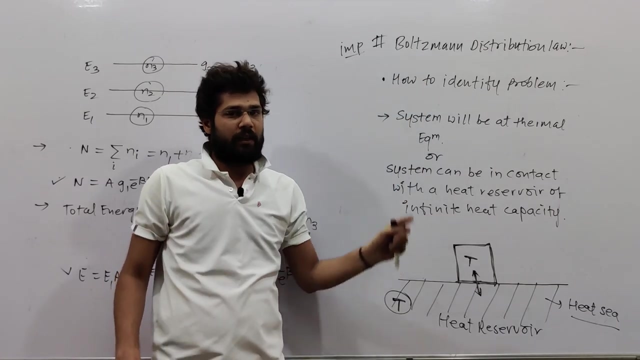 ok, ok. so this type of language can be plus. now, one thing which is special is that you get so used to this language that you- I mean you- stop thinking that it will be a question of Boltzmann distribution. why, see, how do you get used to this language? 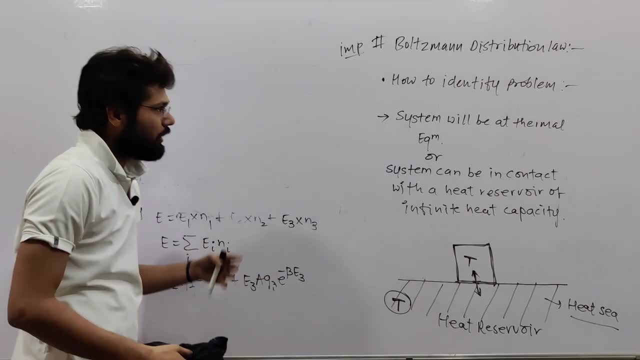 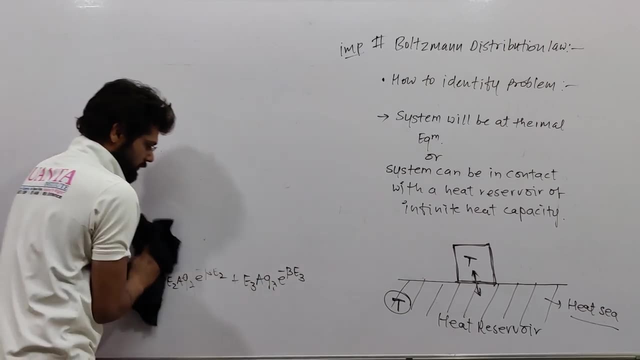 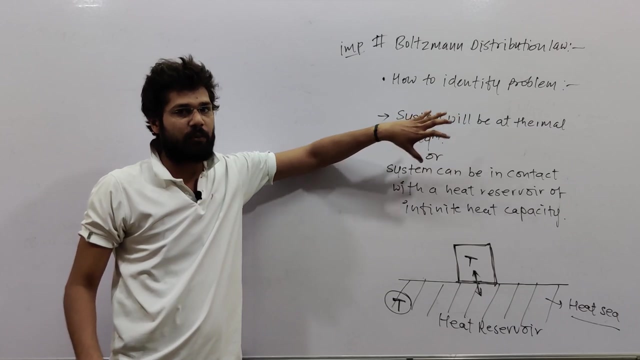 from what is written here. you get used to it and you don't think about Boltzmann distribution. how do you get used to it? see that thing. so this is not a sufficient hint in the question if I say, if it is written just thermal equilibrium. 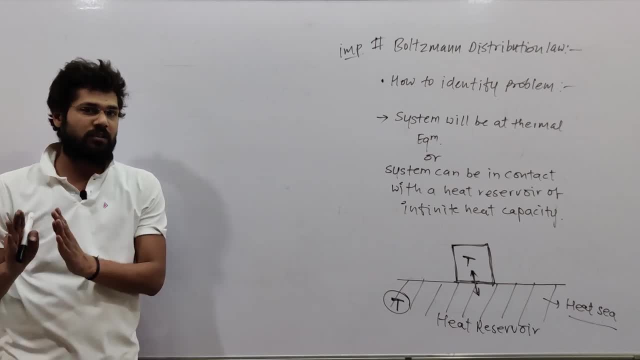 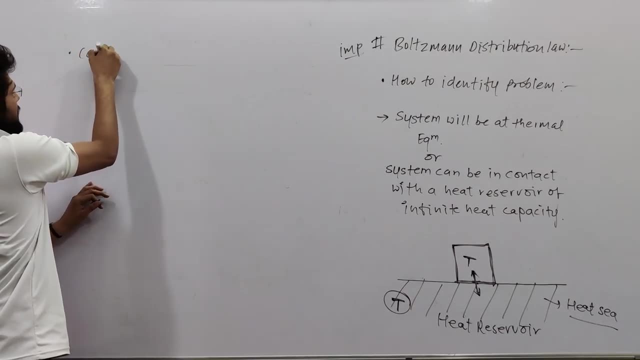 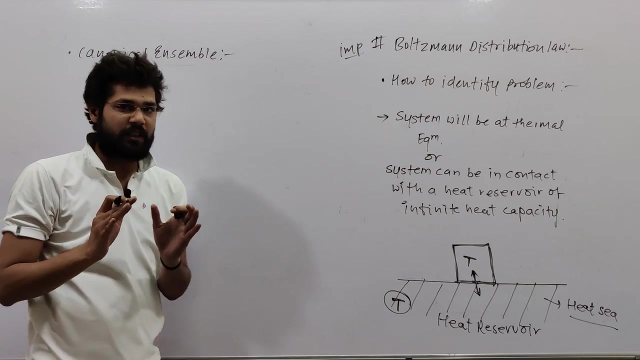 then you should think about Boltzmann distribution. but the question of Boltzmann distribution is not sure how in your future. in your future you will read canonical ensemble and the fact is that the 50% part of the stat- I mean if there are 35 lectures on stat- 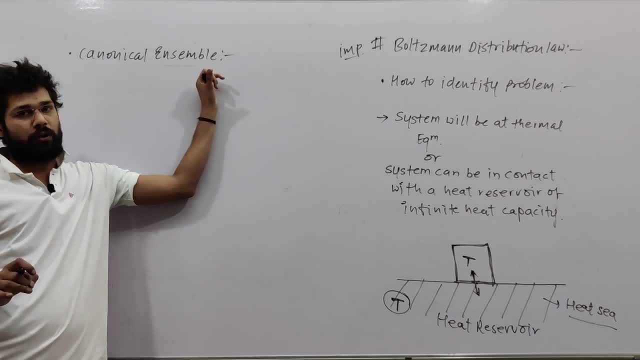 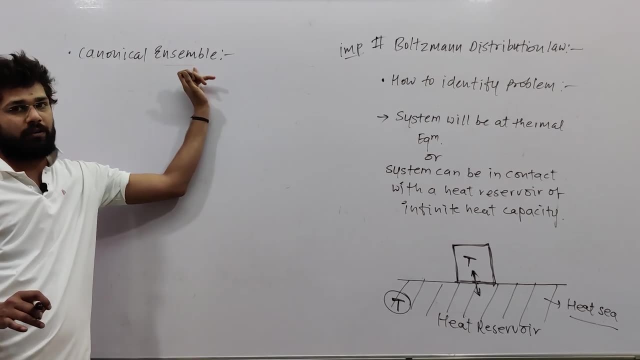 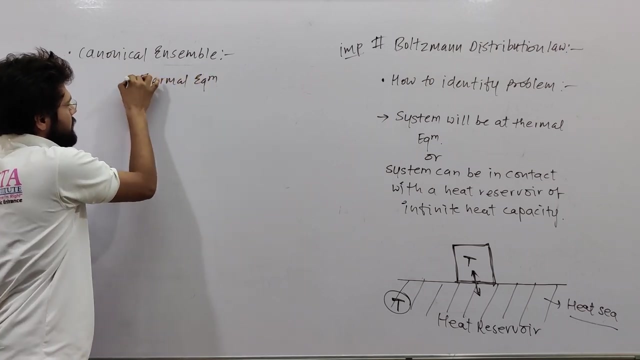 then around 12 lectures will be on canonical ensemble. ok, if you have solved 500 problems, then 300 will be on canonical ensemble only. ok, I am saying, and in canonical ensemble the system is always at thermal equilibrium. ok, always at thermal equilibrium. so by doing questions of canonical ensemble, 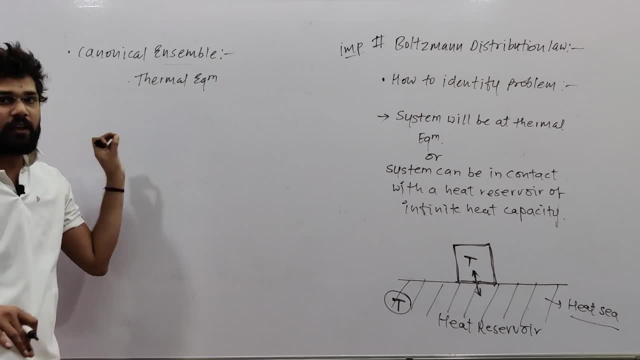 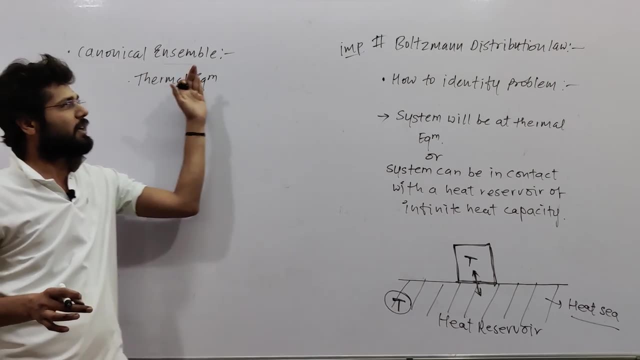 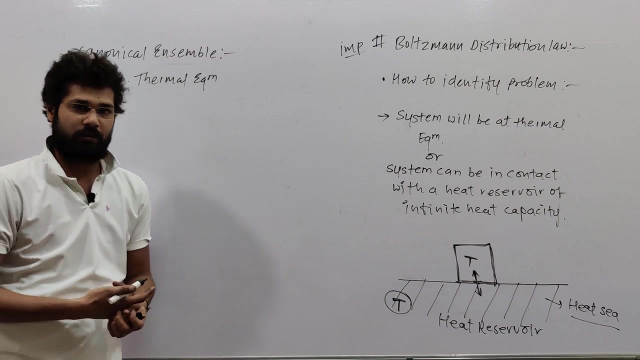 you become so habitual to look at thermal equilibrium in the language of the question that the first image that is created is of canonical ensemble, not of Boltzmann distribution. so now what happened? this is not sufficient. there should be a second hint, absolutely correct. so what is the second hint? 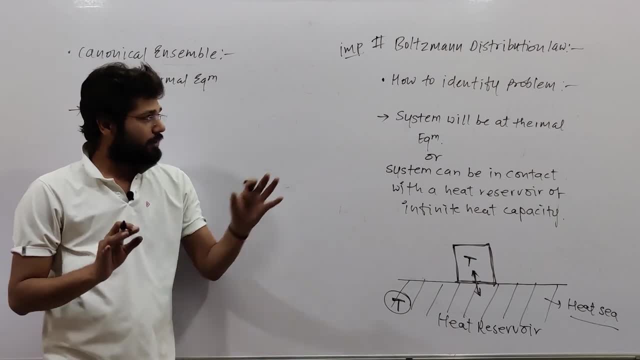 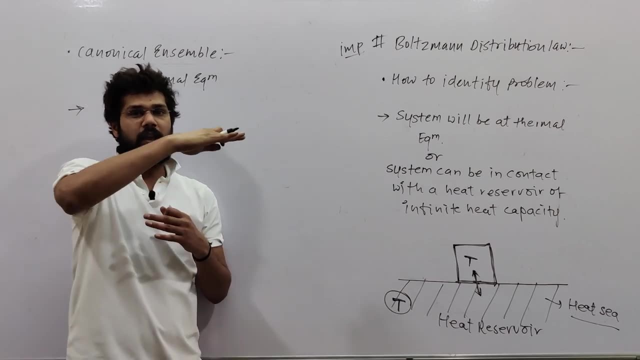 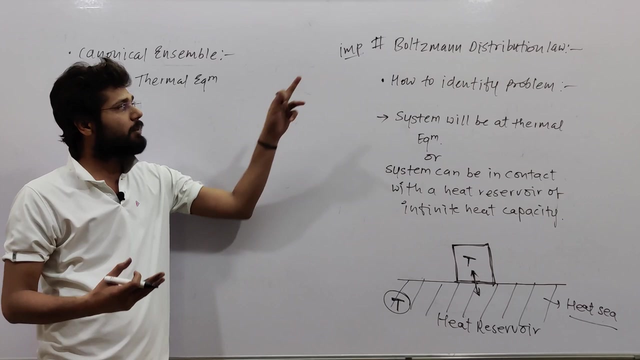 second hint is that see what Boltzmann distribution law tells. that how means what it tells: average number of particles in a level. so whenever there will be number of particles in language of question, then you have to think about Boltzmann distribution law. ok, so the second hint is: 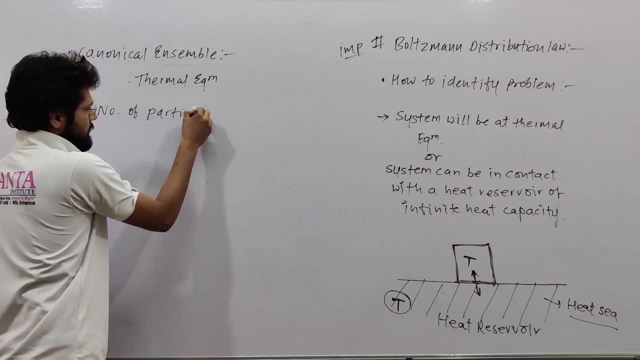 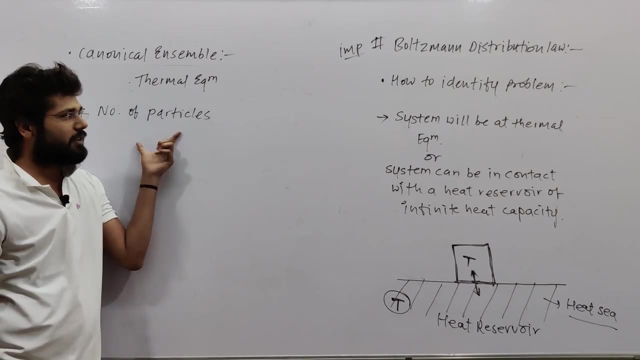 number of particles. language of problem will contain number of particles, correct, and this is a very important thing. as soon as you see this, you have to go straight here. and the two that I told you that you can write total energy. like this, you can write total energy. 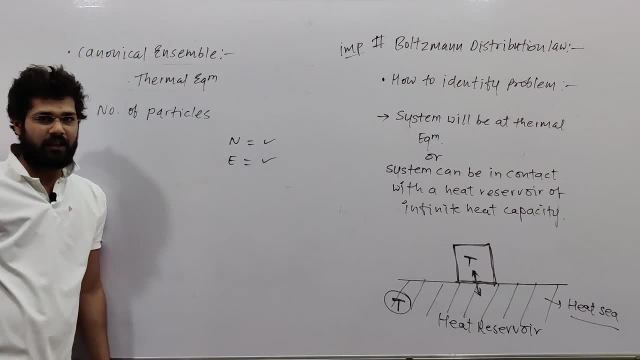 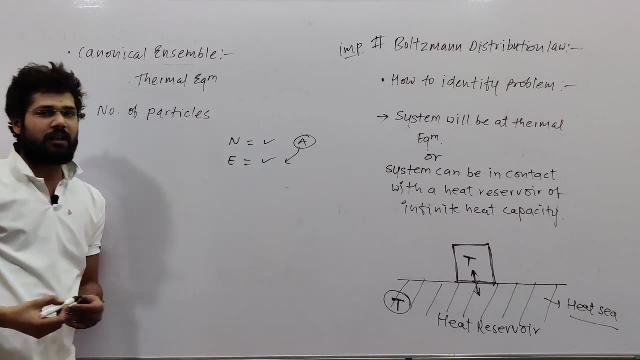 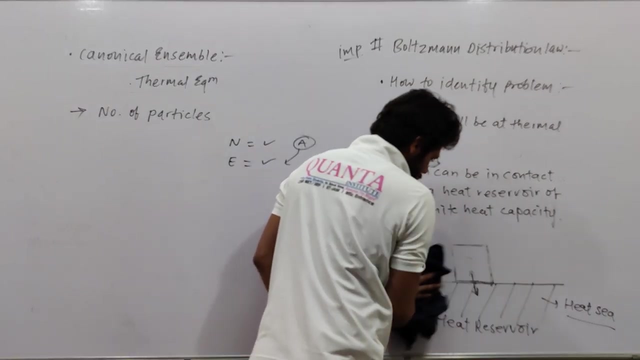 like this: if nothing is happening to you, then write that. ok, sometimes what you have to do is find out A from here and put it in this. like this: there are many operations which you have to do. ok, now let's move to the next topic. next is your. 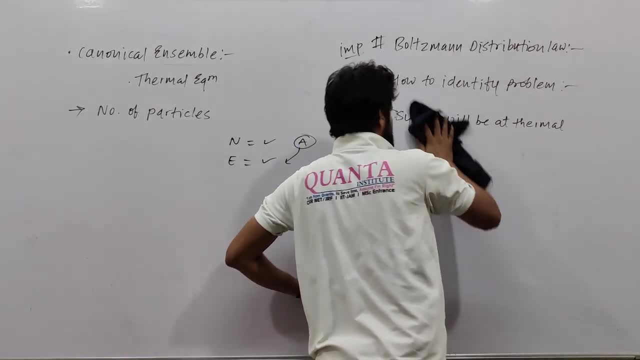 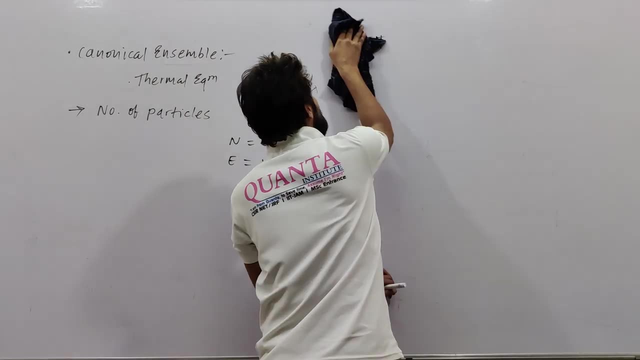 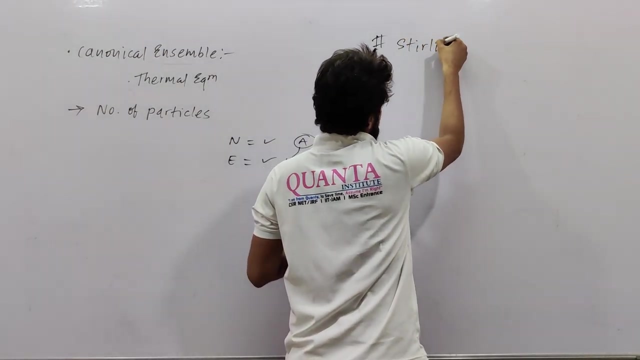 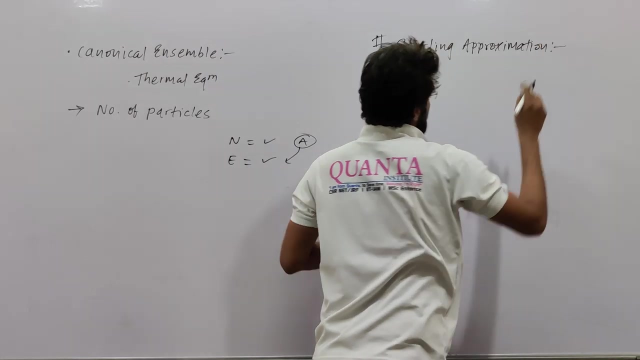 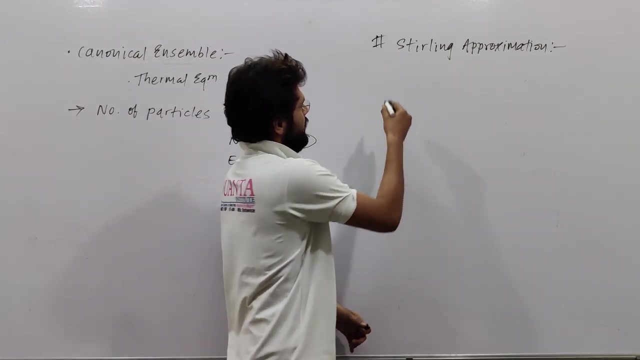 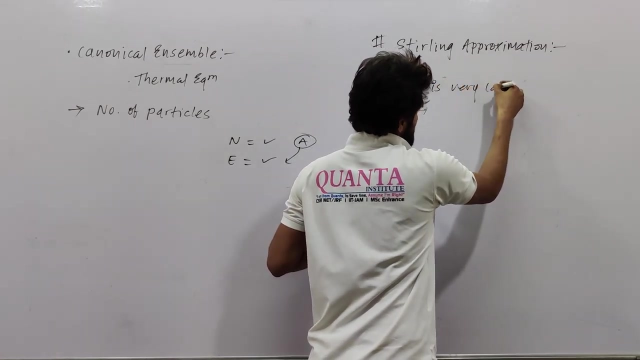 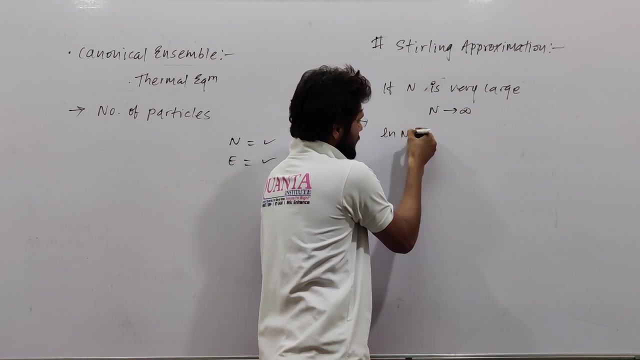 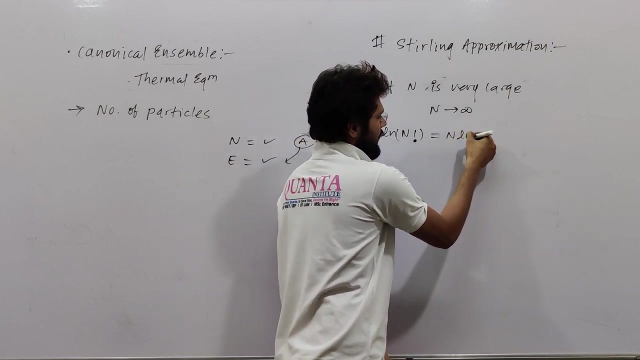 sterling approximation. sterling approximation, this is a mathematical term, this is a mathematical approximation. see what happens if n is very large. if n is very large means n tends to infinity. then then what will happen? that you ln n factorial, ln of n factorial, you can write n, ln, n. 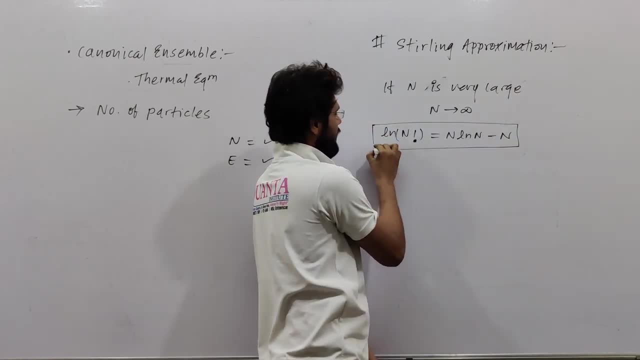 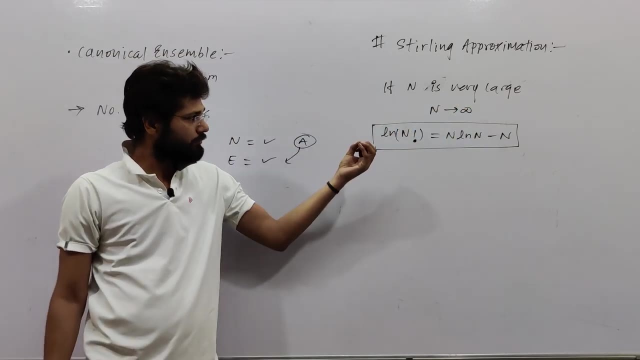 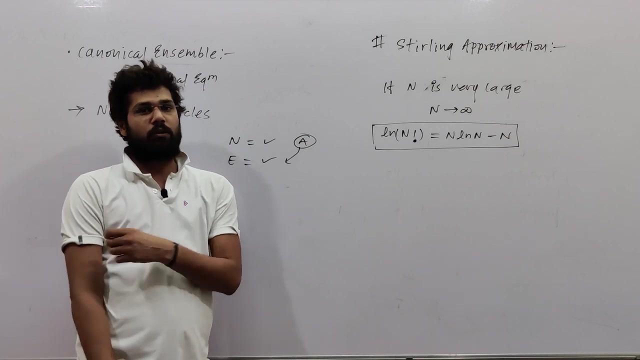 minus n, and this is sterling approximation and this is applicable only then when n tends to infinity and you know that in this stat n number of particles is there. and generally, what is the number of particles in this stat? around 10 to the power of 23. 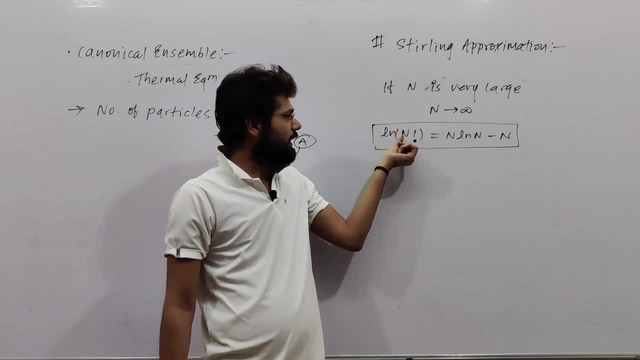 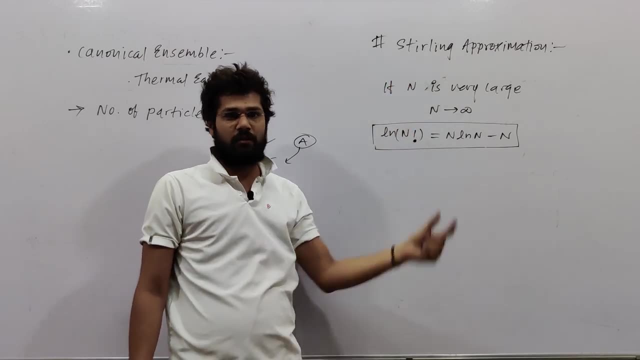 so this is a large number. so in this stat, if n number of particles is there in this type of situation, then this can be applied and that's why we are discussing it here. ok, it was already mathematical, but we have discussed it now, ok. next topic is: 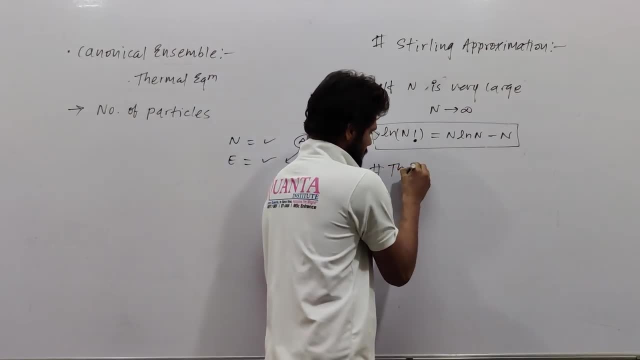 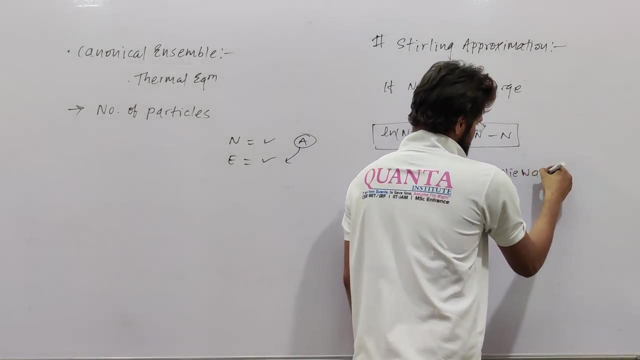 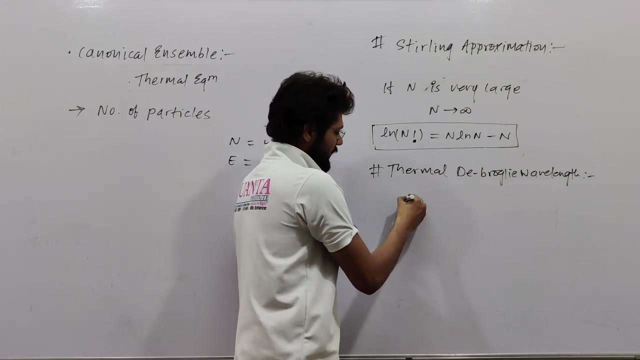 thermal de Broglie wavelength. thermal de Broglie wavelength. thermal de Broglie wavelength. you have seen this also in many places. you will get to see and you should know what it is. let's denote it by λth. λth and this is h over. 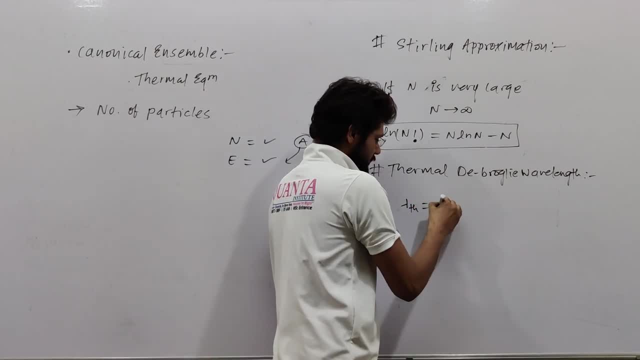 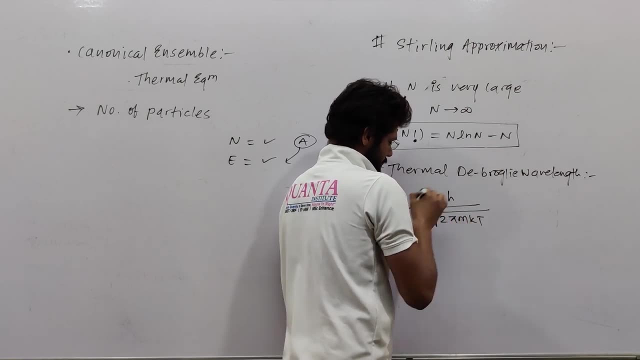 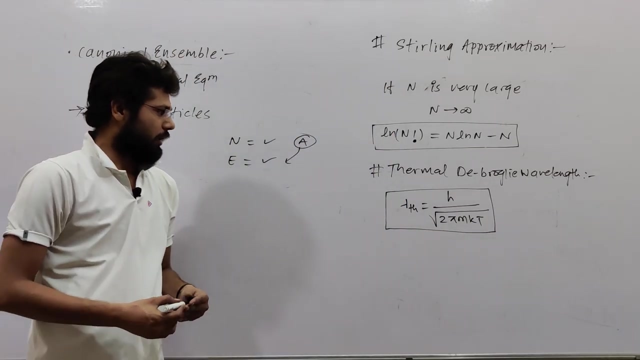 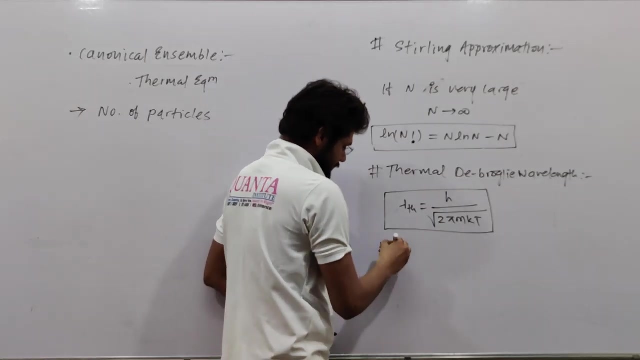 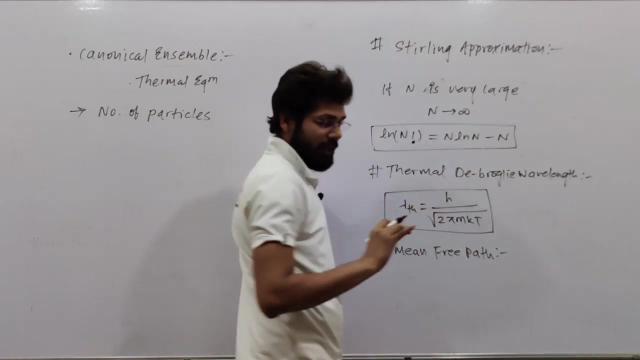 under root 2 π mkt and this is h over under root 2 π mkt. ok, This is thermal triboglic wavelength. and next let's talk about mean free path. you can also get to see this sometime. mean free path. what happens? see? this is denoted by lambda. 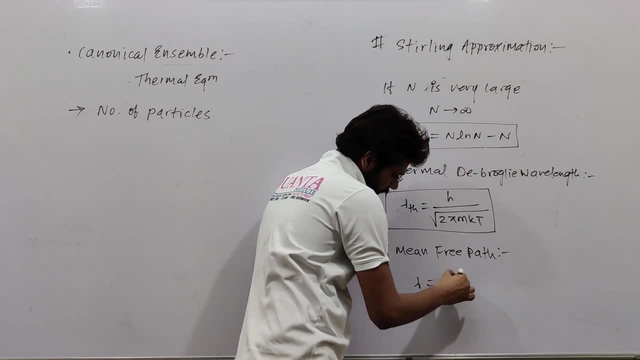 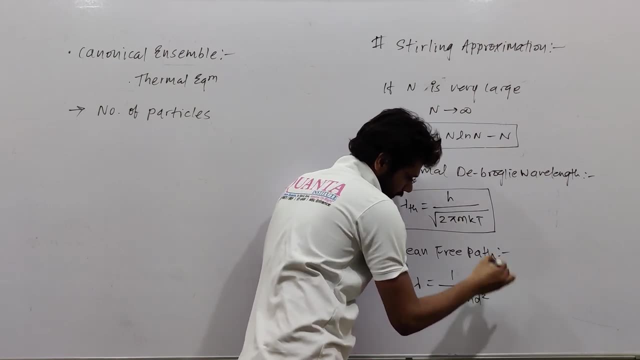 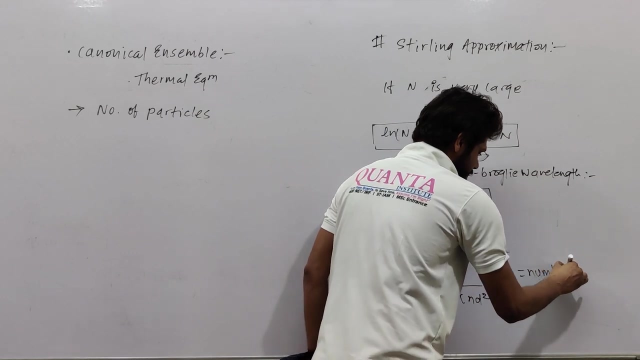 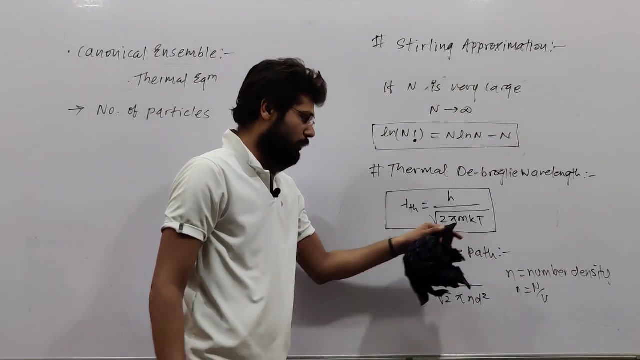 just lambda. and this is 1 over root, 2, pi, n d square. what is n here? n is your number, density. what is the number density? n is n by v, number of particle divided by volume. d is here diameter of the volume. 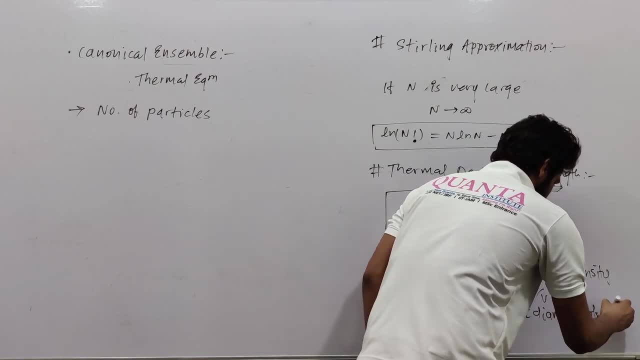 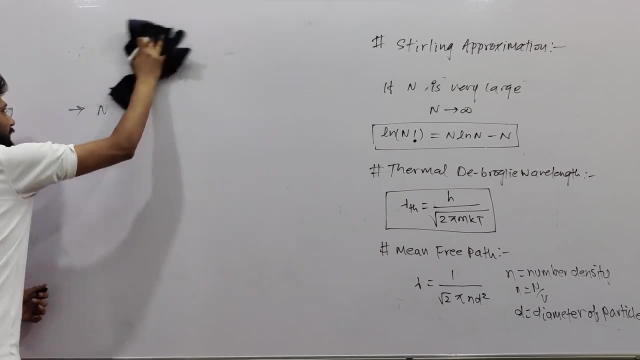 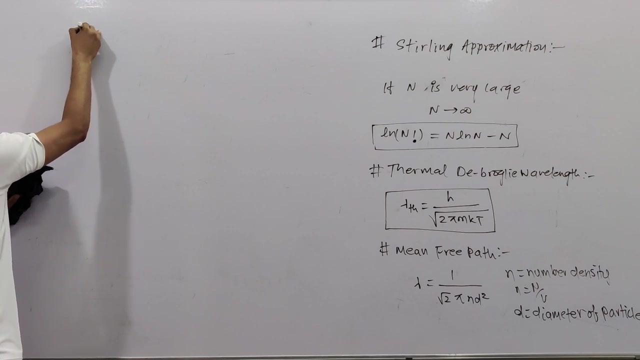 Particle diameter of particle diameter. okay, so whatever your particle is, its diameter is now see what happens. give a feel. mathematically it is okay. see the feel. this is your system. this is your number of particles. various number of particles are there in your system. 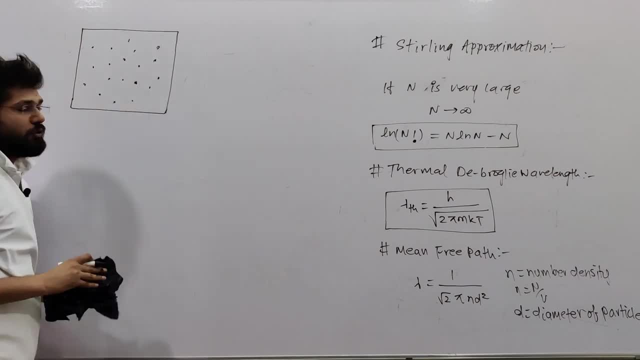 10 of them matter and if we increase this then derives 0 to t or max of b. Yes, now see what happens. this is your number of particles. Give quand yur per binary how it will distribute. what you will get in the mind will also become. 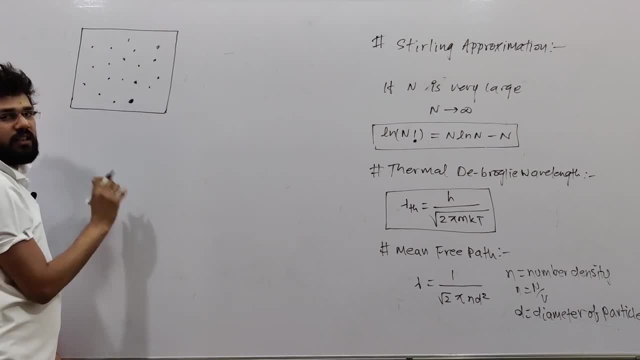 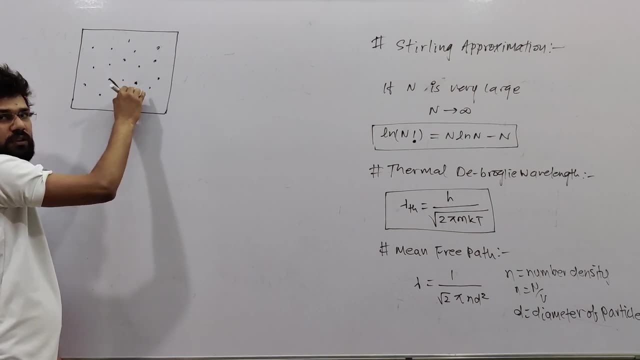 equal. See here: this number of particles is given to me by the rules. these 5 rows has e to 500 rr. and what doing like what now? so this is the Denis of be what value the some randrverso1.h2 function. 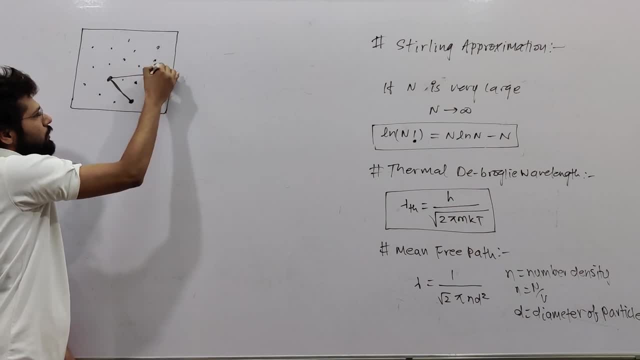 after that it will deflate from here and go somewhere here. and if there was a particle here, then it collided with it. then it went here and collided with the wall. then it went like this and collided with this, then it went here. and if there was a particle here, 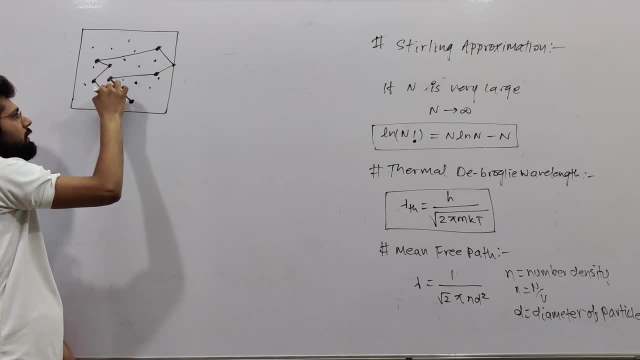 then it went like this: this is how Brownian motion works, is it correct? now, one thing: you have noticed that while doing Brownian motion, while doing collision, sometimes it has to go this path, sometimes it has to travel this path, sometimes it has to travel this path. 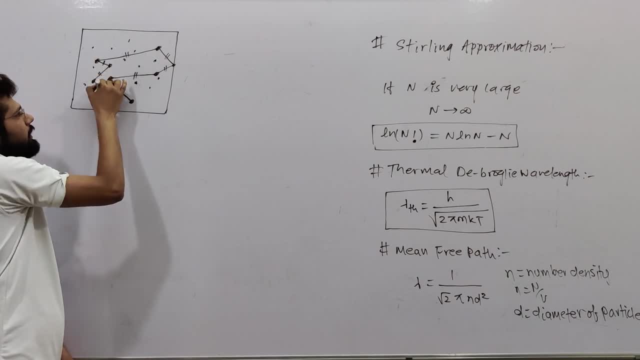 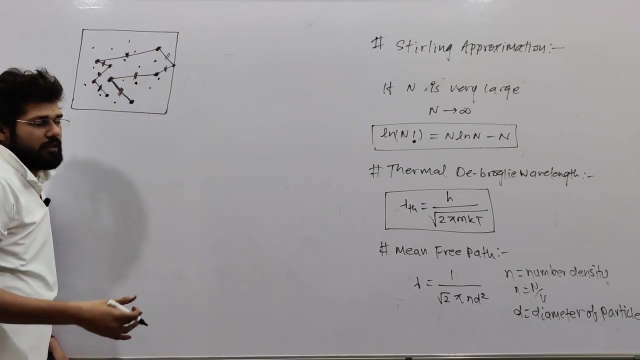 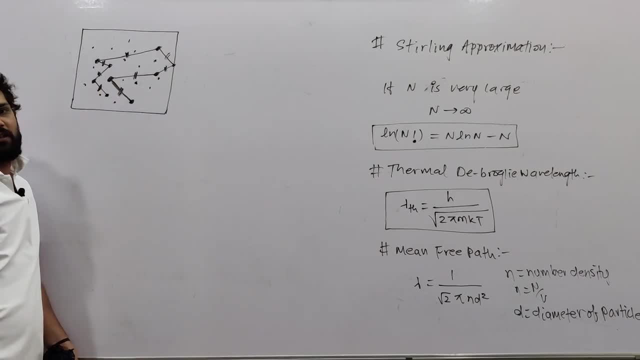 because the particle is free for so long there is no collision with anyone. that is why it is called free path. so I can say it like this: that the mean distance, the average distance, lambda is. what mean free path is lambda. mean free path is average distance. 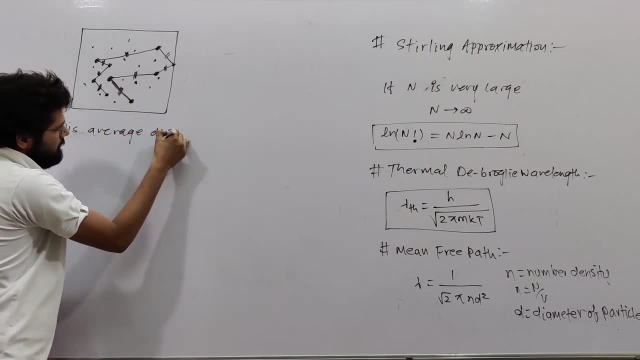 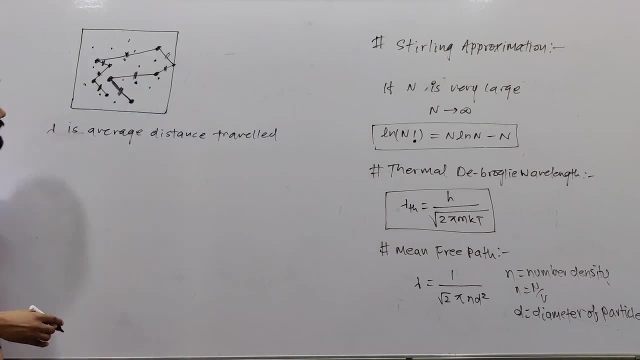 average distance. so is it targeting these points? 됐ع so like that, you have to keep all division okay, but it sinking just one thing as long as make a doing collision. just take time for that. now let me ships, let's take Bigfoot. so after: 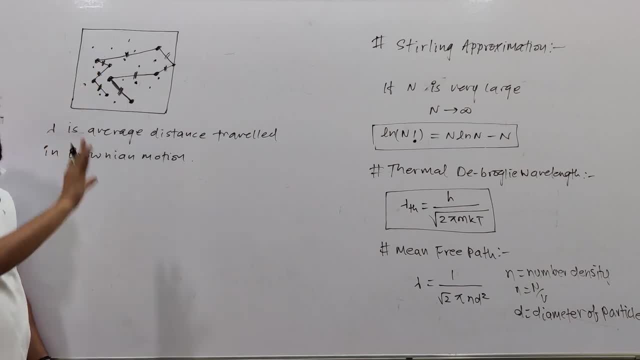 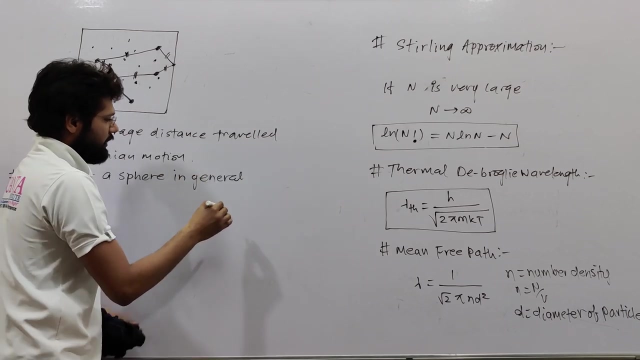 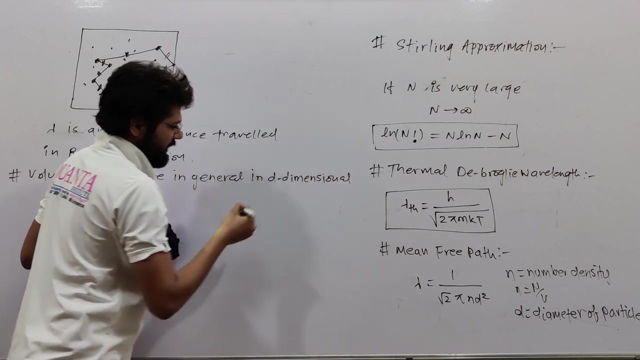 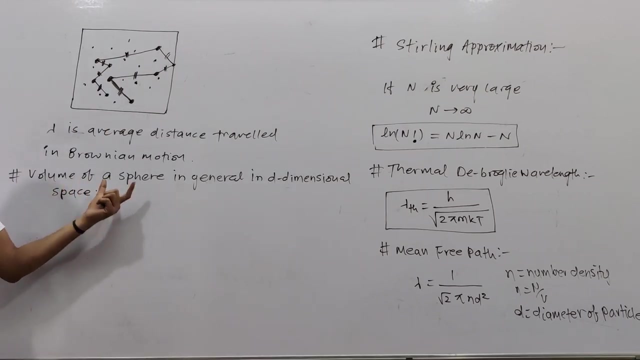 distance travelled in Brownian motion. You must have understood this. This is the mean free path. Next topic is general volume of a sphere in general, d-dimension in general, in d-dimensional space. In d-dimensional space there is a d-dimensional space. What will be the volume of a sphere in that? What will be the general? 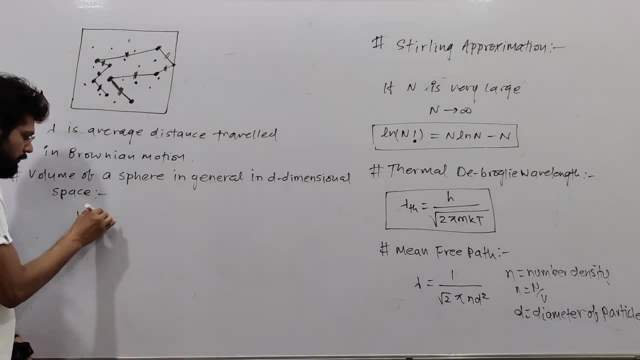 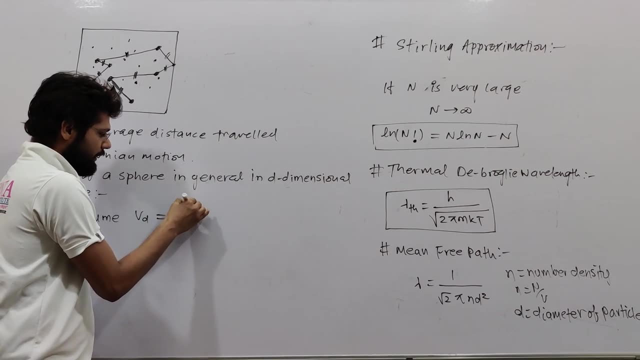 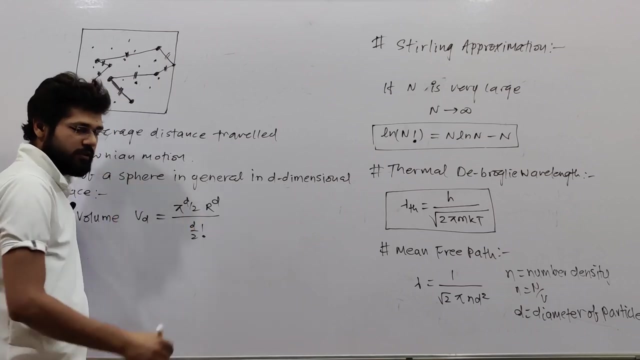 volume. So its formula is volume. we denote it with d because we are talking about d-dimension, and this one is pi d, Pi, d by 2, r d and d by 2 factorial. This is the formula of volume. Now, you are not. 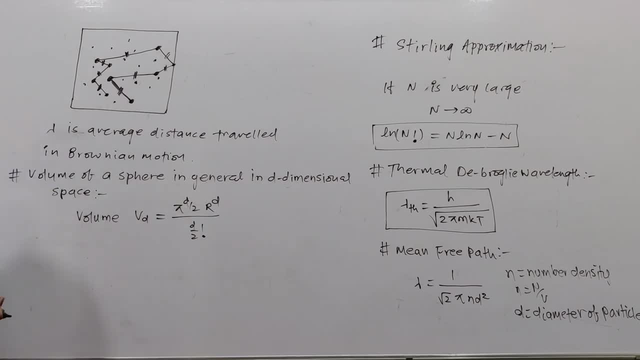 believing that it is a formula of volume. How will you believe If I talk about it in 3D. what is the formula of volume of a sphere in 3D? In 3D, the formula of volume is 4 times. 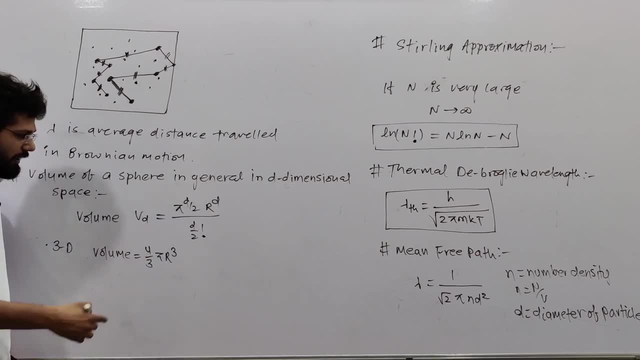 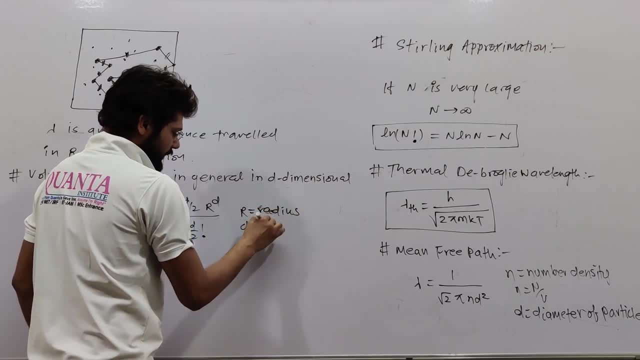 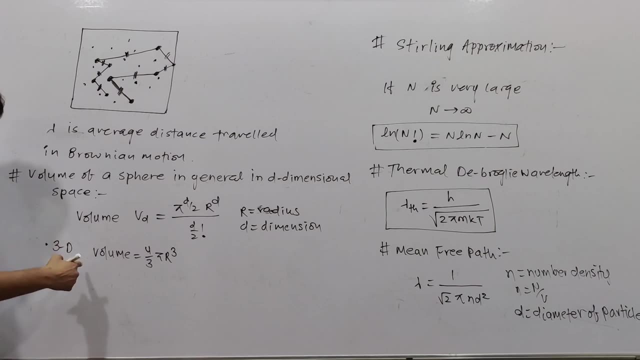 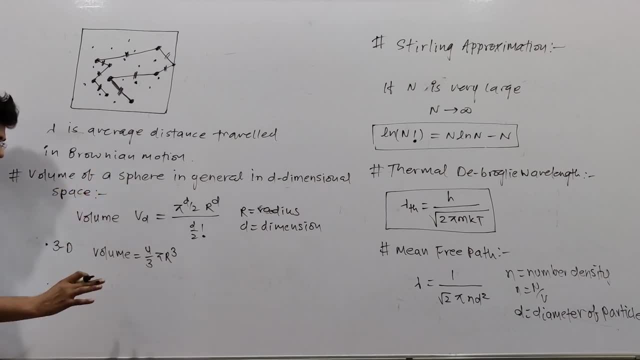 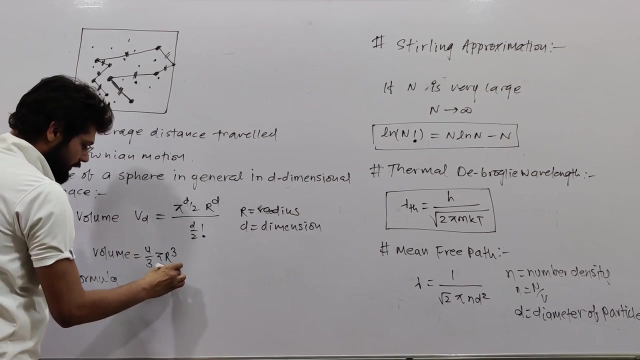 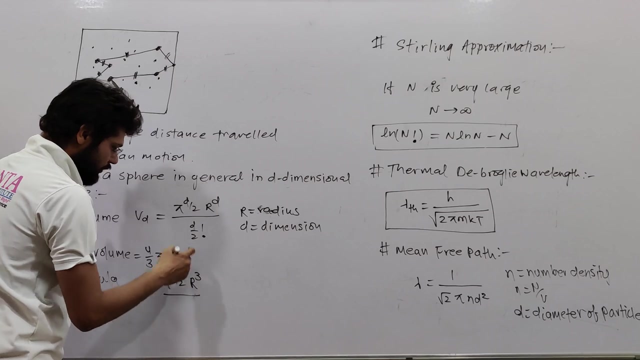 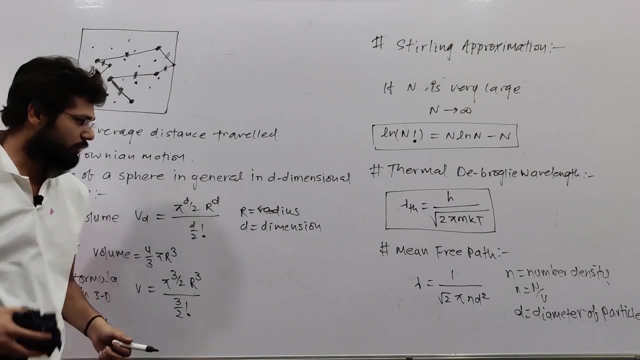 volume of a sphere in 3D. one will believe that I am right. this formula is correct, absolutely correct. What's the formula in 3D? p, r, log, f, e in 3D. In case of 3D, what will be your V equal to V- I have not written D. okay, the power of Pi is 3 by 2 because D is equal to 3, you are talking about 3 dimensional space. the power of R is cube below- will be 3 by 2 factorial. now, how to solve the factorial of 3 by 2, see, think I will erase it. 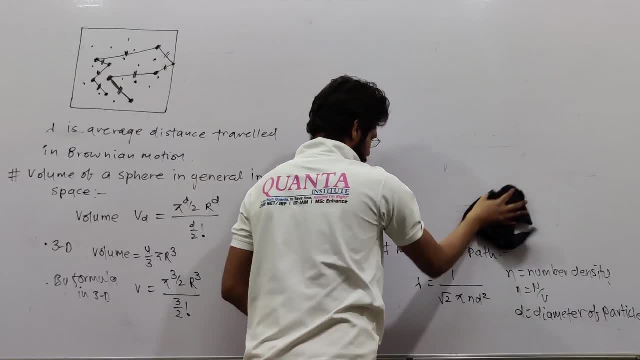 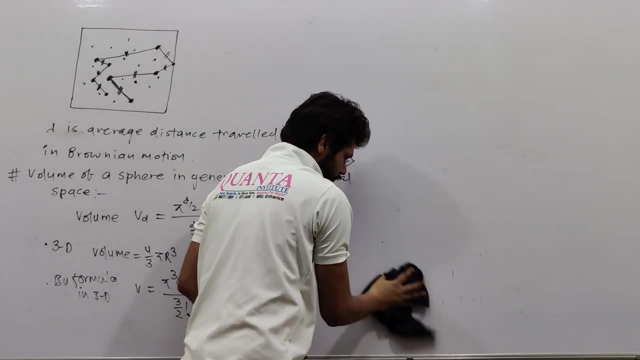 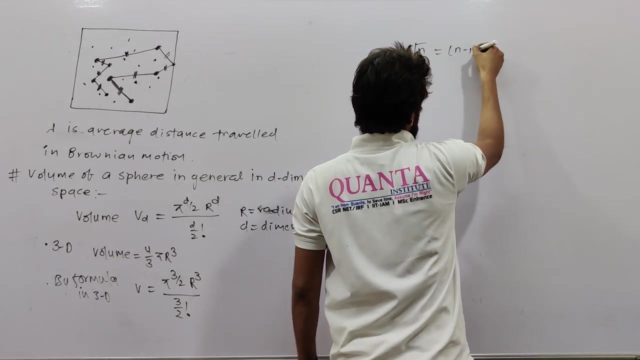 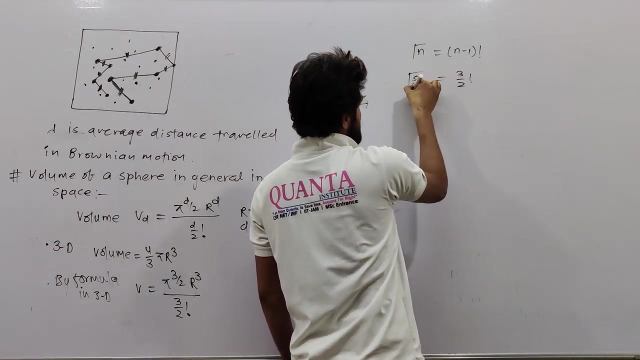 3 by 2 factorial will be solved. see now you know what is gamma n, factorial of n minus 1, so 3 by 2 factorial will be. can I write gamma 5 by 2 or not? can I write? so see what will be V. V was. 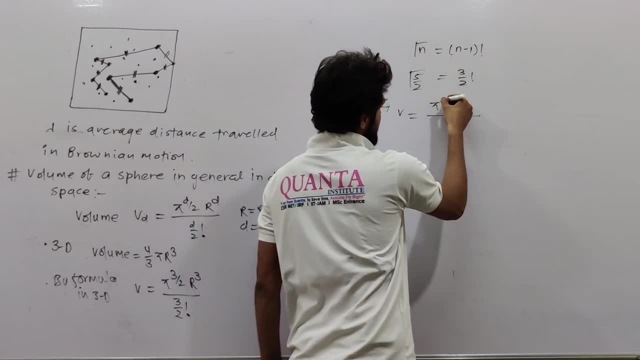 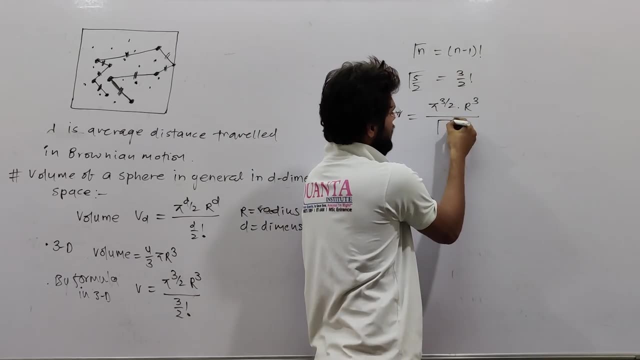 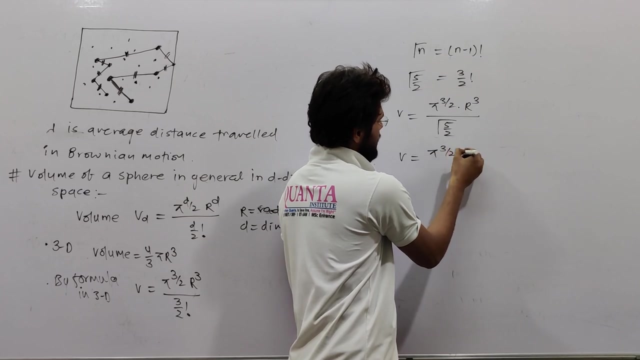 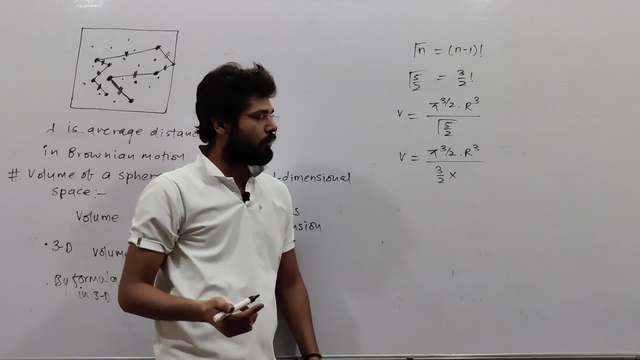 Pi's power 3 by 2, Pi's power 3 by 2, R's power cube and 3 by 2 factorial, 3 by 2, factorial. I will write gamma 5 by 2, okay, now gamma 5 by 2 will be solved. see how much will be Pi's power 3 by 2, R cube. gamma 5 by 2 is what 3 by 2 into 3 by 2, gamma 3 by 2 and gamma 3 by 2 is what half into gamma half. gamma half is what 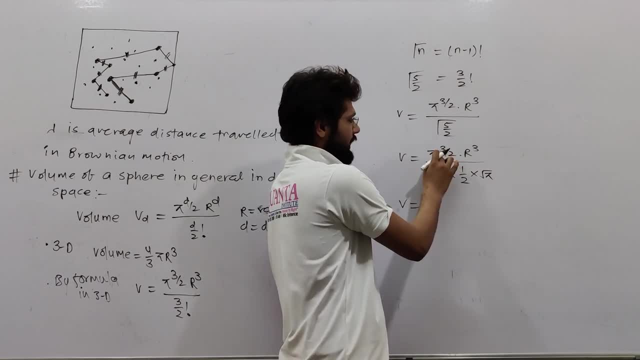 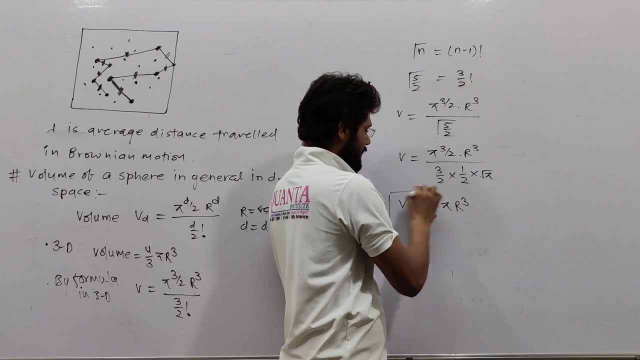 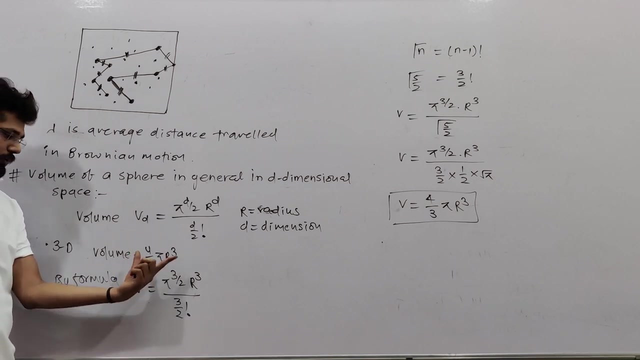 root Pi. so what will be? here Pi's power, 3 by 2, here, root Pi, Pi's power is half, so half will be left. Pi will be left above. okay, below this is 3, 4 will go above 4 by 3. Pi R cube, is it done or not? so in 3 dimensional space, by formula also, you are obtaining the same result which you already know. this means this formula is correct. so now I will box up. 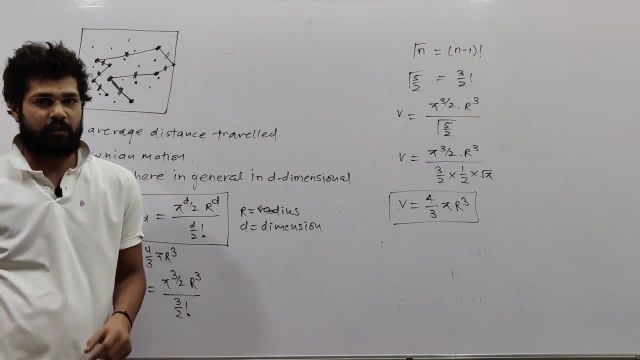 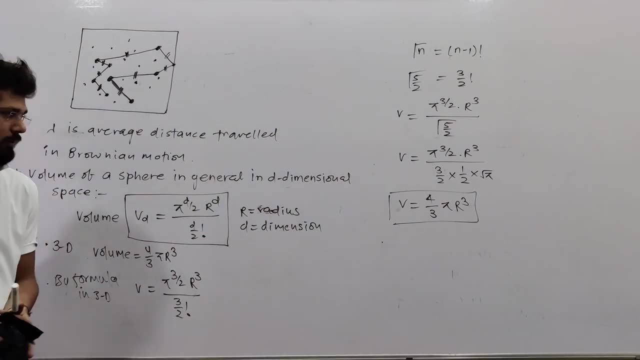 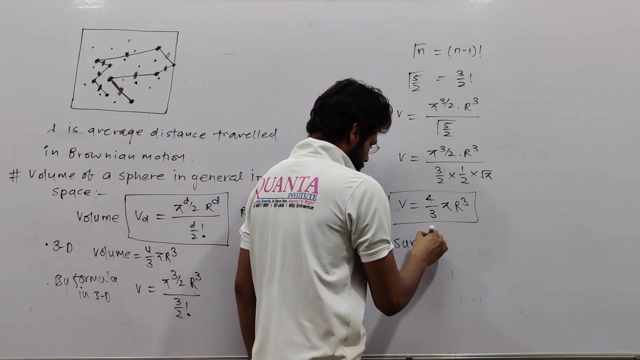 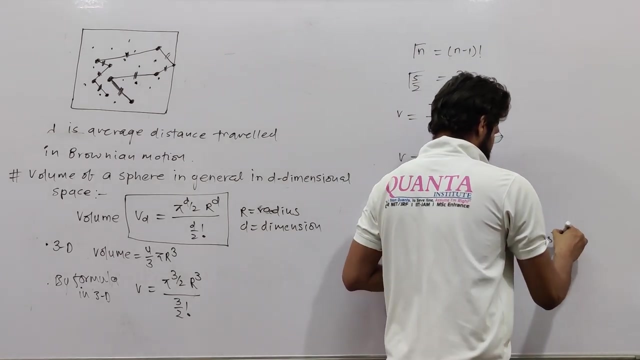 that in d dimensional space, volume is written like this: you will need this somewhere. okay, let's talk next. okay, volume is done. surface area, although surface area is not needed, but still, let's tell surface area in d dimensional, in d dimensional space. see what will happen. 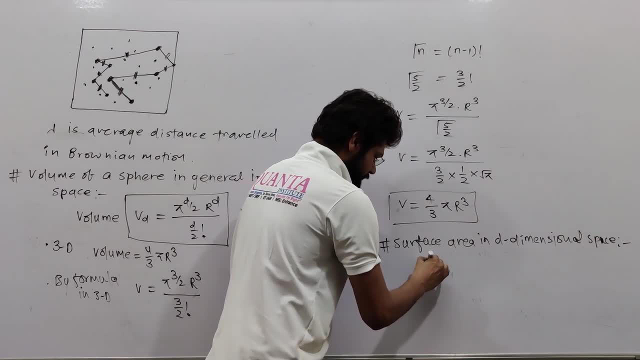 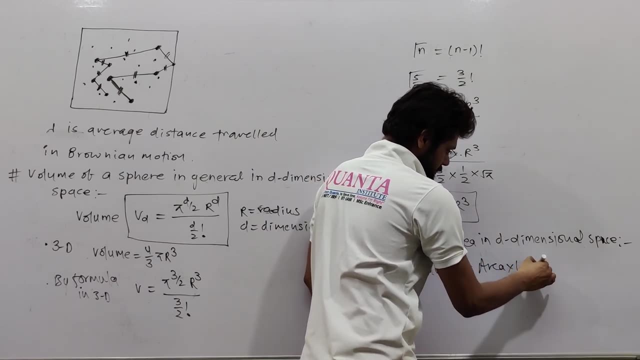 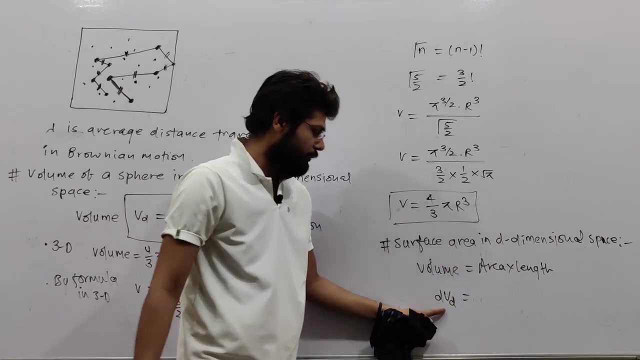 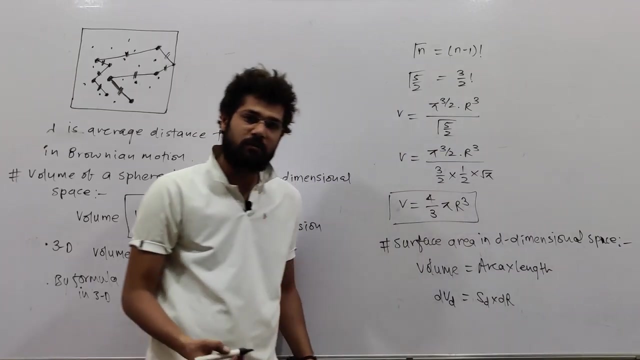 now you know what is volume: area into length, area into length. okay, so the volume in d dimensional space, an elementary volume, dvd. I can write it like this: that surface area into length means dr radius, is it correct or not? 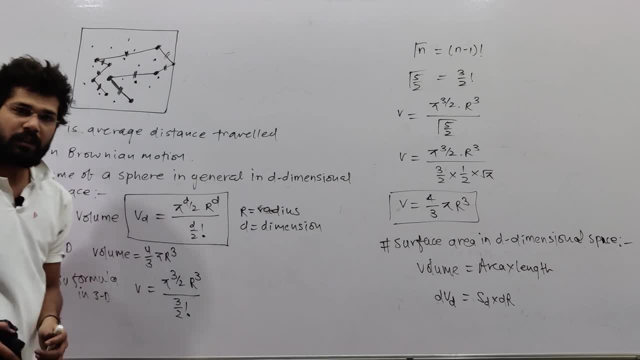 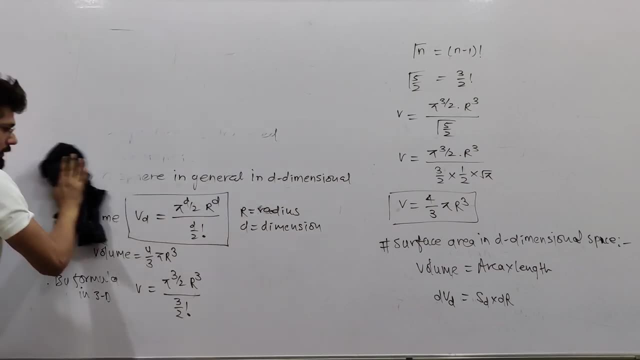 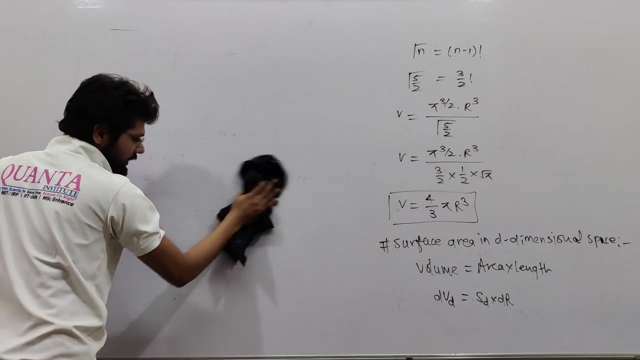 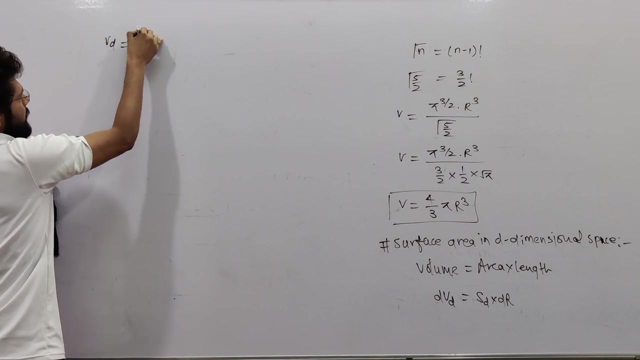 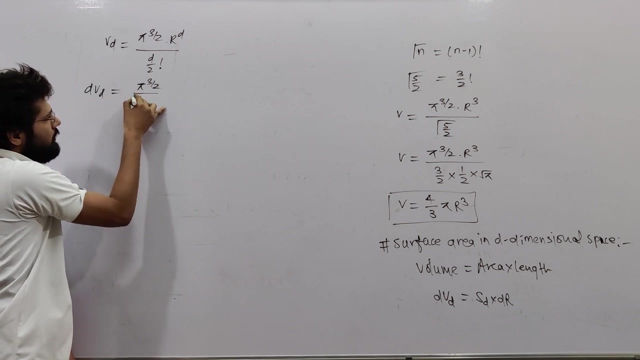 and compare it with this relation test will be found out. let's do it. what is vd? what is vd volume in d dimensional? since vd is Pi's power 3 by 2, and R's power d d by 2, factorial. so what will be dvd, dvd? dvd will be Pi's power 3 by 2, and this one is constant. so you keep it as it is: d by 2, factorial. okay, R's power d. 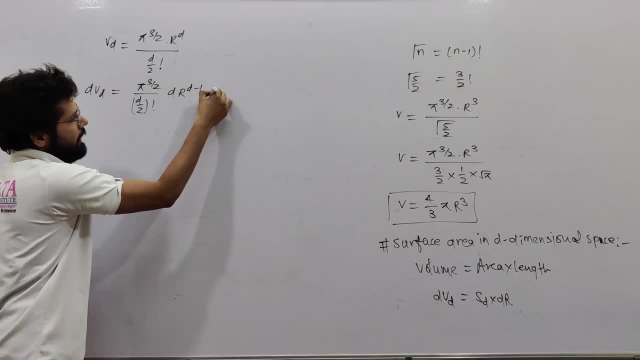 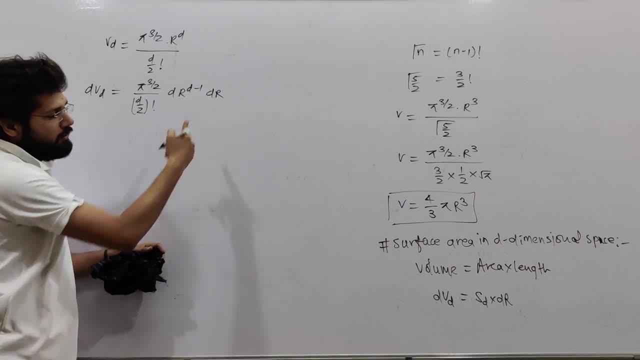 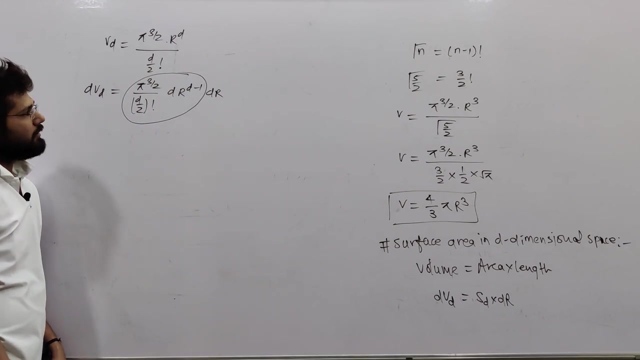 d, R's power d minus 1, dr. now compare it with this: so dvd and dr. what will be the remaining part? sd surface area in d dimensional. so sd is equal to your Pi's power, 3 by 2, and dr's power d minus 1, divided by d by 2. factorial. 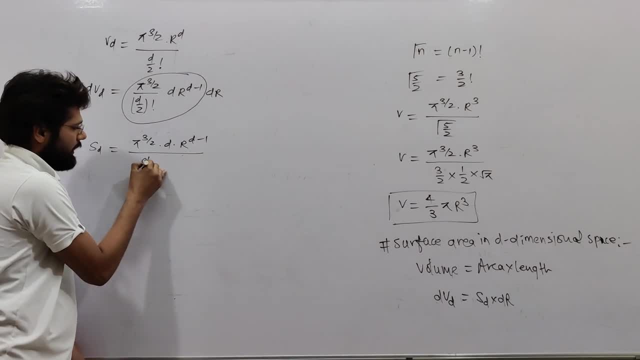 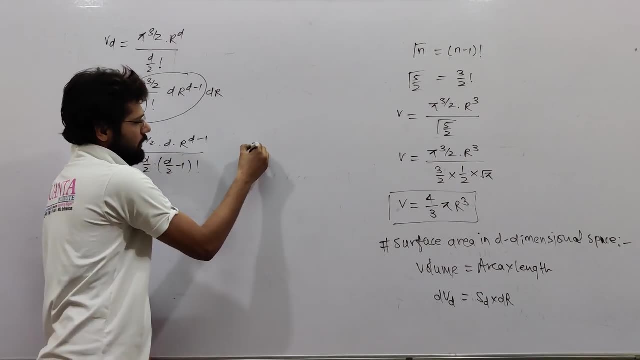 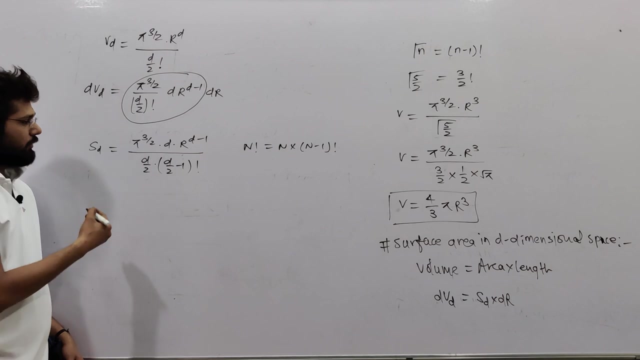 okay, d by 2 factorial. I can write one thing: that: d by 2 into d by 2 minus 1 factorial. can you write it like this: you write n like this: n factorial. n into n minus 1 factorial. you write it like this: you write it like this: you can write it like this. you can write it like this. you can write it like this: 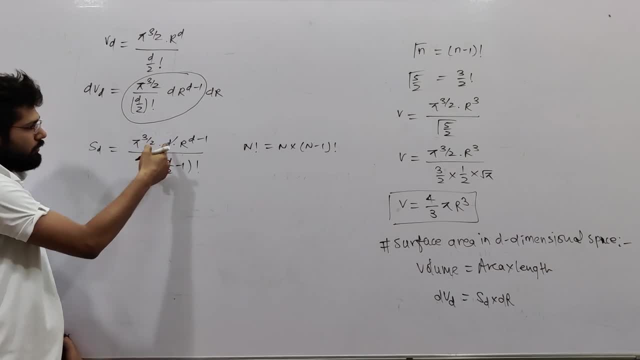 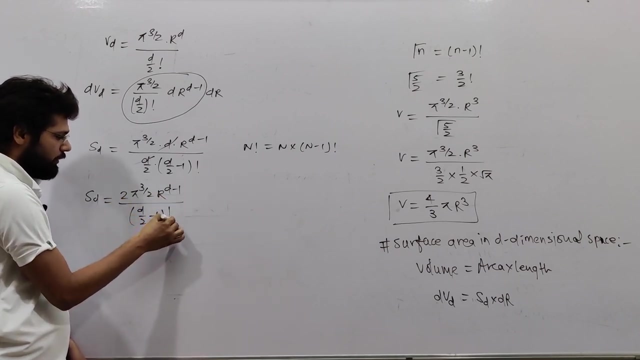 it is written like this because you want to cut d into it. I was not able to do it, so you cut d into d. so what will be sd Pi's power: 3 by 2, and let's bring 2 up, so 2, and R's power, d minus 1, and d by 2 minus 1 factorial. so this one is formula for surface area in d dimensional. okay. 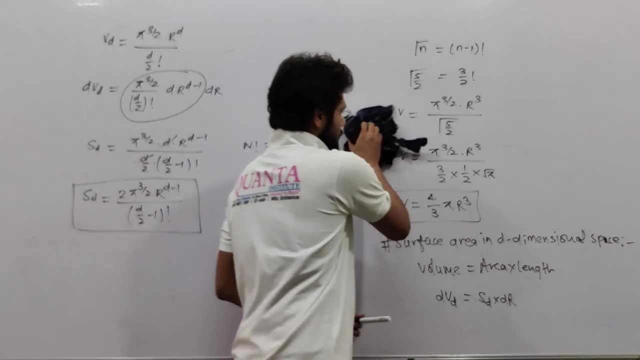 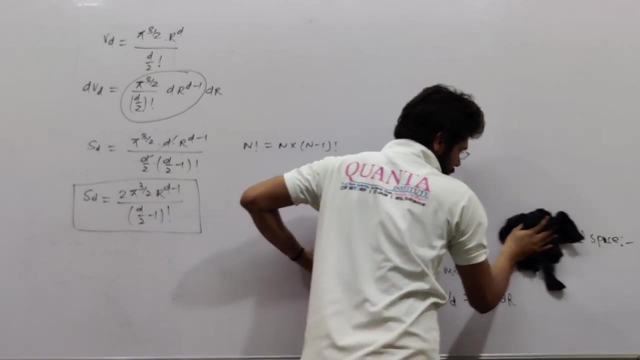 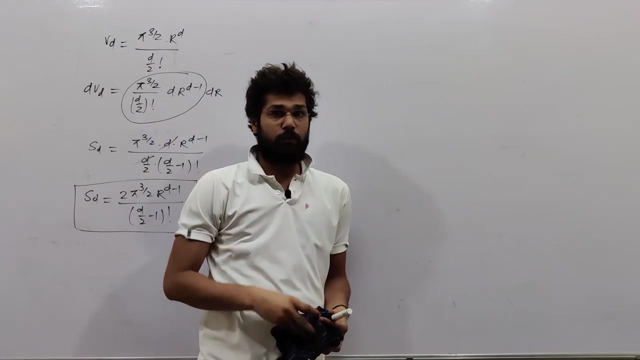 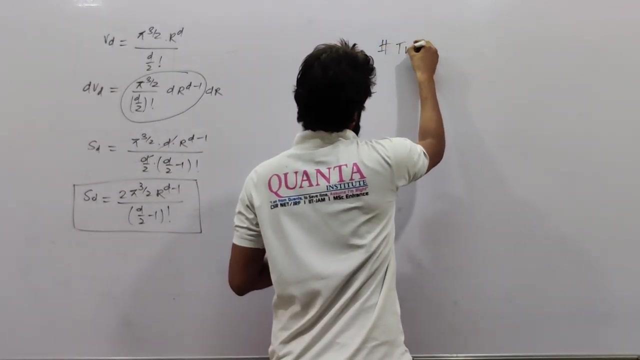 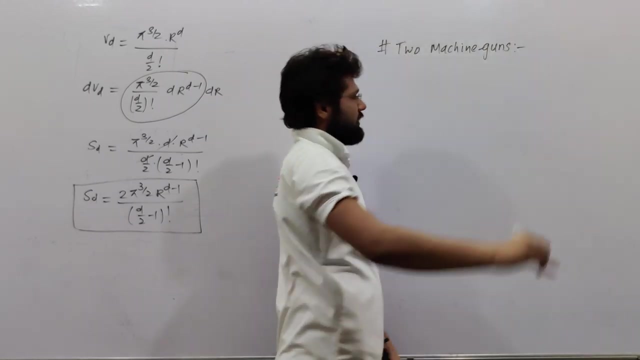 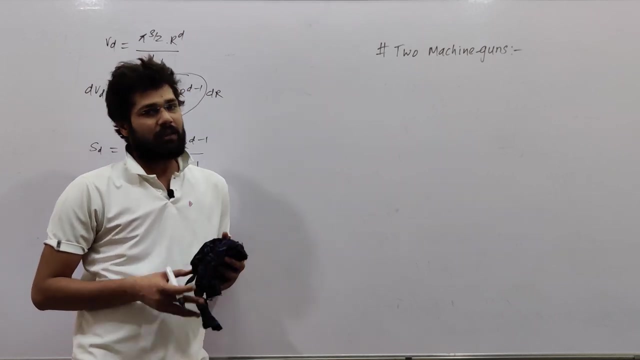 let's move on to the next topic. next is your topic: two machine guns. what two machine guns? two machine guns? this topic doesn't seem obvious to you. you aren't into physics? ohno, I made it. why I made it? have a look. 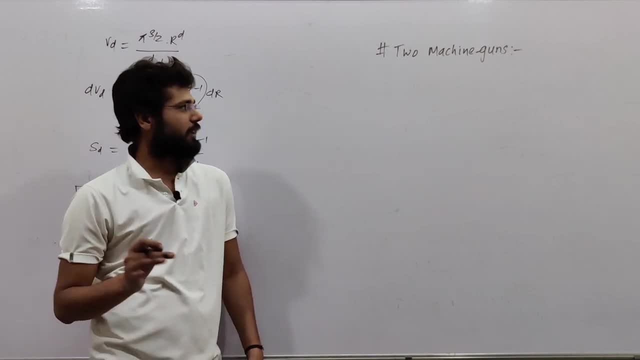 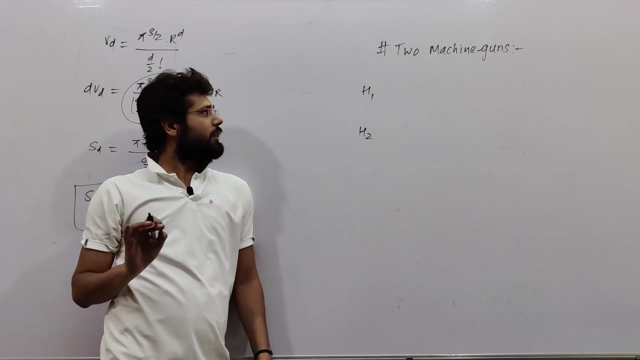 looks like these objects. so look at these two objects here. these two things are such that you can control the whole state. you can say that someone else is providing them to you. you will be in control of a human being because of physical대 y 안에. 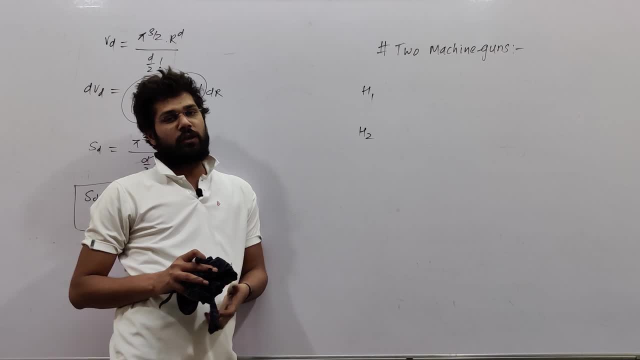 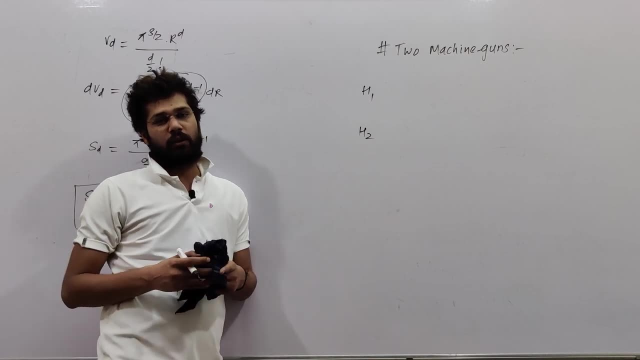 Academy of JW's. 자주 가 데려�نا means anywhere in your community. there you will have someone else to call upon. You don't need to write the formula. you just need to know H1 and H2 and you will be able to solve it easily. 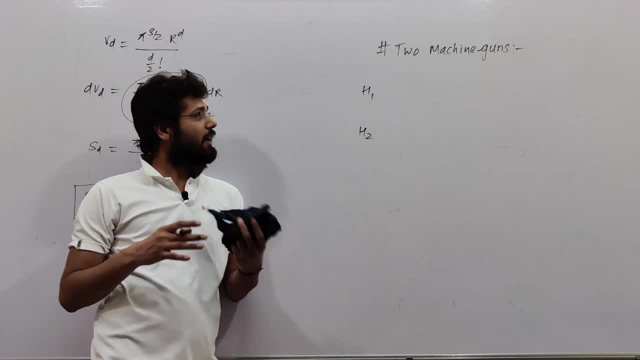 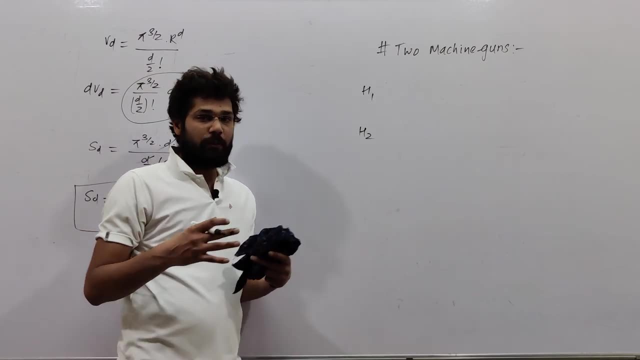 So this is why I am calling this as Machinery. Now, what are R1 and R2?? You will notice that This is a very powerful thing. You will get to know the power later, as we move forward. What is H1?? 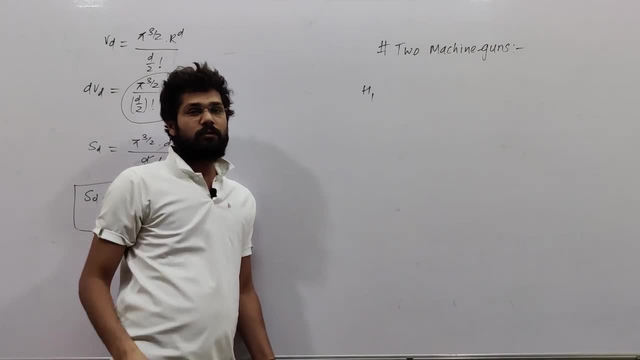 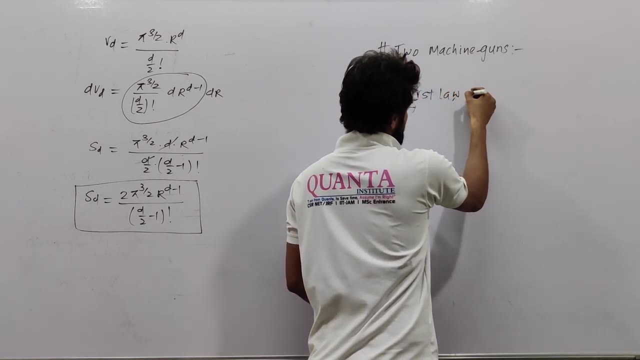 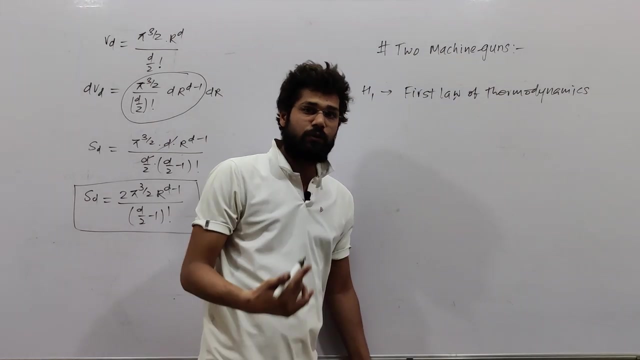 H1 is simply your first law of thermodynamics. H1 is simply first law of thermodynamics. I will write both H1 and H2 and then I will tell you where they will be used. First law of thermodynamics. everyone remembers it. 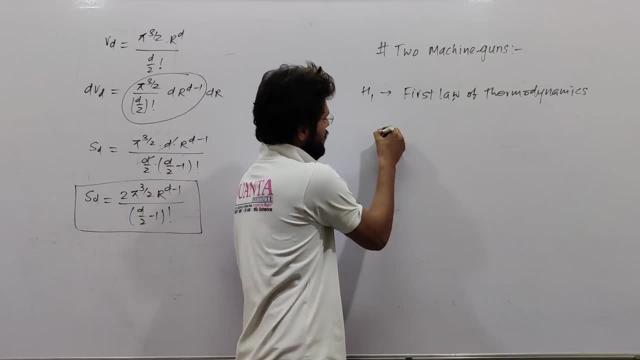 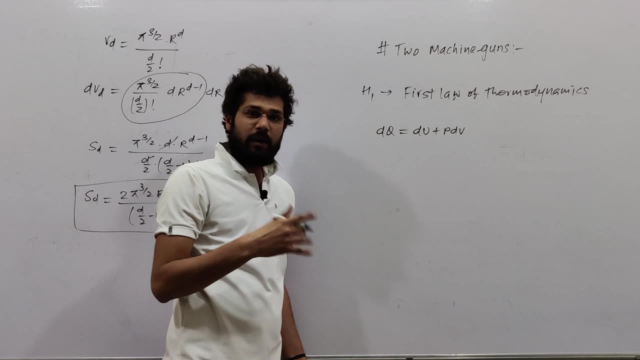 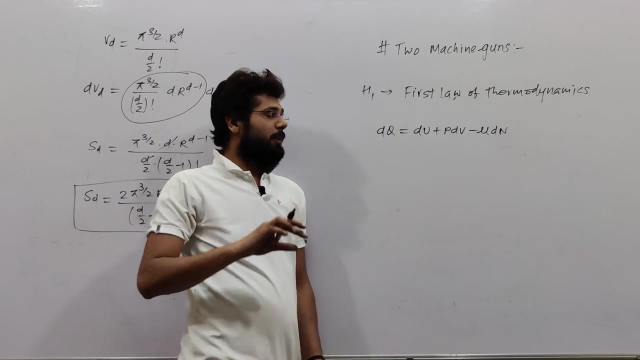 You already had H1.. What is the first law of thermodynamics? dQ is equal to du plus pdv. This is what you have read. There is one more term in this: minus mu dn. This is when the number of particles are also changing in the system. 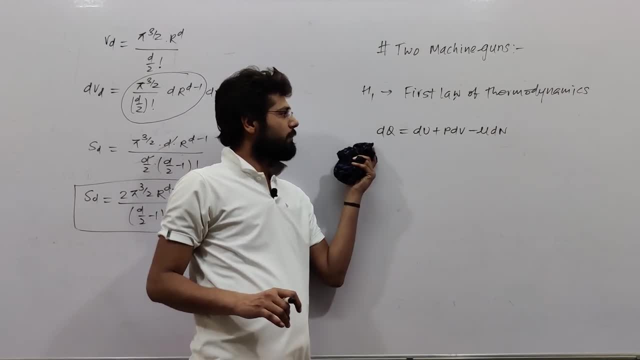 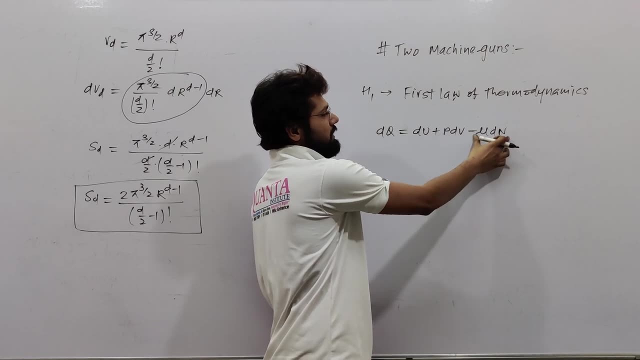 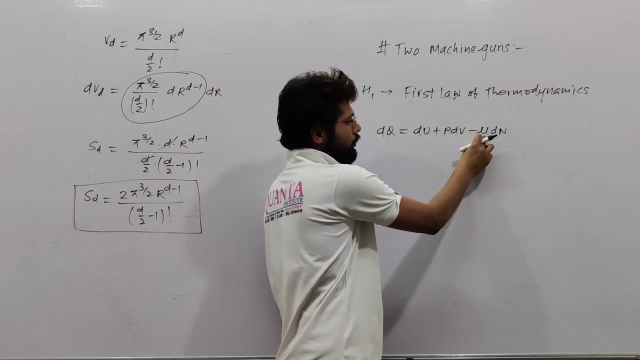 This is a general first law of thermodynamics. You have read this much till now, but if the number of particles changes in the system, then this term is also added. You are already familiar with this. I will tell you. mu. What is mu? 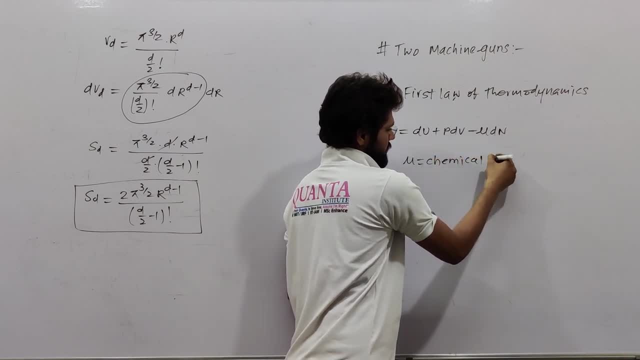 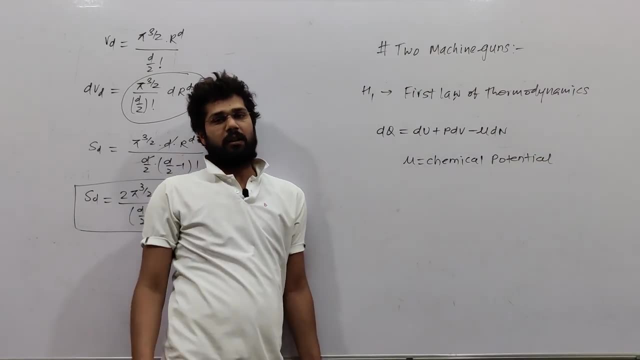 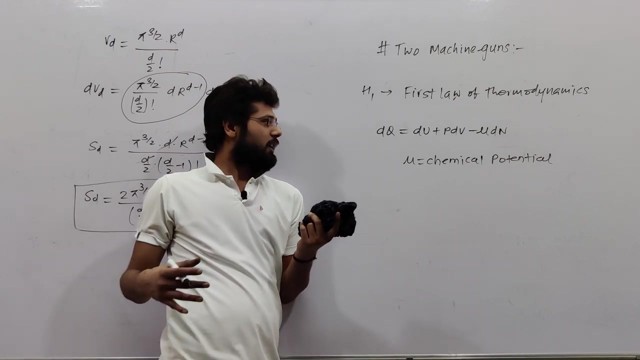 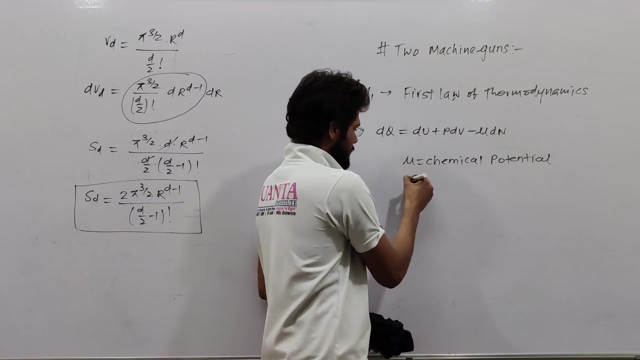 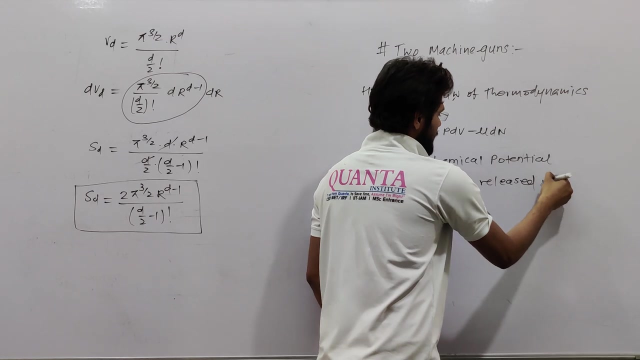 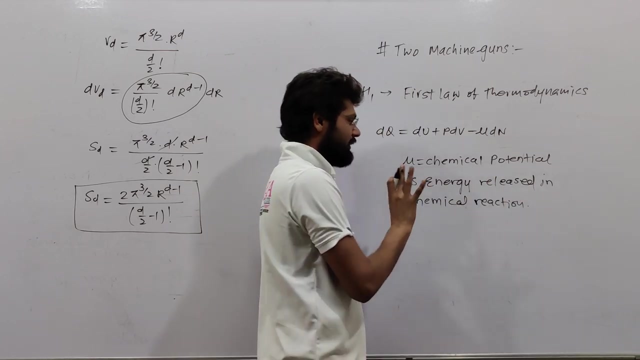 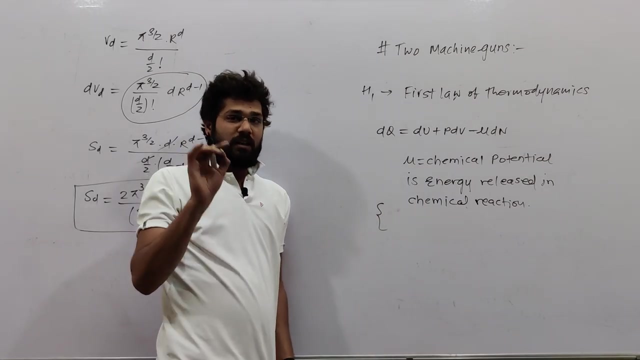 mu, is your chemical potential? What is chemical potential? It is a chemical energy that comes out in the reaction. Chemical potential is an energy released in a reaction. Chemical potential is an energy released in a reaction, In a chemical reaction. Actually, when we talk about chemical potential, whenever the number of particles are changing in the system, then we will talk about chemical potential. 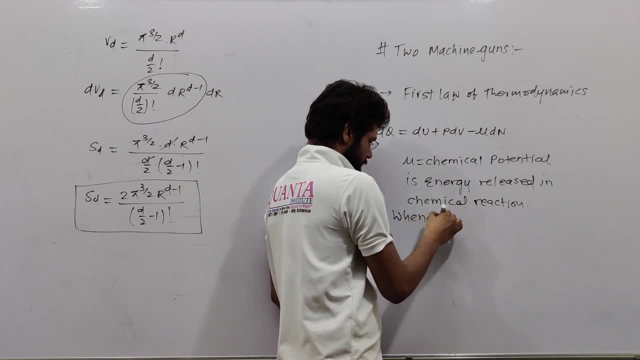 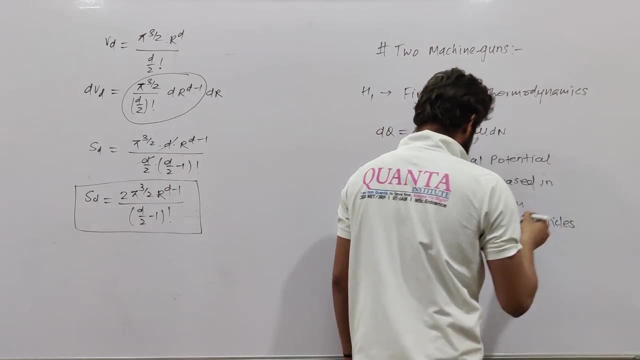 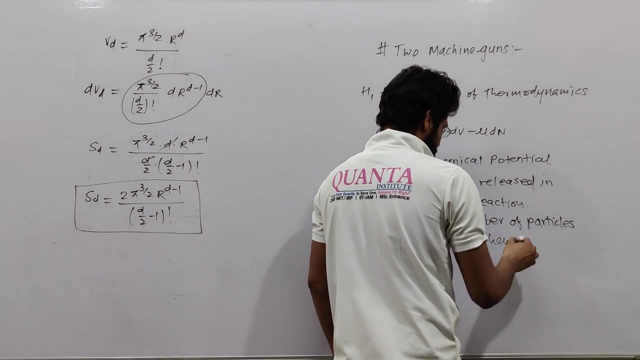 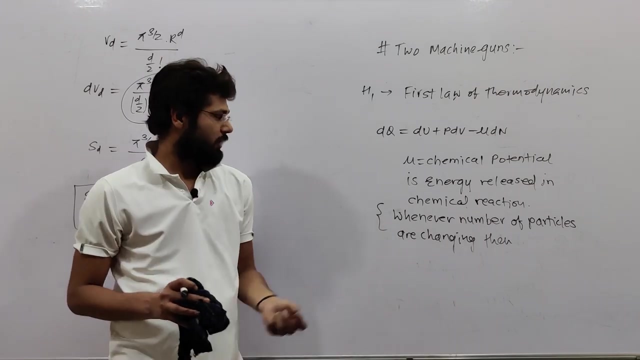 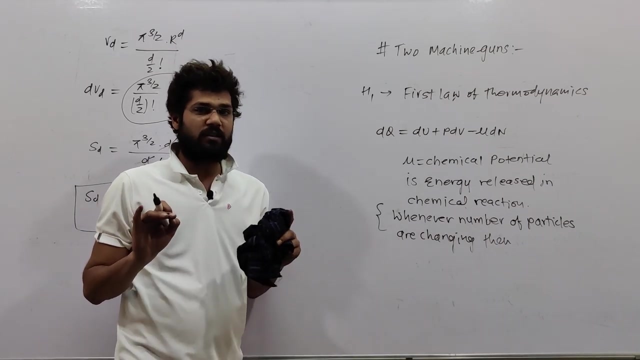 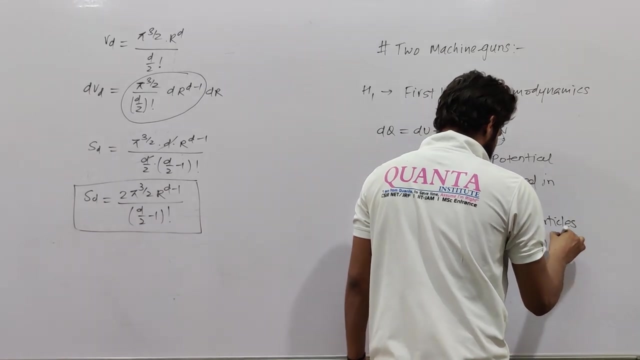 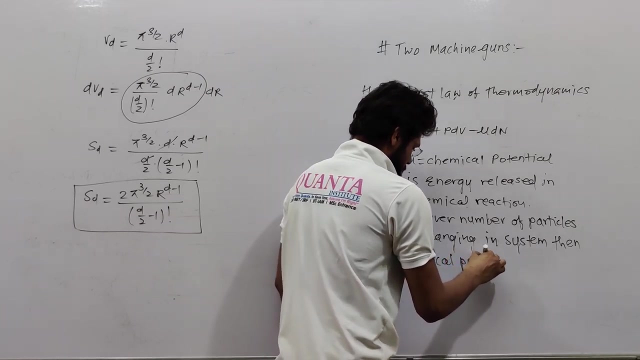 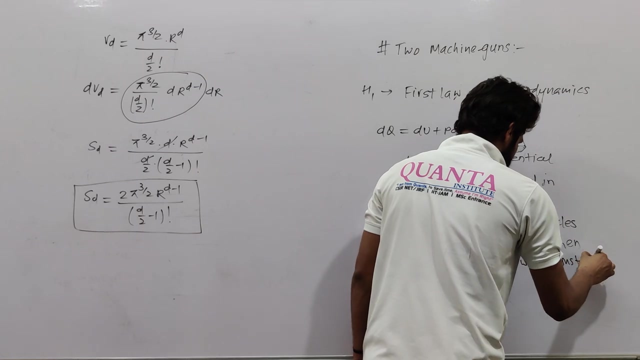 Whenever the number of particles are changing in the system, then we will talk about chemical potential. Whenever the number of particles are changing in the system, then chemical potential will be constant. changing in system, then chemical potential will be constant, will be constant for system, the system. a chemical potential come constant right. 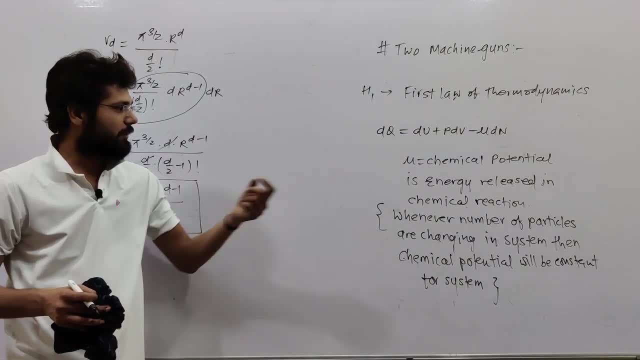 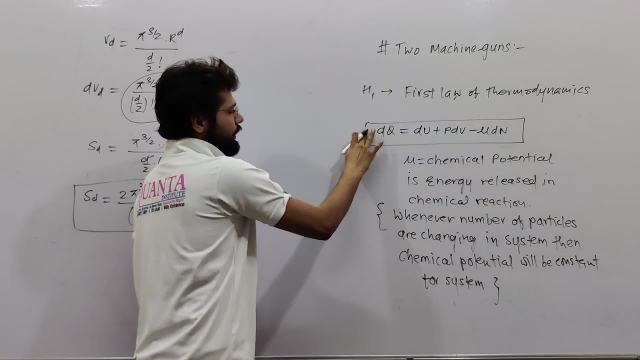 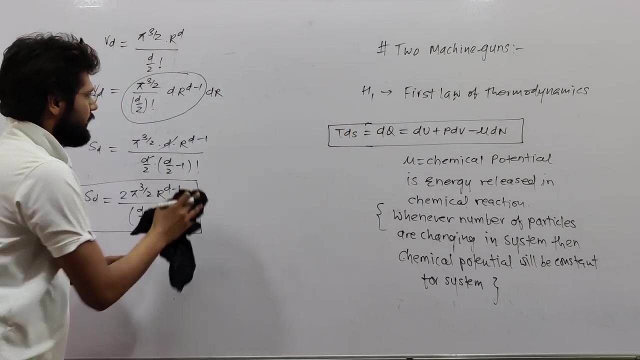 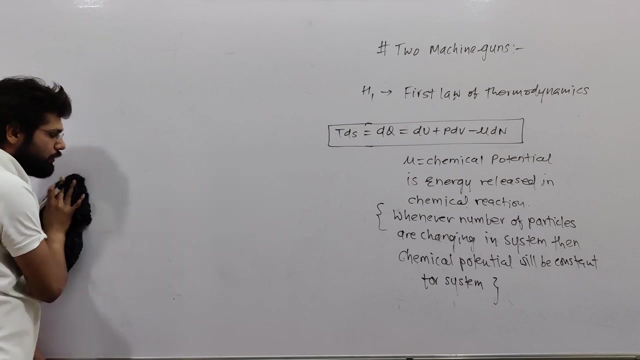 now you know, the number of particles will be changing. this is your weapon 1. now i will add one more thing. what do you write in dq tds? now this is your whole weapon. now we will talk about h2 weapon 2. now we will talk about where this weapon will be used. 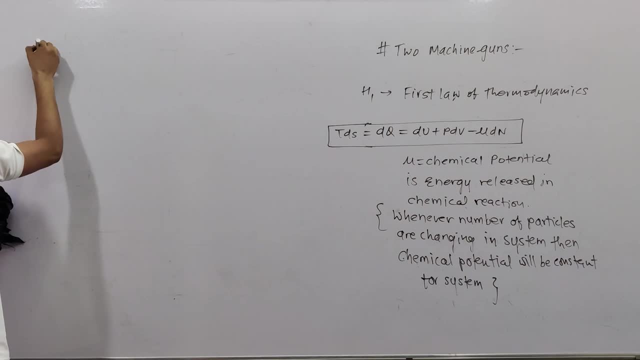 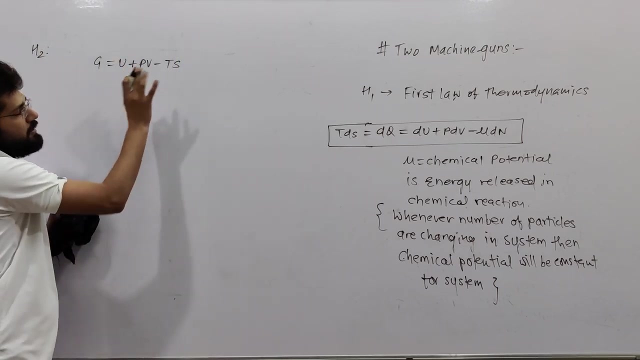 now we will talk about where this weapon will be used. lets see, lets see h2. h2 is this relation that gives free energy. g will be equal to u plus u plus pv minus u plus pv minus ts, u plus pv minus ts, and also equal to mu n. 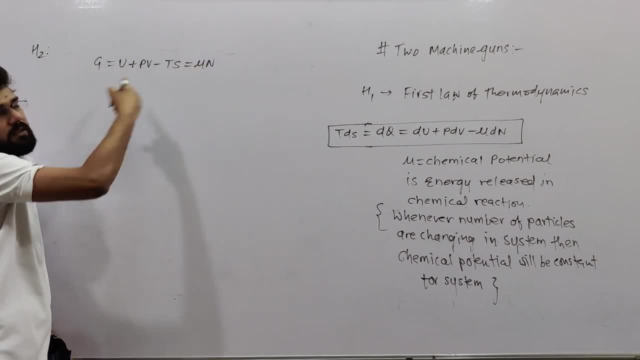 and also equal to mu. n gives free energy. can be written in two types: gives free energy. can be written in two types: mu is chemical potential, n number of particles, t is temperature, s is entropy, p is pressure, v is volume and u is internal energy, g is gives free energy. 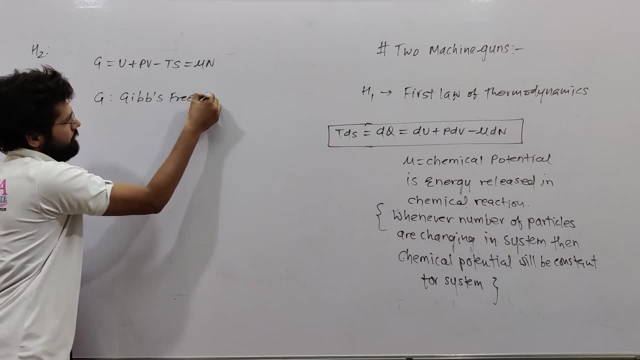 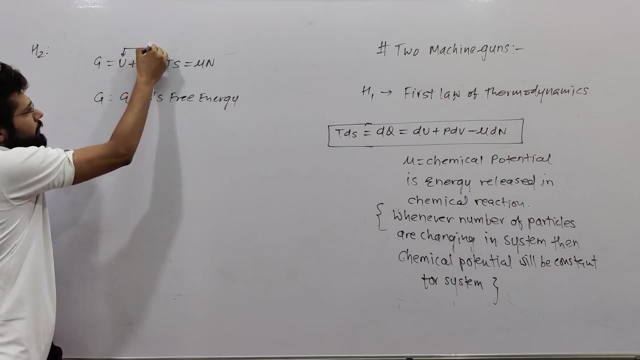 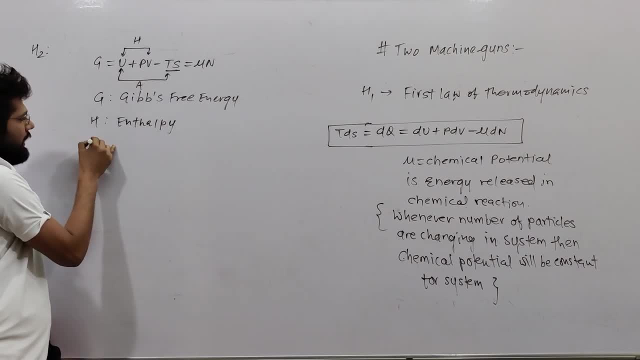 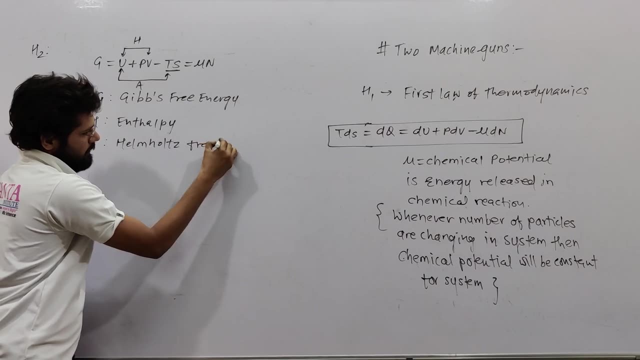 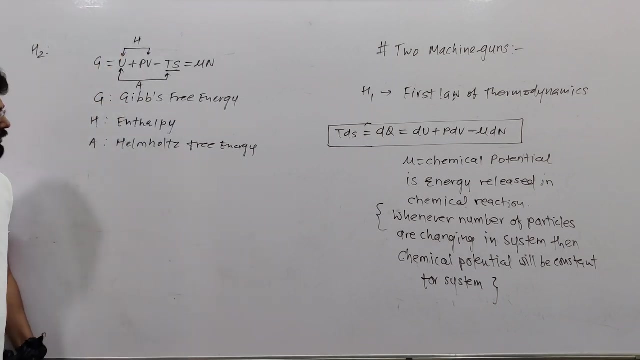 they make a and a is: helm holds free energy. helm holds free energy- free energy, free energy, ok, and this is h2. how to write h: enthalpy: u plus pv. and how to write: helm holds free energy: u plus pv. and how to write: helm holds free energy. 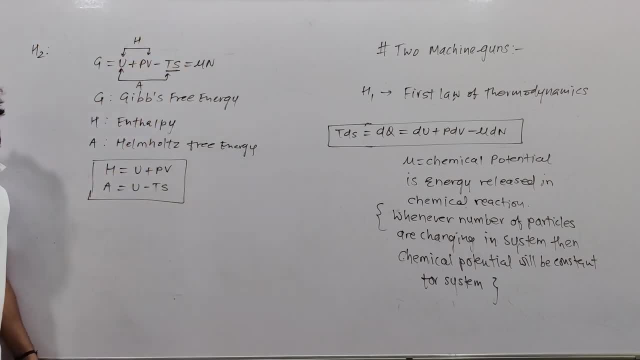 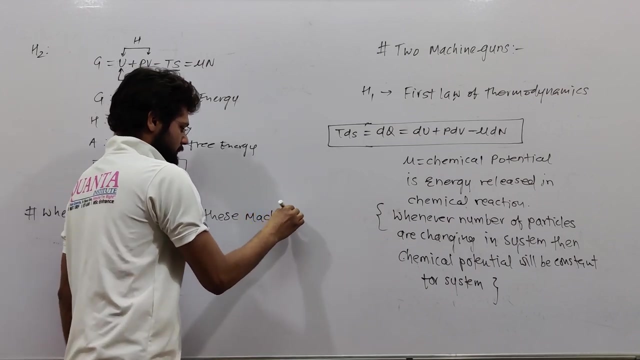 u minus ts. simply write u plus pv, and g is written mu n. this is h2. where is h2 used? see where we have to use, where we have to use these machine guns. where we have to use these machine guns, use these machine guns, use these machine guns. 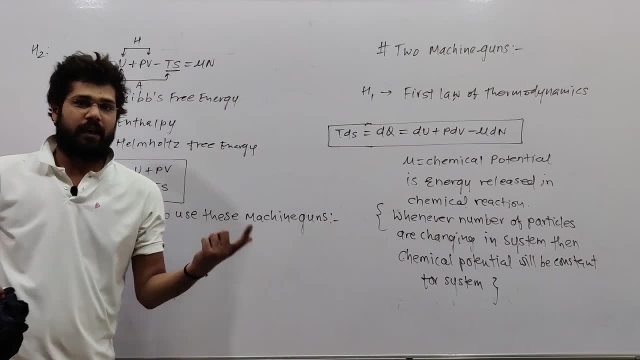 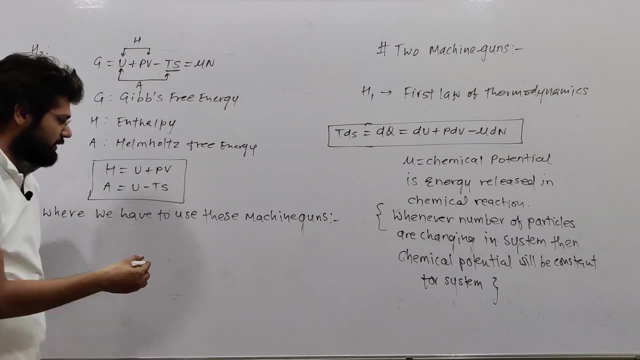 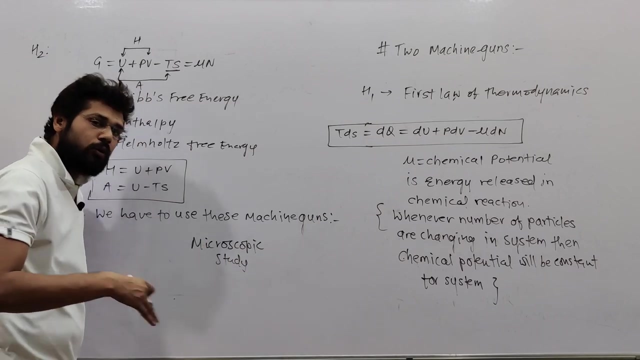 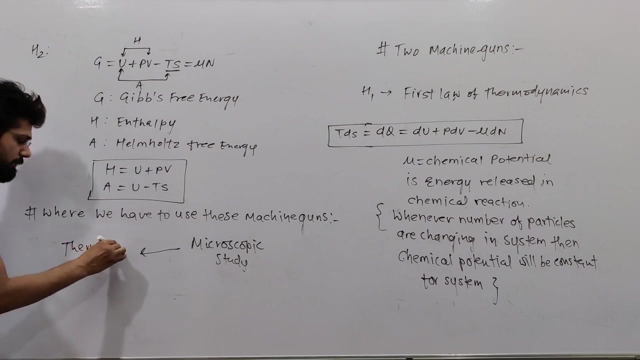 see what is in your stat. first of all, mechanics. What do you do with STATMAX? You do microscopic study of the system with STATMAX. What do you obtain from that study? You obtain thermodynamic variables from microscopic study. You obtain thermodynamic variables from STATMAX. 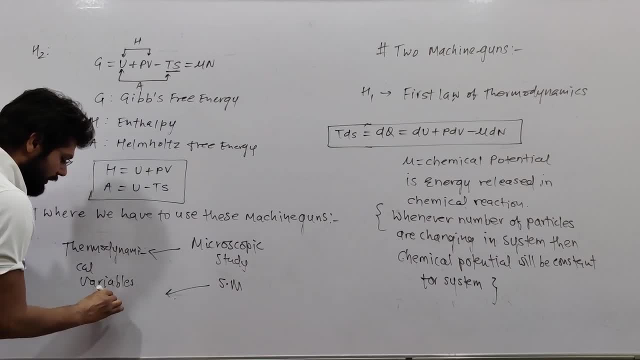 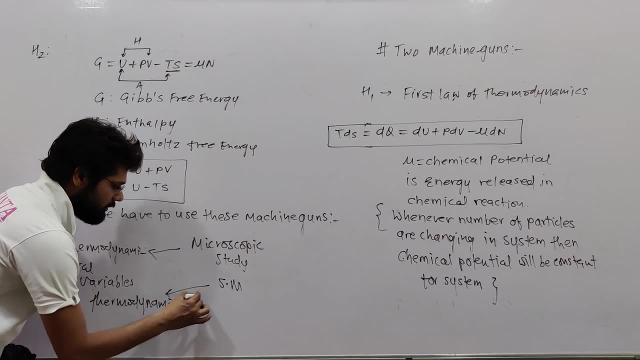 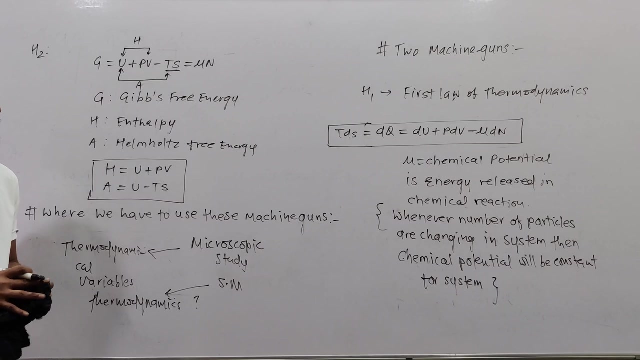 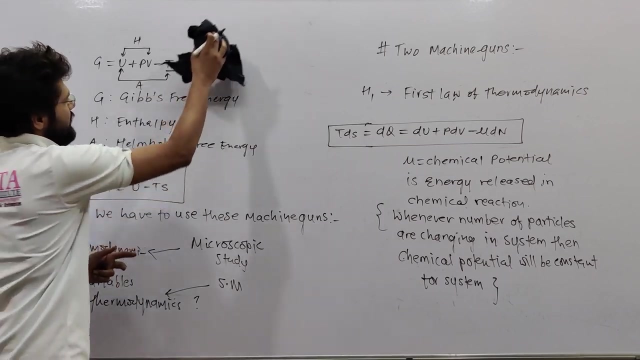 What does STATMAX give you? It gives you thermodynamics. Now the question arises: how do you obtain thermodynamic variables from STATMAX? It will take some time to explain. There are three ensembles of thermodynamic variables. I will create some space here. 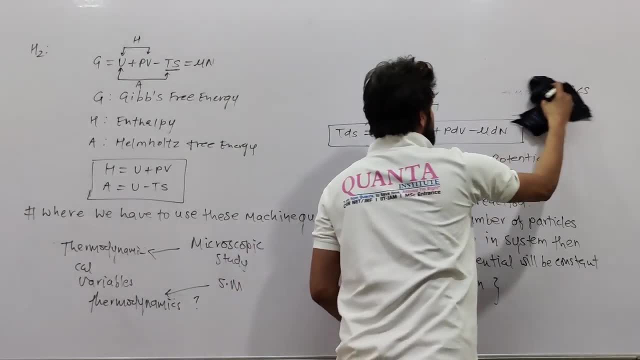 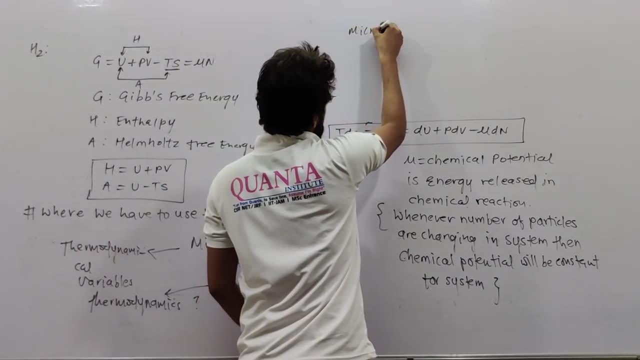 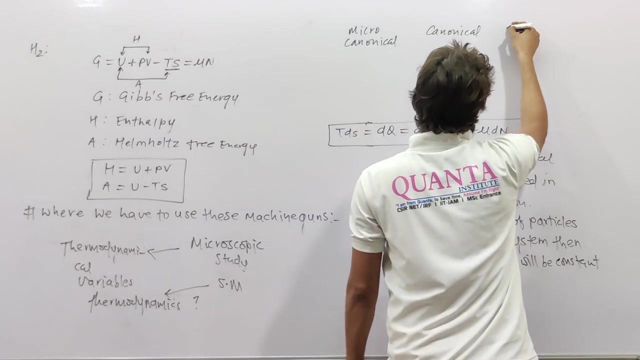 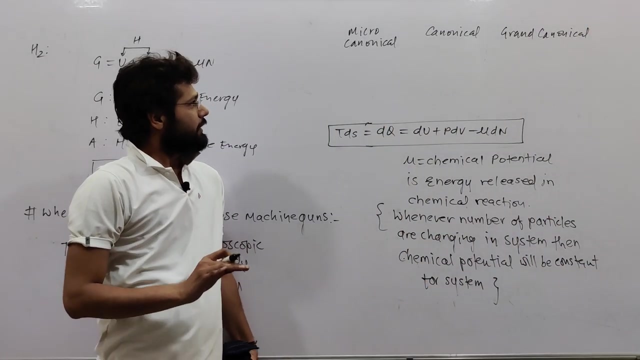 Let's remove this. There will be three ensembles of thermodynamic variables. One will be MICRO-CANONICAL, One will be CANONICAL, One will be GRAND-CANONICAL. These three ensembles will be discussed. One thermodynamic variable plays a leading role in these three ensembles. 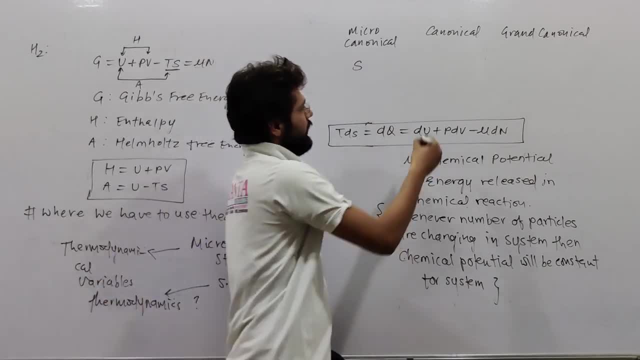 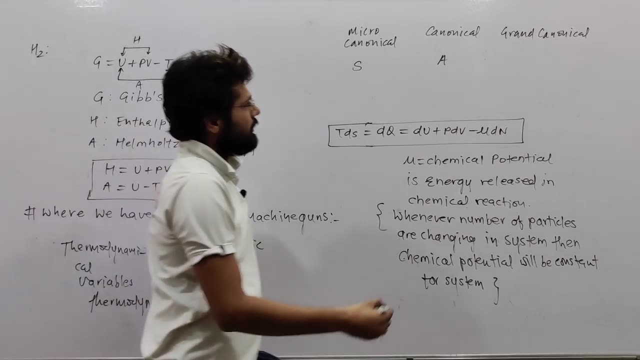 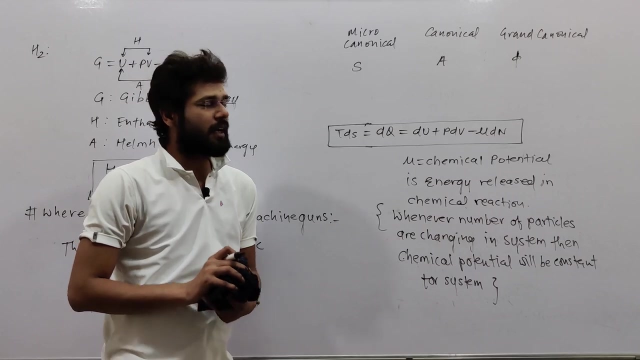 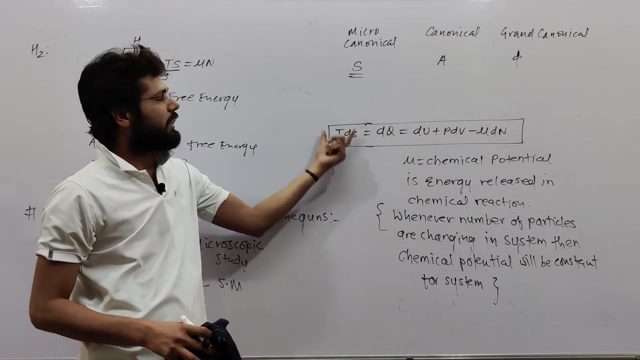 Here entropy plays a leading role. Here Helmholtz, free energy plays a leading role Here. GIBBS potential is defined as PHI. What does leading mean? If you have entropy, then other thermodynamic variables like Cb, Cp, Gamma, Pressure, Temperature, Mu, etc. 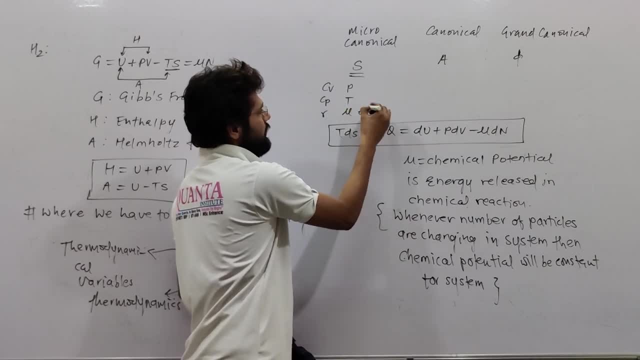 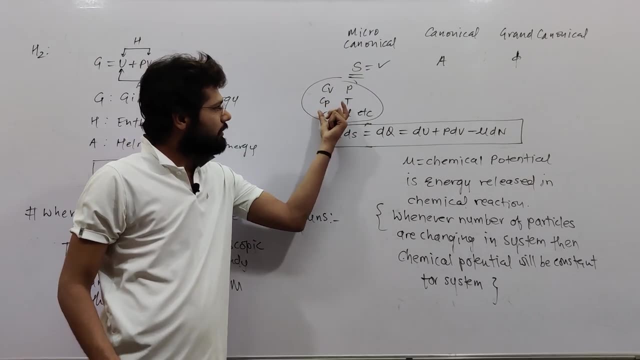 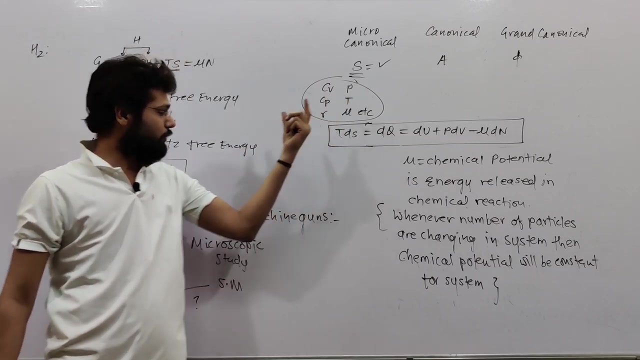 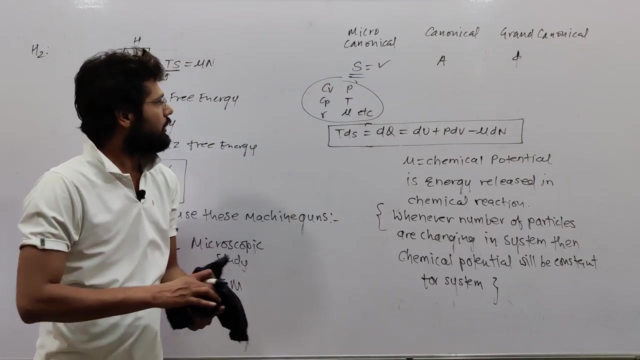 You can obtain all these if you know S. How do you obtain these From H1 and H2.. This is the thing. You can obtain thermodynamic variables from STATMAX. This is what you get from STATMAX. What is S equal to? 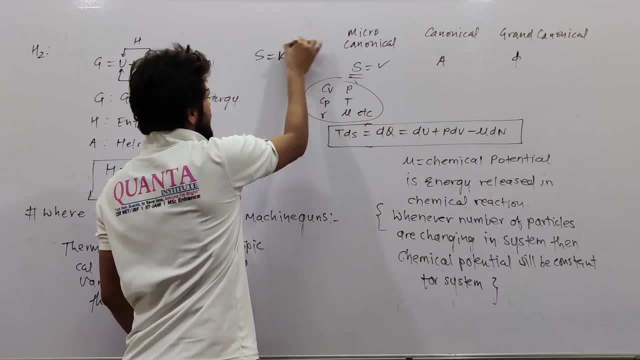 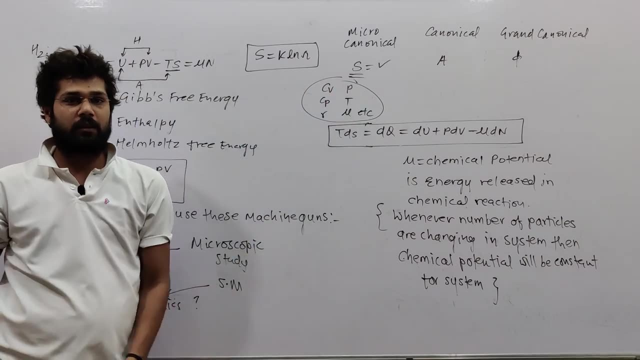 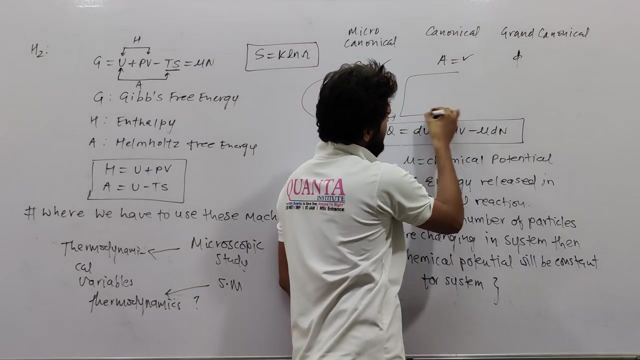 Let me talk about MICRO. If you know S from here, you can find out everything. We will do this in the near future. Similarly, if you know Helmholtz free energy in CANONICAL ENSEMBLE, then you can obtain all other thermodynamic variables. 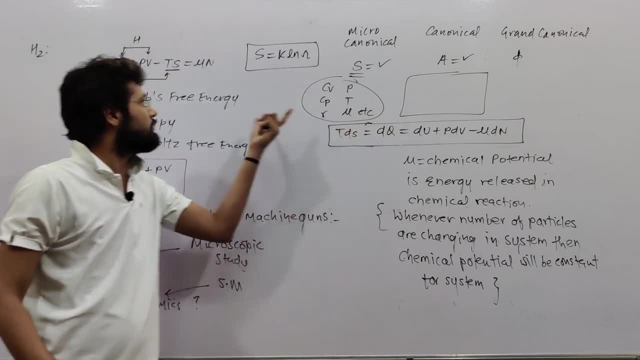 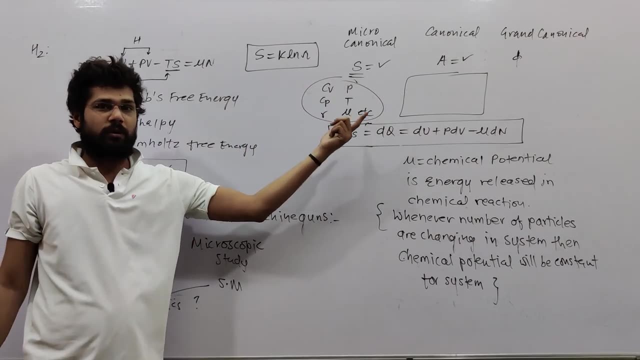 You just have to use these two, This one and this one, And that's why I am calling MACHINE GUNS. Once you know A, then you have the control in your hands. You just have to use MACHINE GUNS and you will get anything. 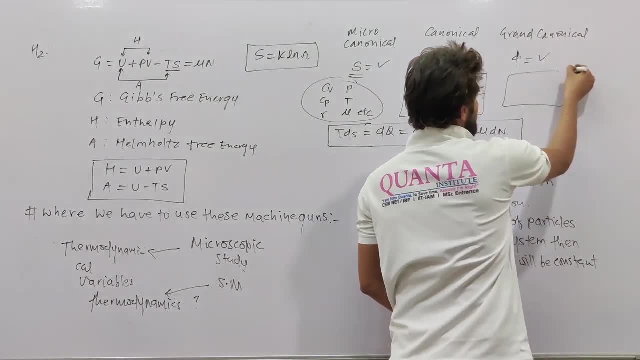 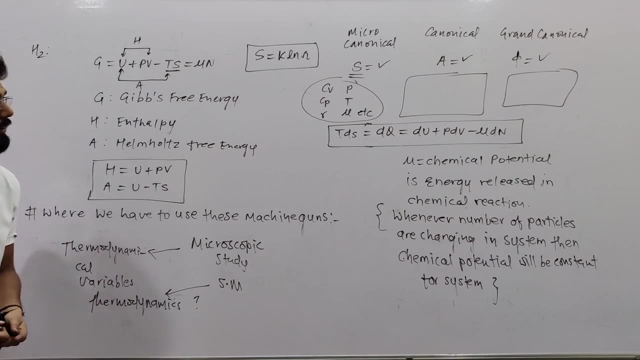 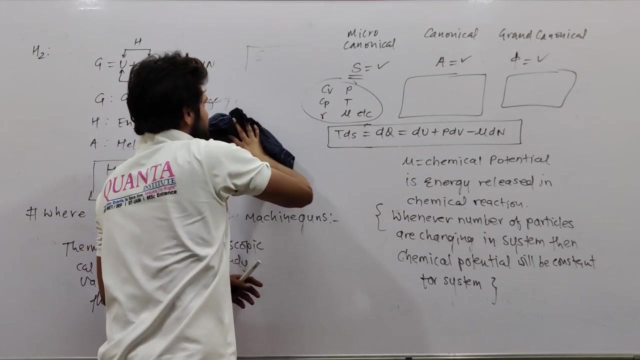 Similarly, if you know PHI, then you can obtain any thermodynamic variables. So you can obtain thermodynamics from STATMAX. Is it clear? Let's talk about the next topic. Keep H1 and H2 safe. You should know how to use them. 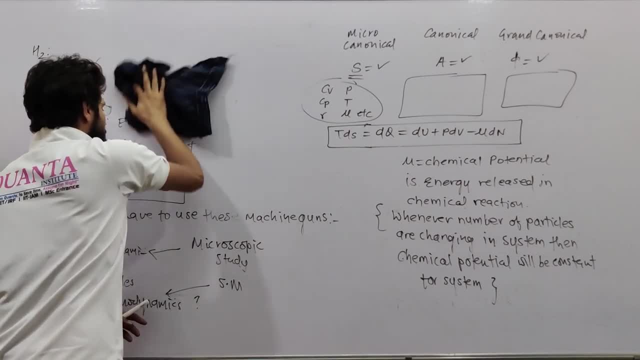 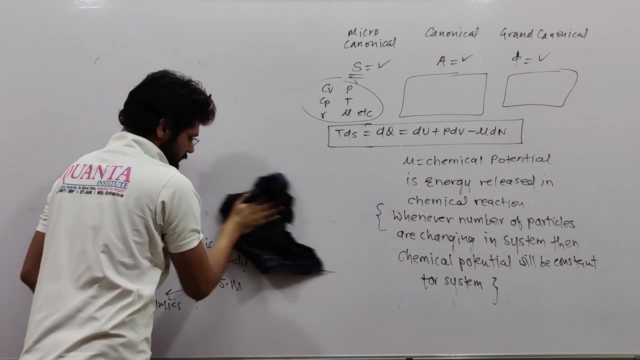 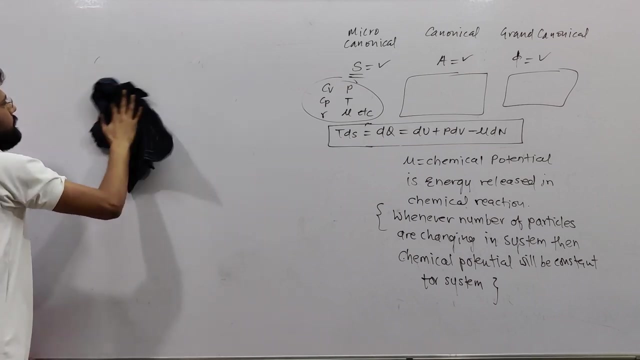 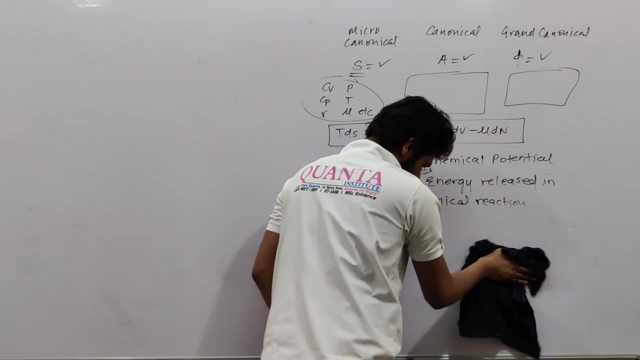 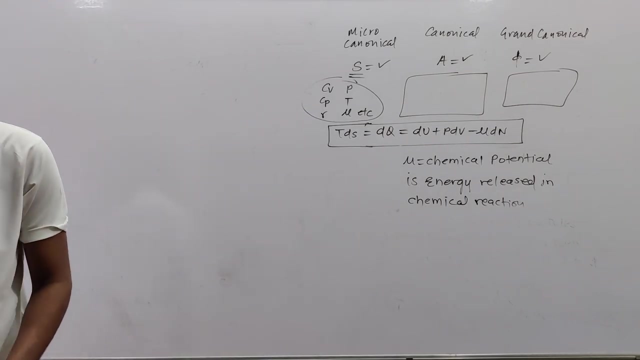 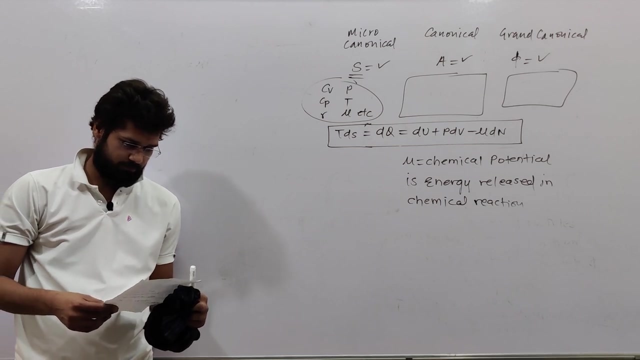 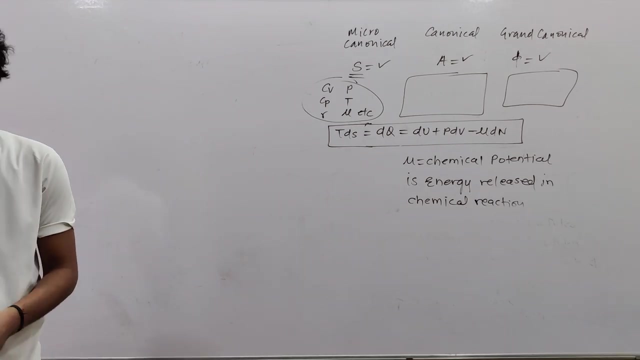 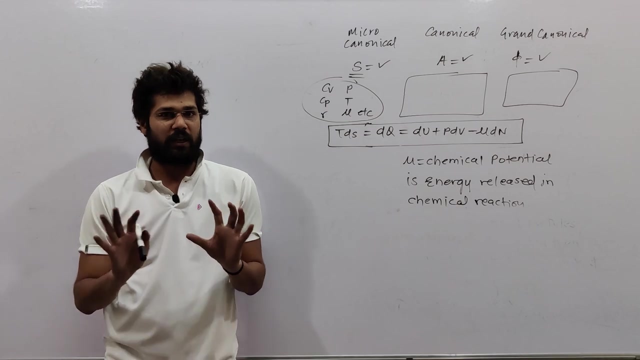 We will teach you how to use them in the near future. Okay, The next topic is…. Let me see it once. Okay, Okay, Okay. So this lecture is over now and now listen. what will happen next means basics of thermodynamics. 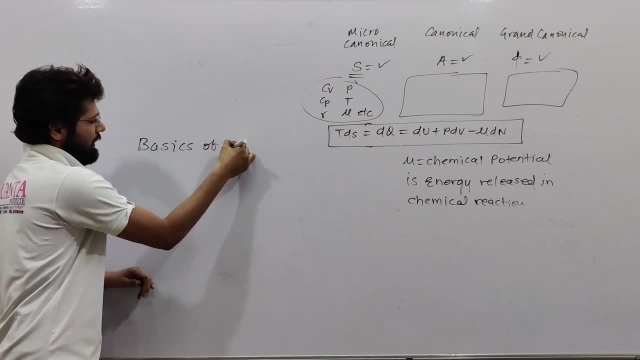 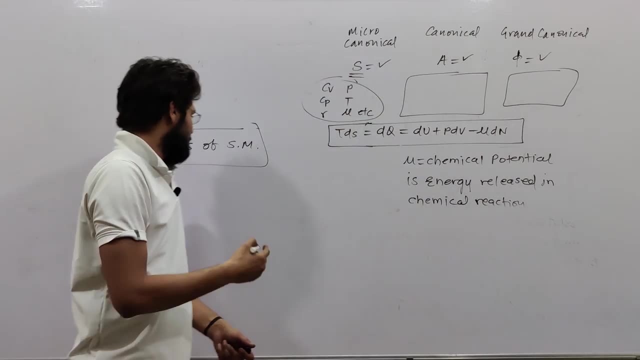 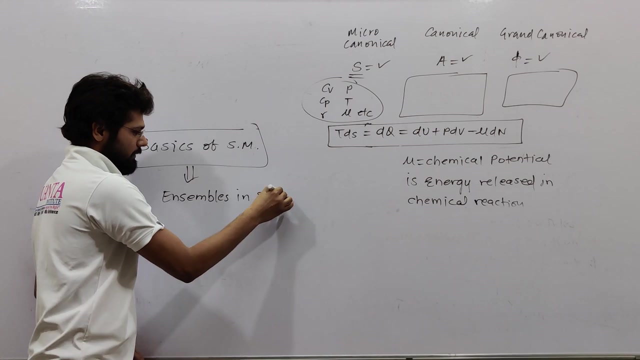 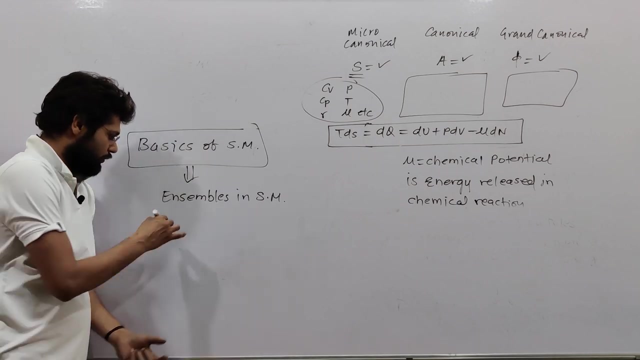 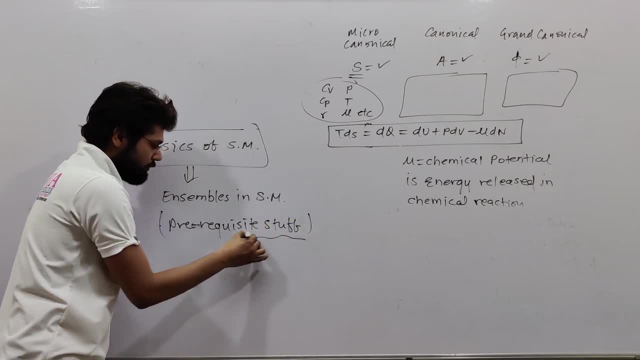 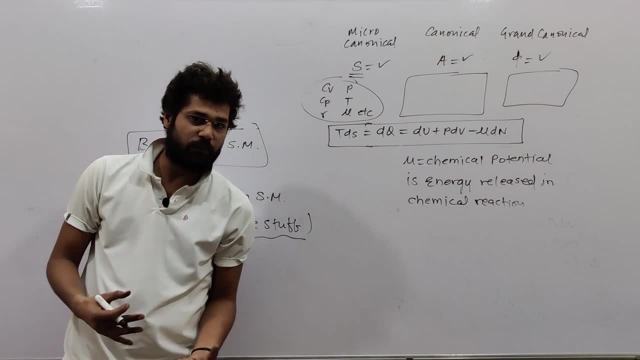